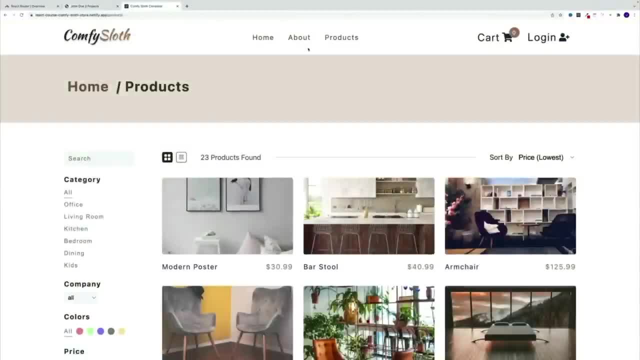 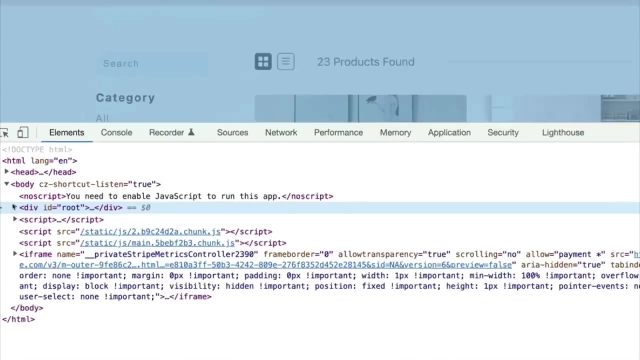 Unlike the react application, where changes happen instantly or get this snappy response, And the reason for that is because we have single page application. So, like I said, we have single page. More specifically, we have single div with an ID of rules. 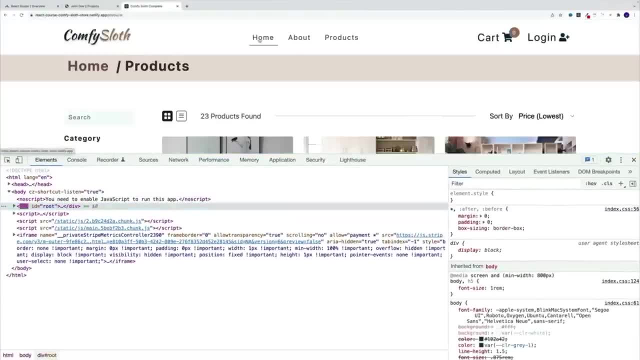 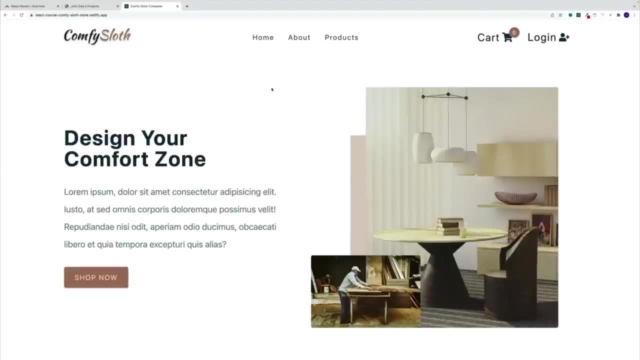 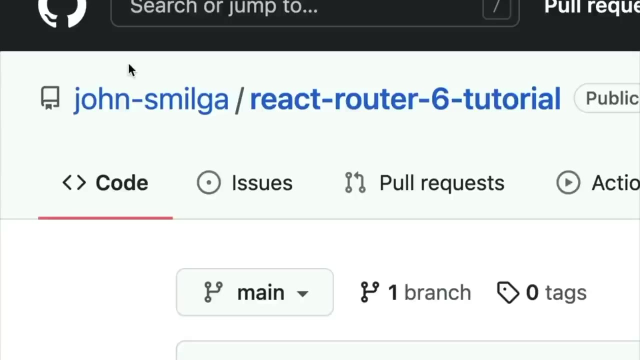 And then all the changes get handled by JavaScript And therefore the contents of the page load instantly without the full page refresh. In order to follow, you need a star, And it's located in this repo. So look for my GitHub and then, more specifically, repo. 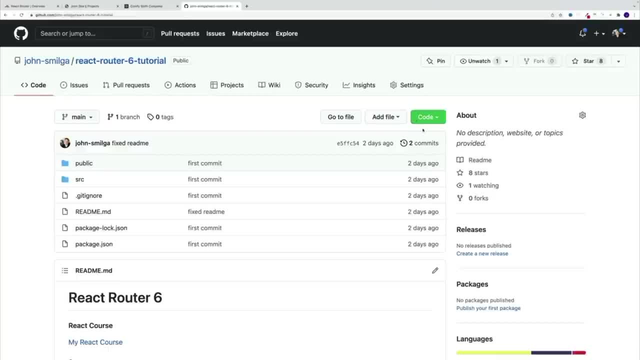 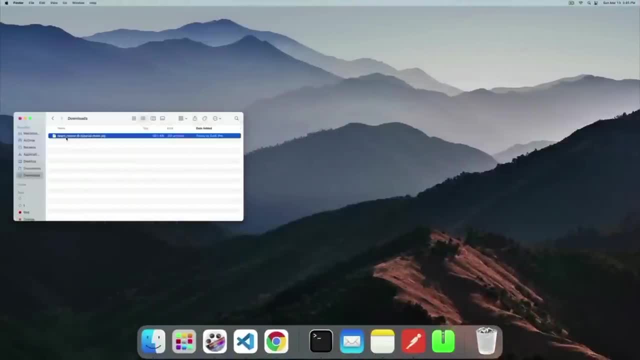 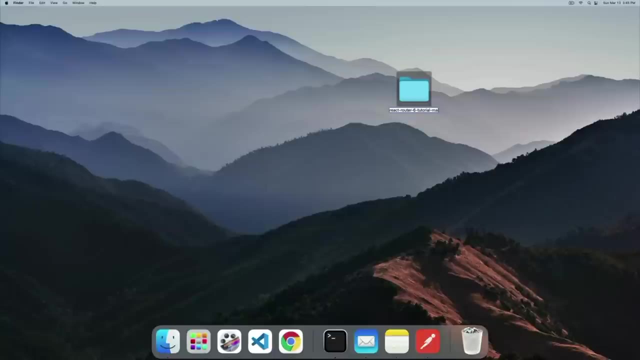 by the name of React router six tutorial. then I'm going to go for download option. How's that that? I'm going to navigate to my downloads, crack it open, drag and drop. So now it's sitting on the desktop. then I think I'll rename it. I'm just going to go with react router After that. 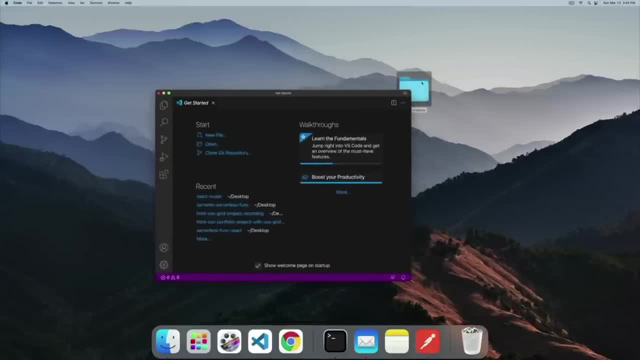 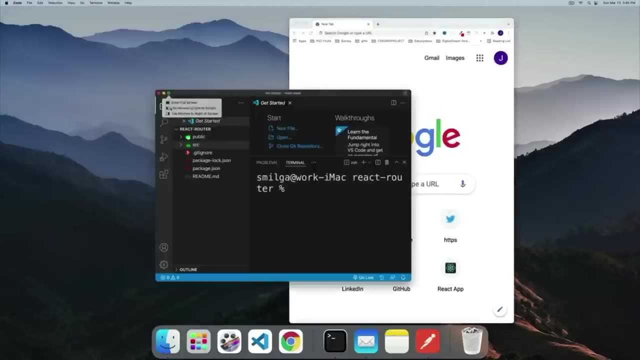 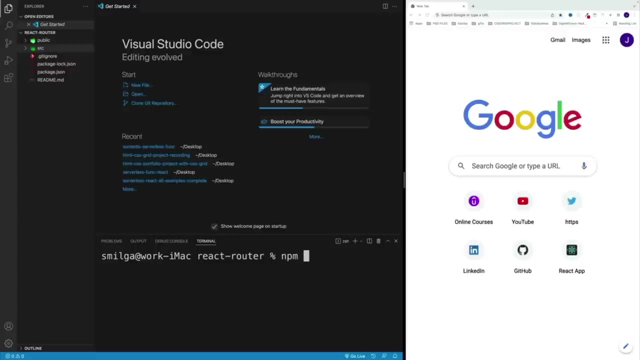 I want to open up Visual Studio code drag and drop, set right away side by side with the browser. And then we want to open up the integrated terminal And we want to go with npm install and right away npm start, And essentially this is a boilerplate react application. 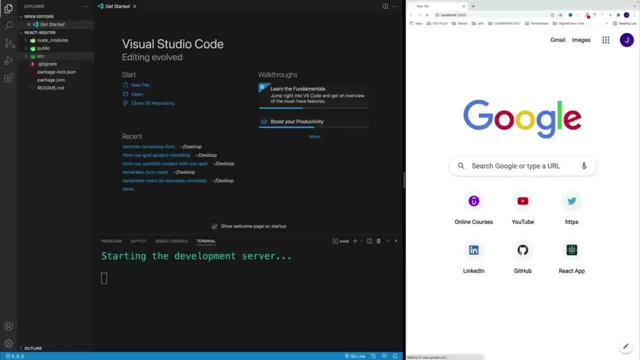 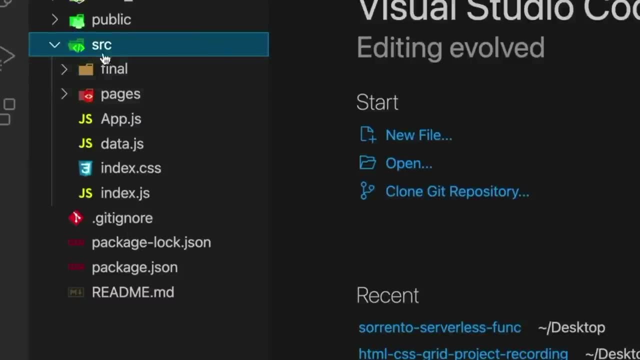 Effectively. I created with create react app And here you'll just find some useful resources So we don't have to type out some boilerplate code. So in the source there's a final folder where you'll find complete application. So if you ever need to, 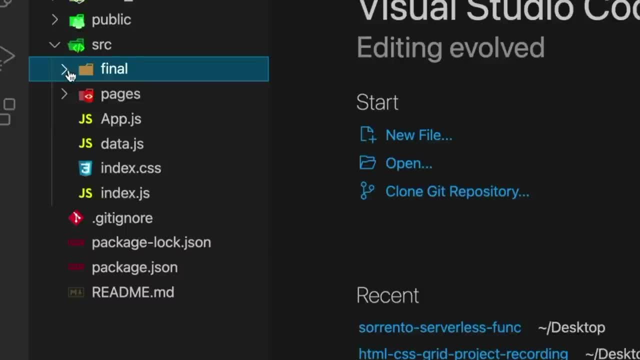 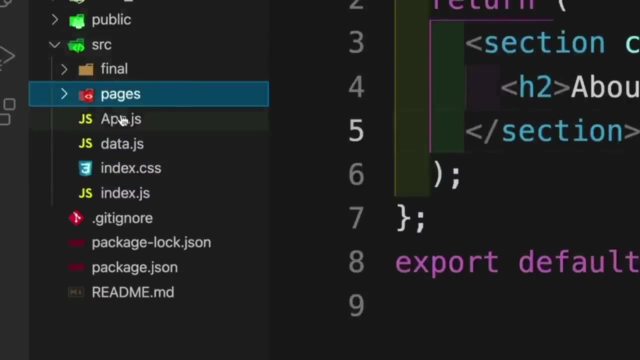 reference the code that I type in the videos. you can find it over there. We also have pages folder. You'll see in the following videos why we have it there effectively is just a bunch of react components, And again we'll talk about them in a few videos. 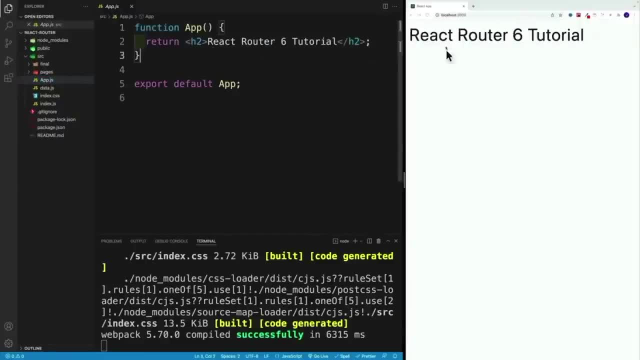 After that we have app js, where we just have a heading to with this text, data js- also something that we'll implement a little bit later in the CSS, with all of the styling. Now, there's not much to it, But still, I added a little bit of styling here And, of course, 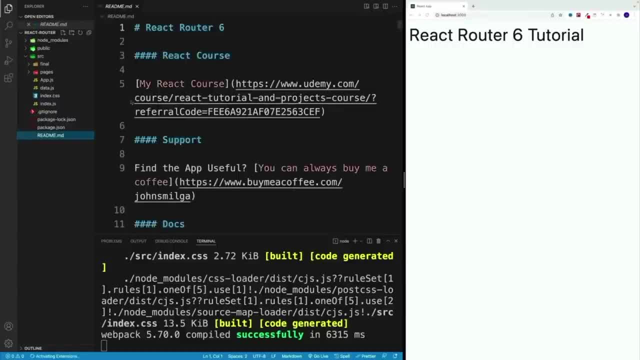 indexjs And also in the route we'll find readme where I wrote down all the steps we're going to take throughout this project. And if you see in the browser react router six tutorial, then we're in good shape And we can start exploring react router six. Okay. 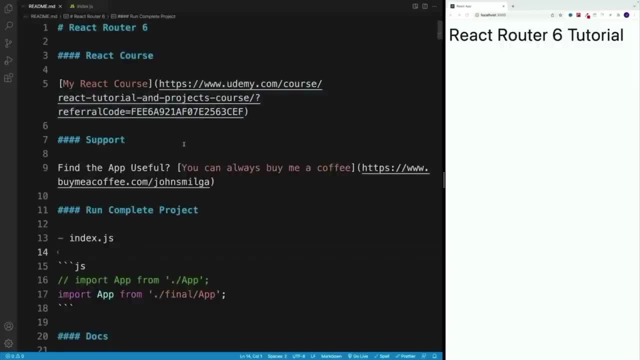 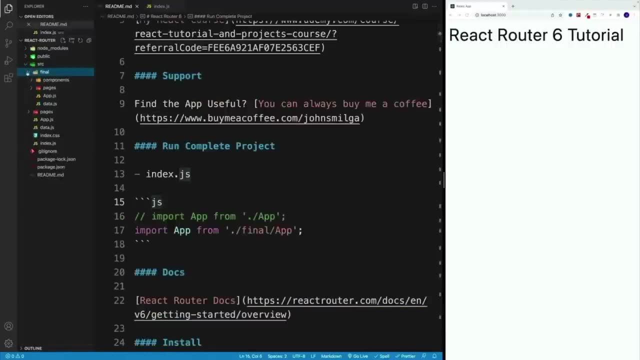 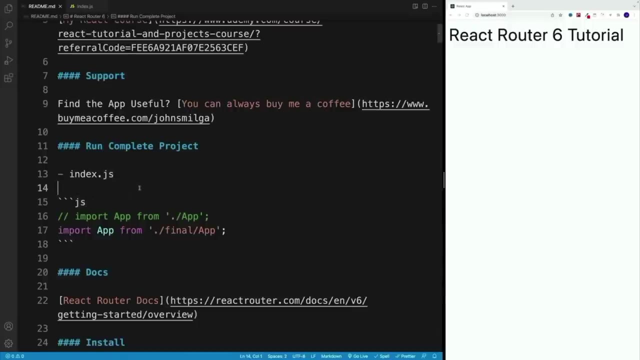 and before we start typing away, let me just mention a few things. First, if you ever want to run the complete application, so not just reference the code in the final one, But if you actually want to see some feature in action, just go to indexjs and swap the app js files. So 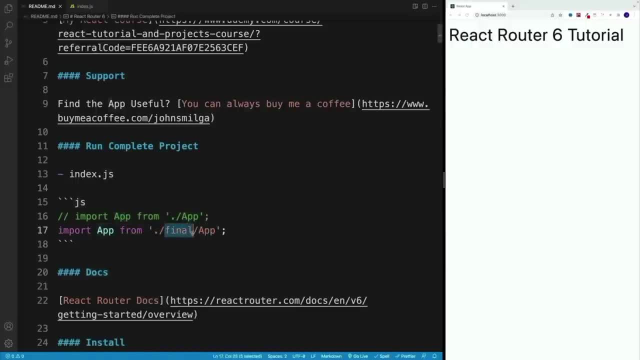 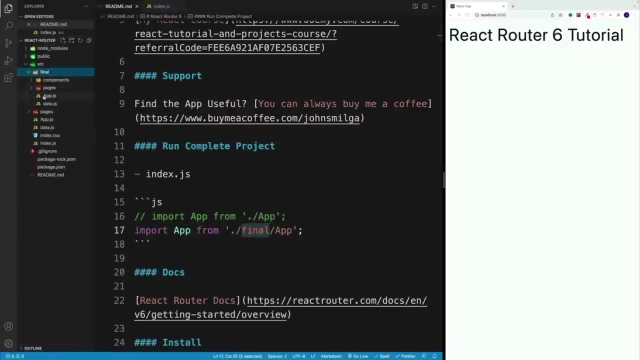 essentially you want to get the app js from the final folder. So, like I said, final folder is where you'll find complete application And in here there's also a app js. So just go to indexjs, get the app js. 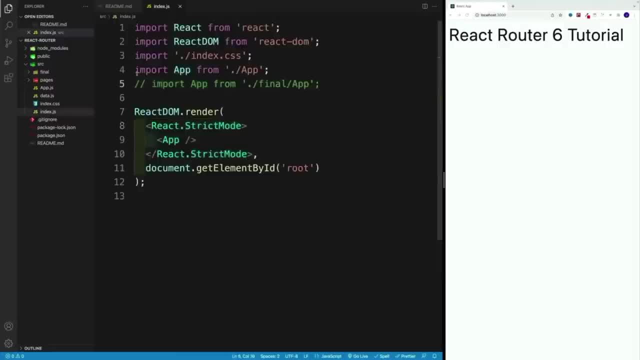 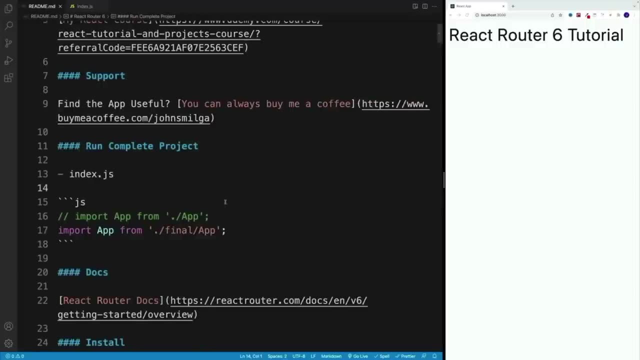 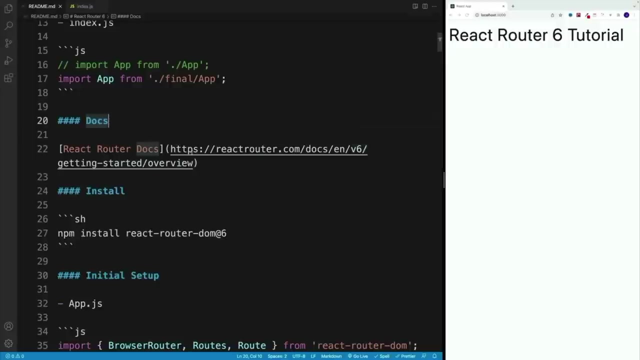 from the final folder, And I already added the code. you just need to comment the first one out and uncomment the last one. Then, if you ever need a reference to official documentation, I left it in the readme, a link. So if you click on this link you'll navigate to the official. 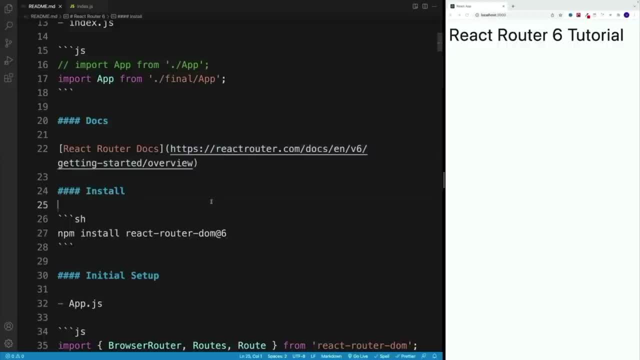 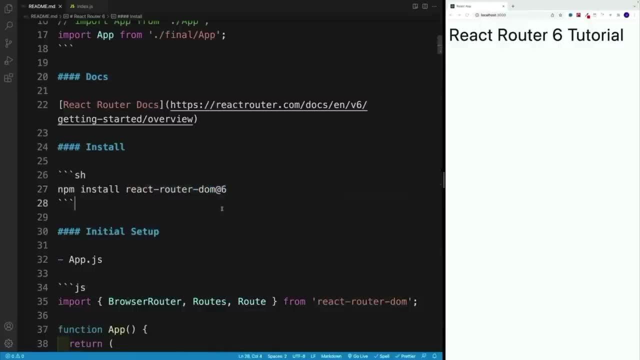 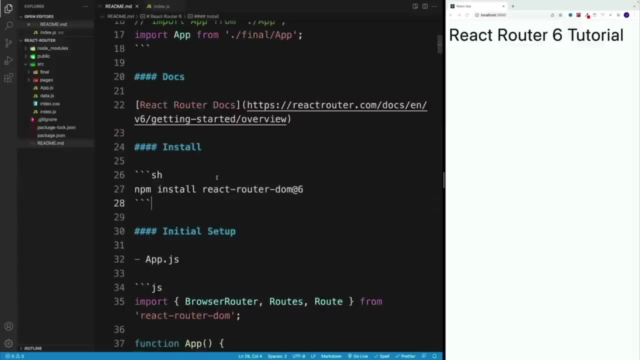 docs of react router six. And when it comes to install for your own projects, the command you're looking for is npm: install react router DOM at six. Now, of course, I already installed this package in this project, But just so you don't think that there's some funny business going on. 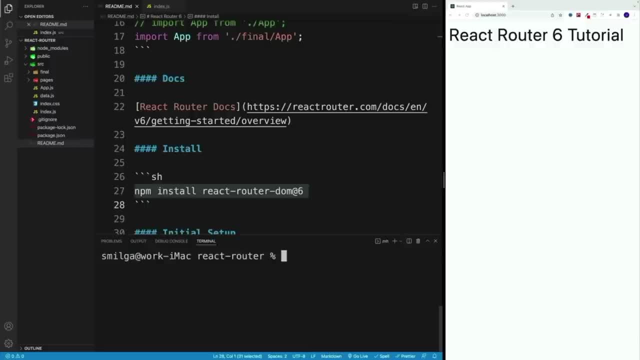 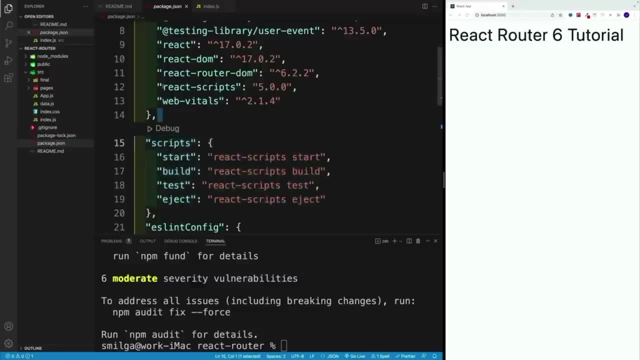 Let me open up here the terminal. Let me open up here the terminal. I'll clear everything around the command And once the install is complete in a package JSON, we'll see or react, router DOM package And as far as the setup, here's what we want to do. 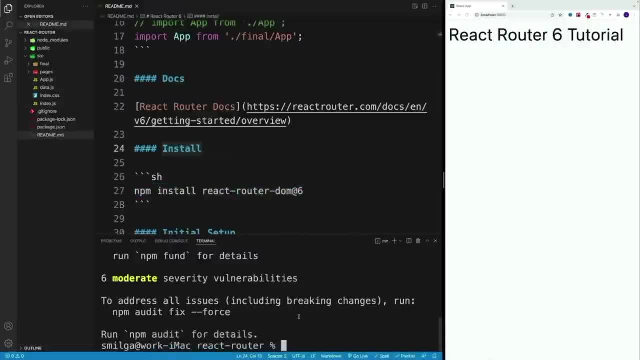 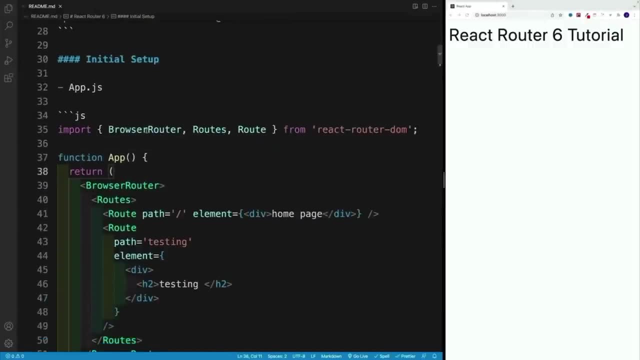 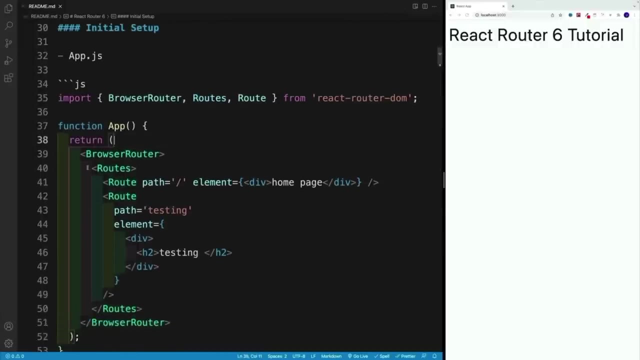 We want to go to app js And you're not going to start this one up, So npm start. And we want to import three things: We want to get the browser router, which is going to connect to the actual browser, the routes component, which is going to be a parent for all our routes, and then route. 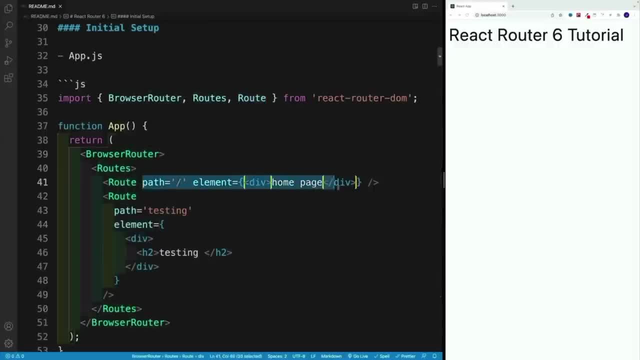 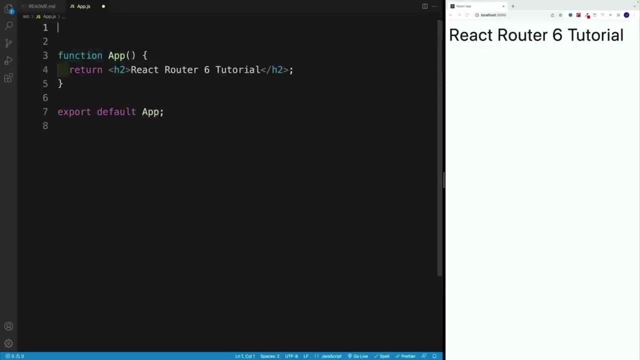 component which we'll use to set up a single page. So let's go there, Let's start setting up the code, And then I'll talk about the props and the rest of the stuff. So let me first navigate to app js. Like I said, we want to grab three components Now. eventually we'll also get a link. 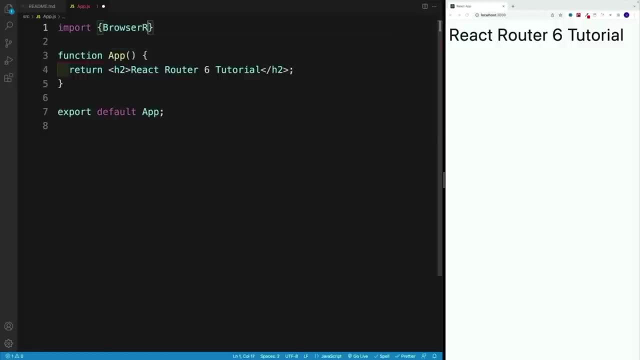 which is going to be the browser router route and route. And as a quick side note, if you want you can add browser router in the indexjs, basically where you wrap the whole application. but in my case I'll sell for app js. then we want to go with react and then router DOM. 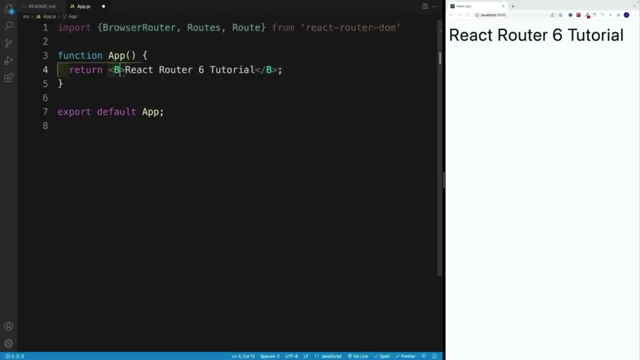 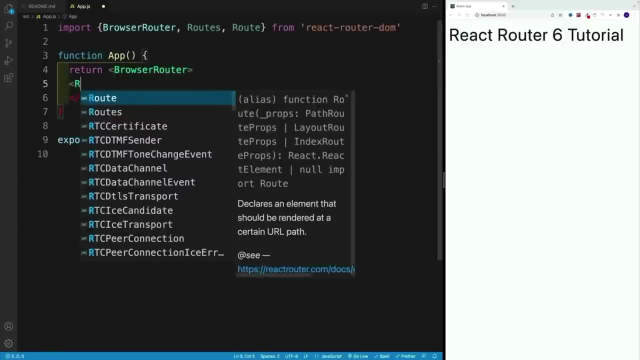 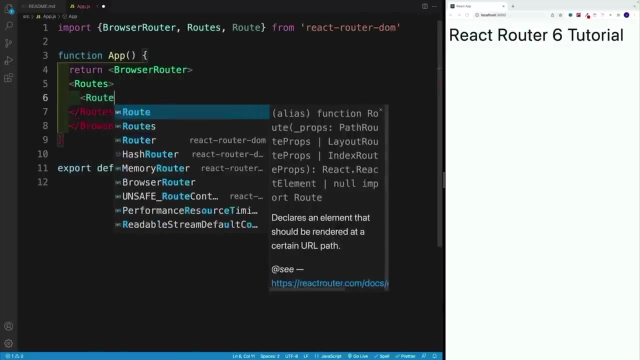 And, like I said, first we want to connect to the actual browser Go with browser router. then we'll set up the route component. So let's go here with routes And then we need to set up those single routes And basically the idea is following where we go. 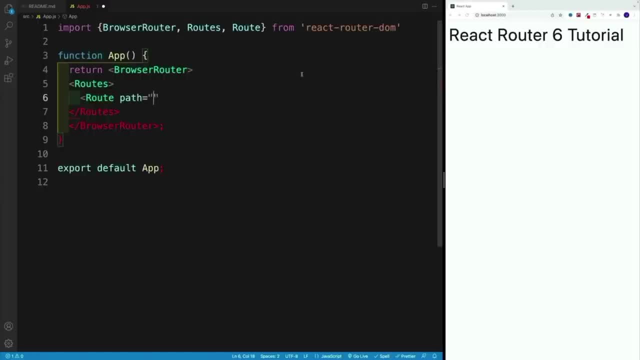 with route, then we need to go with path. So this is going to reflect whatever we have in the URL And when it comes to the homepage, we have special syntax where we go forward slash. Now, in this local setup, that forward slash means localhost 3000.. In production that is going to. 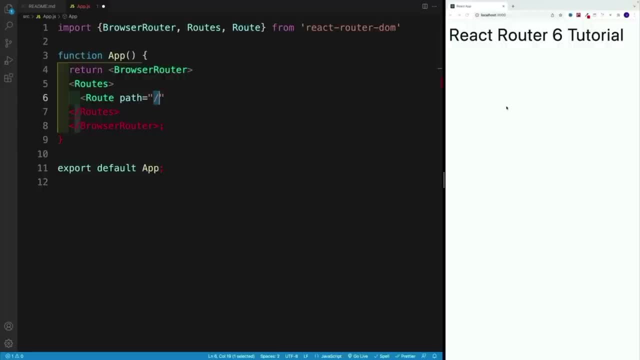 be, whatever is your domain, whether that is udemycom or youtubecom or johnsmilkcom, And hopefully you see where I'm going with this. So this is special, this forward slash, But basically where we have the path will set up whatever URL is going to be here in the URL bar. 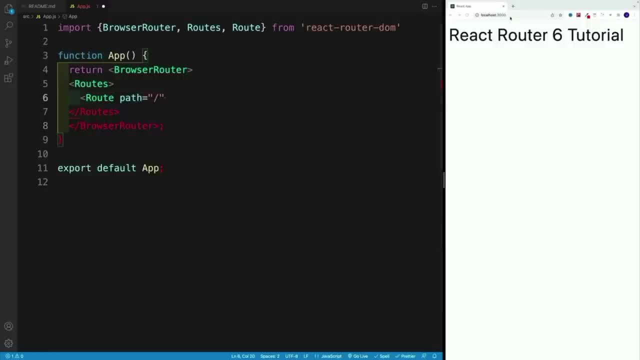 So, for example, I want to have a page by the name of testing, then instead of forward slash I'll type path equals to testing. And if I want to set up a nested one- let's say I want to go with products and then forward slash info, then yes, you guessed it. One of the ways how we can set it up is going: 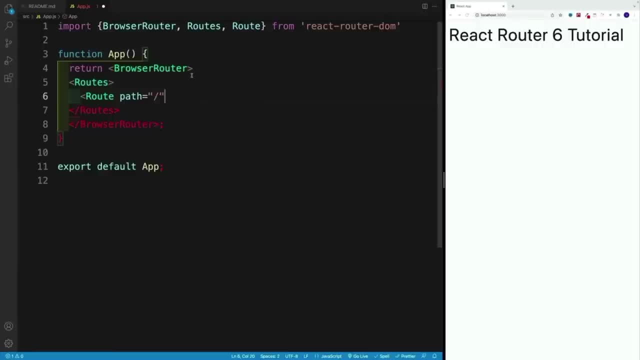 with products here and then forward slash testing. And if you're a little bit iffy on that, don't worry, as we cover more examples it's going to be easier to understand that. So first let's go with path forward slash- again, that means our homepage- And then we want to go with element And 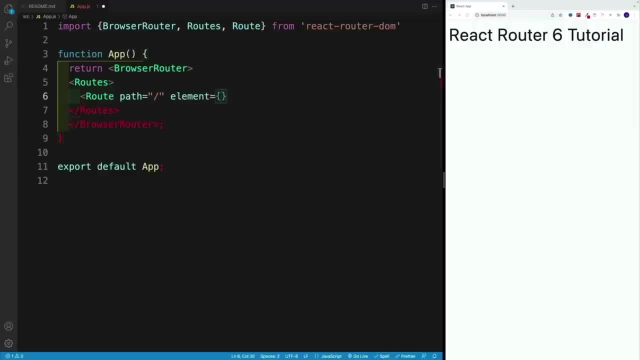 at the very basic level we can just pass in the code directly here in the element, And in the upcoming videos we'll see how we can use components for that. But at the very basic level we just need to set up here what we want to see on the screen. So in my case I'm going to go with 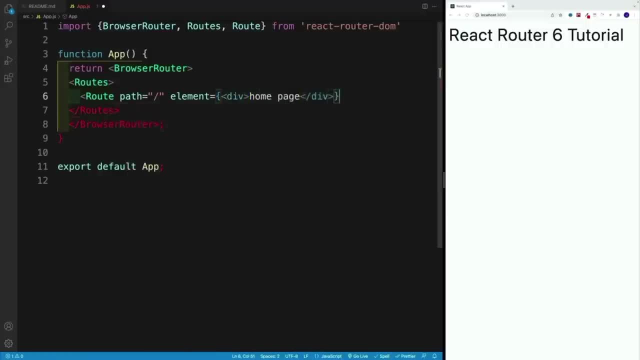 simple div here And I'll say homepage, like so. So let me close out the route component And once we save we should see homepage, and we do So. that is my homepage And, like I said, now let's set up some dummy page And I'll call this testing. So instead of forward slash, which 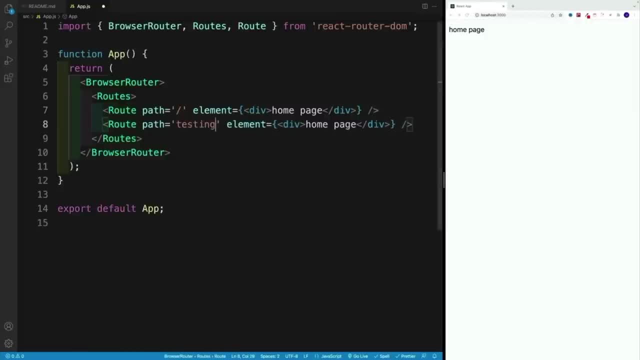 is a syntax for the homepage. I simply go here with testing. Now, if I'm going to write about, then of course in the URL I'll have to type forward slash about. Now, if I have testing and you guessed it, I'll go with forward slash. 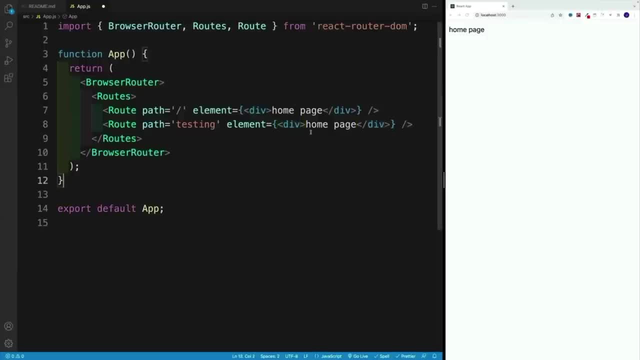 Testing And what I want to display here. well, let's make this one a little bit more complex just to showcase that of course we can set up whatever logic we want over here. So I'm going to go with div, And then inside of it we're going to go with heading two, And then the testing. 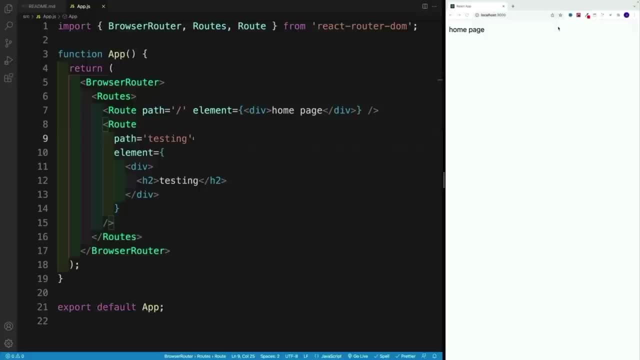 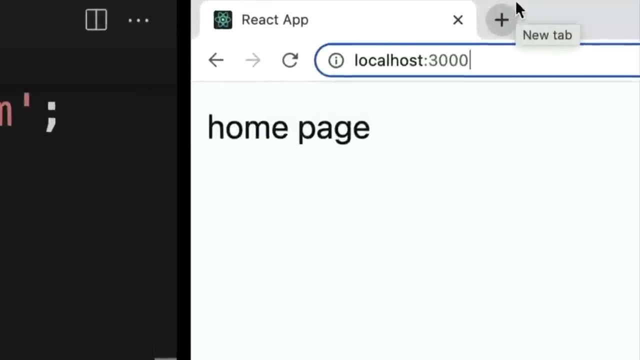 let's save it. And eventually, of course, there's going to be a navbar and all of that cool stuff, But for now, yes, we'll have to do all the navigation in the URL bar. So let me navigate there. And what is the page name? So I'm going to go with navigation, And what is the page name? 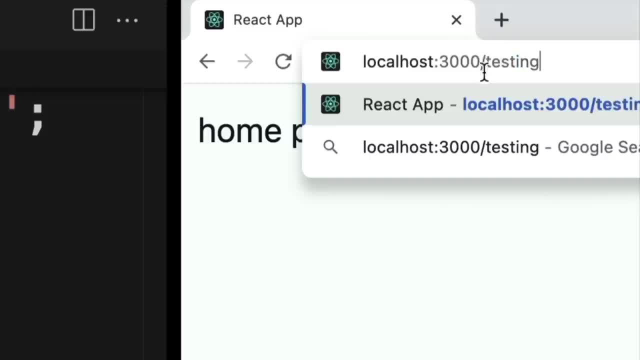 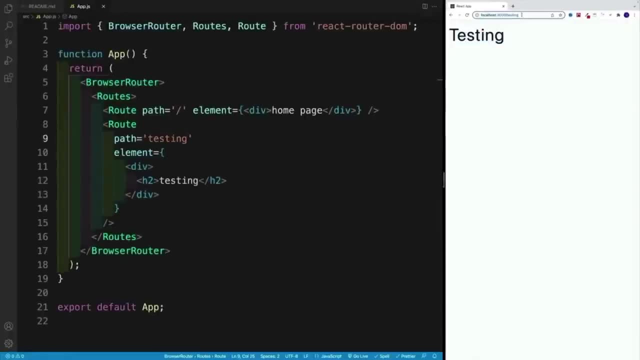 Well, it is testing correct. So we go forward, slash and then testing. Once we navigate there, check it out. Now we have our page And if you want to go back to the homepage- you guessed it- we just need to go back to the localhost 3000.. So, again, we install the package. 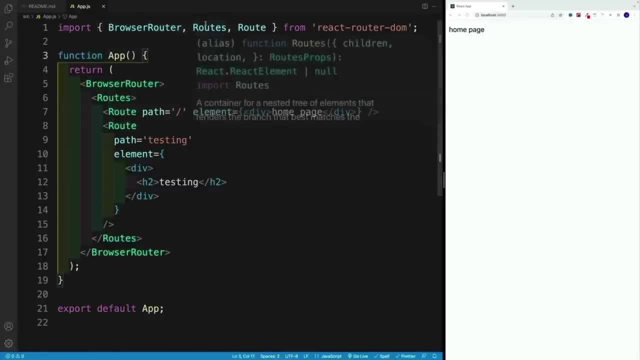 we grab three components: browser, router, routes and route browser. our connect to the browser routes is going to be a parent for all our routes And then for every page we'll set up a route component with two props: a path. So what is going? 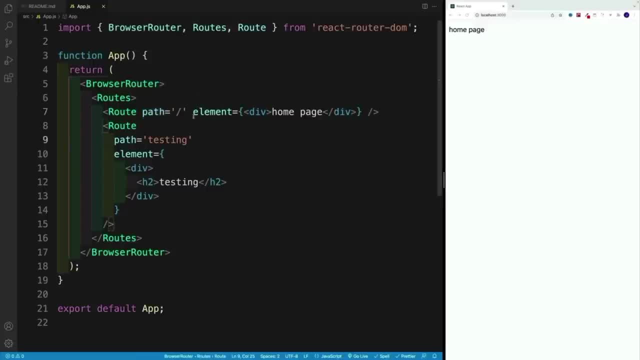 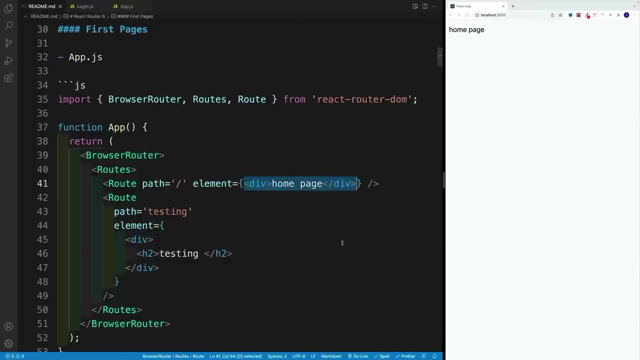 to be the URL And then what we want to render, we pass into the element. Not bad, not bad. we created our first pages. Life is great, But you would have to agree with me that, when it comes to any realistic application, hard coding the page content in app j s. 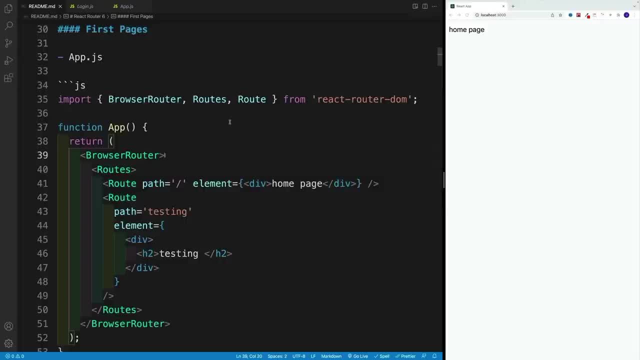 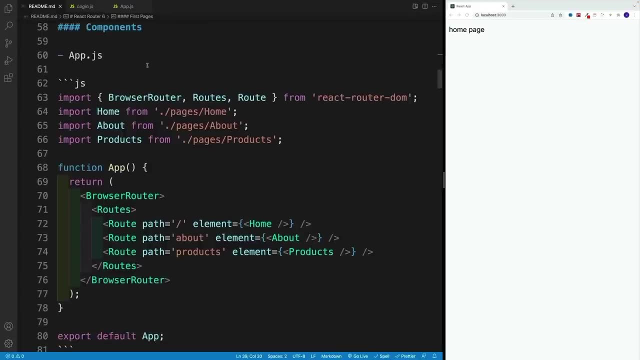 is probably not going to be very good on your health. you'll just end up screaming at your computer. So here's the thing we can also pass in component directly. So path setup stays the same Again. whatever we type over here will match in the URL bar. So if it's forward slash, then it's. 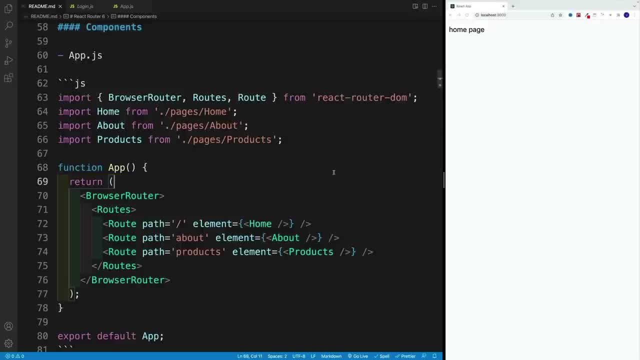 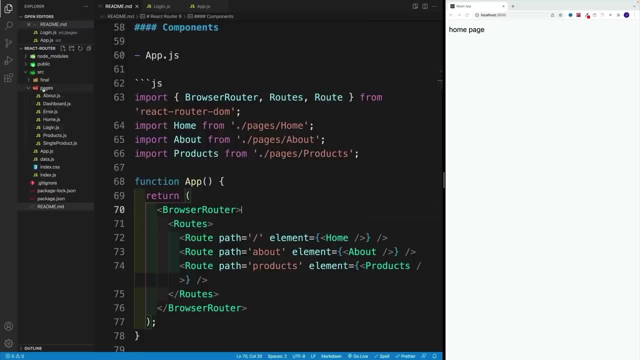 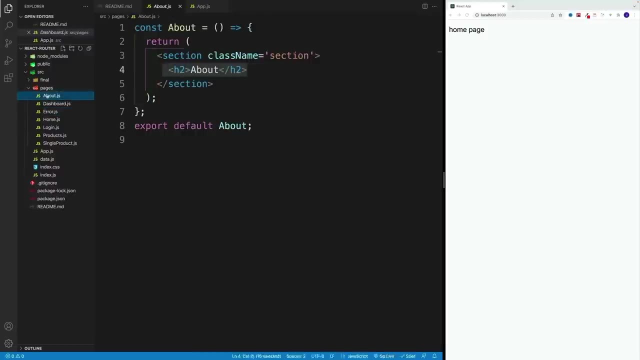 home page If it's about. hopefully you see where I'm going with this. But when it comes to element, we can pass here the component And therefore you'll find in the pages bunch of components. Again, the only reason why I set them up is just so we can save a little bit of time on setting up. 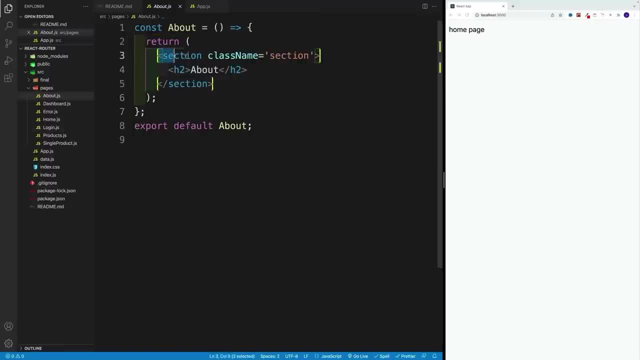 the boilerplate. So for the most components you'll just find this section with the class name of suction. So in here we just add a little bit of CSS. you can take a look at it in the index, CSS, and heading to with about. 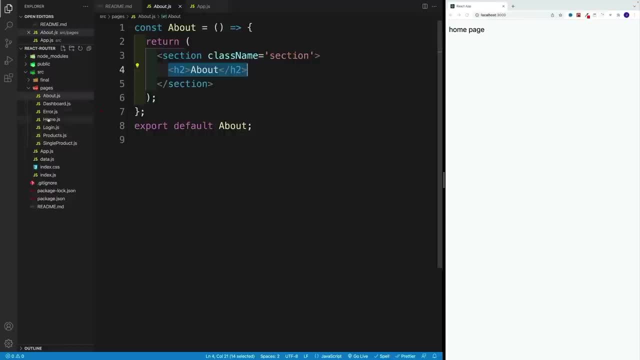 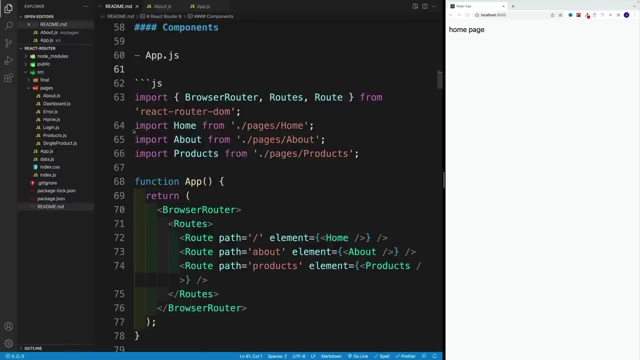 Speaker 1. So please are the pages that we will have in our project. So here's what I want to do. I want to go to appjs, I want to import them all. So for now just home about and product Notice all. 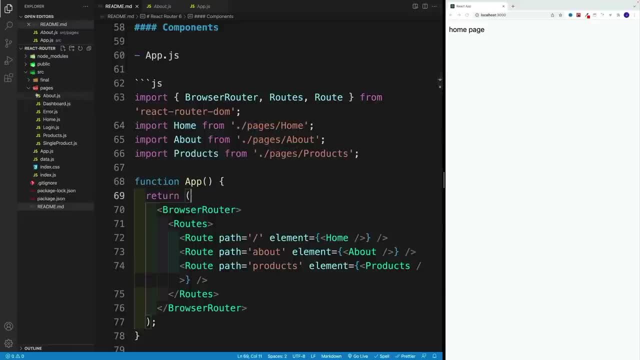 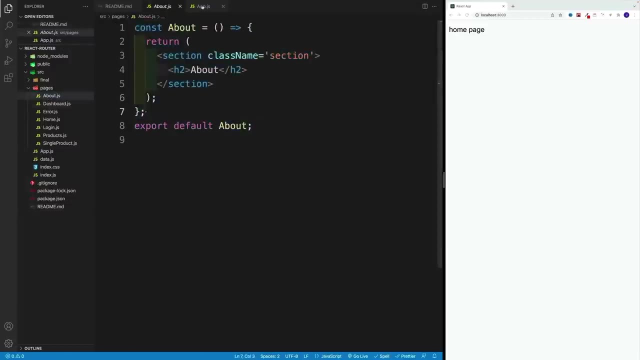 of them are coming from the pages And, as I know, of course you don't have to name your folder pages. It can be anything. It can be banana pudding And also. there's nothing special about these components. They're straight up components. The only difference is that 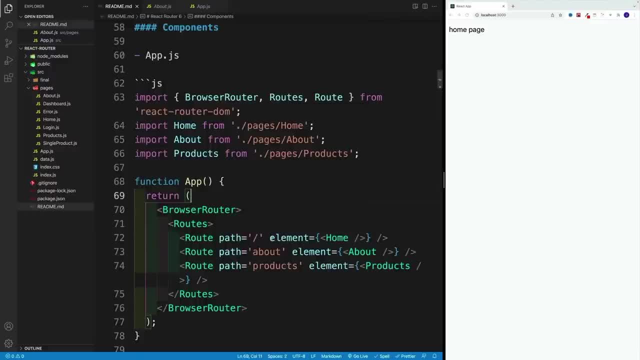 now we will use them in the appjs And we'll pass them into the element prop And, as a result, whatever we have in the component will be the content of the page. And yes, in those components you can import another component, which also is something we're going. 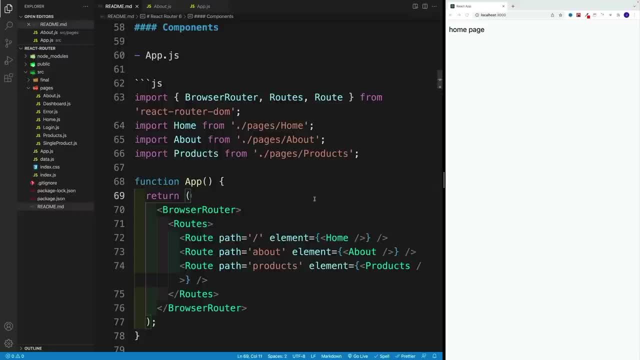 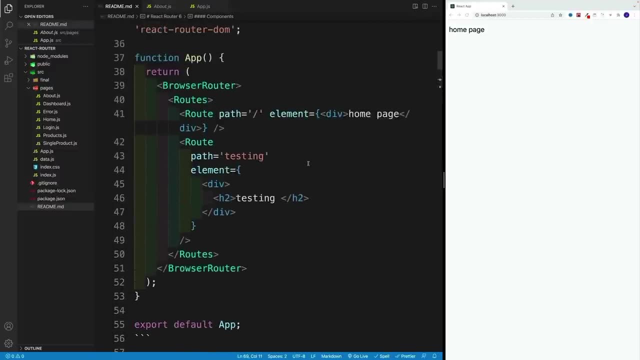 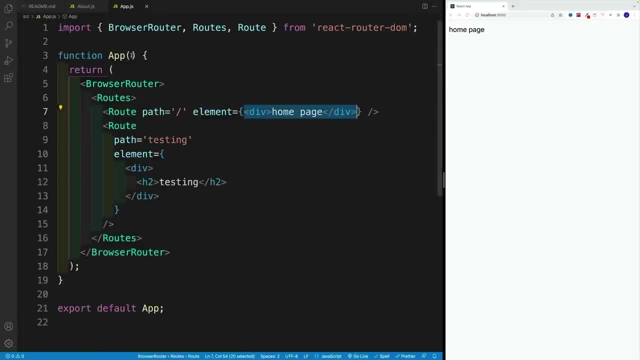 to do And, as you can see, as a result, it's going to be easier to manage your application instead of hard coding everything in the app. Yes, So let's try this one out, where I want to go to appjs And I want to import three. 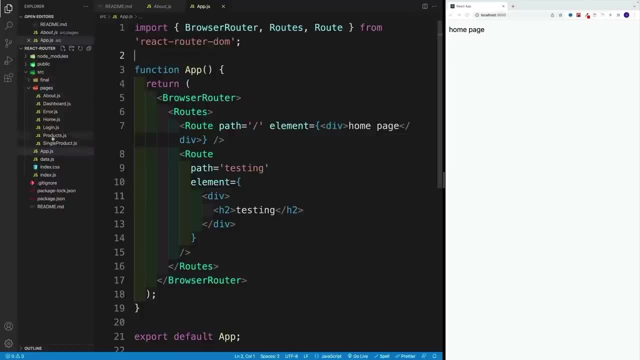 components. And lastly, if you want to set up here index- Jess, that is your preference- or basically, in the pages you import all of the components and then export them, You can also do so, But in my case I'll just go the along. 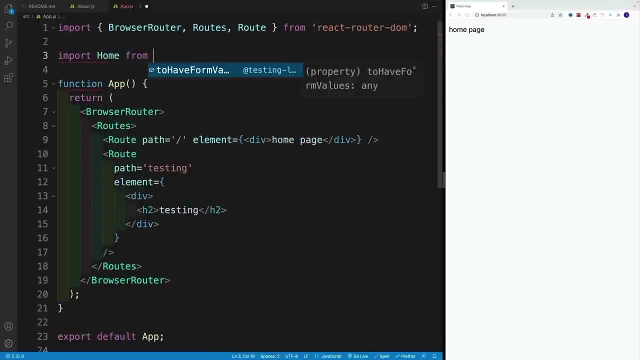 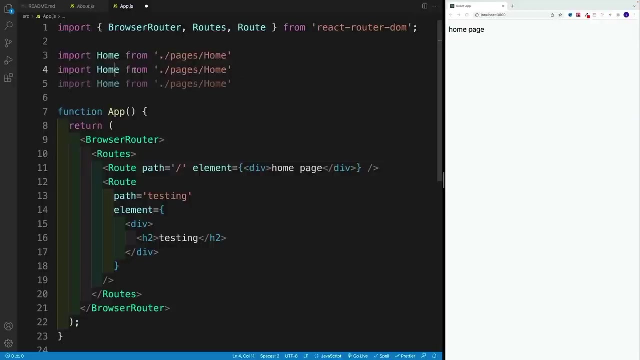 route Where I'll say import, then home, And then that one is coming from And I'm looking for the pages folder, more specifically home one. Let me copy and paste here. Let me just change a few things around where I want to go with a about one. So let me select that one And 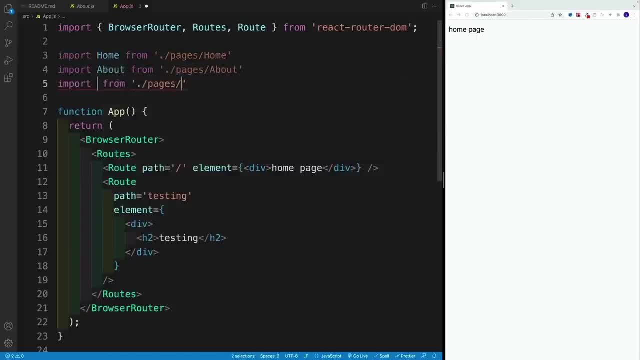 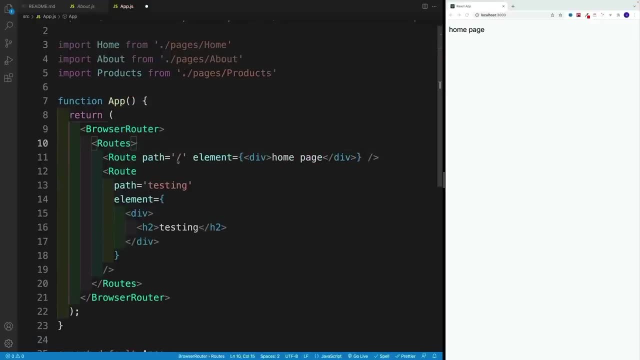 we also want to go with the product. So let's go here And let's say products, And once we have all of the imports in place, Now let's keep the path forward. slash again. this is going to be for the homepage, But let's change around for testing one, where I will remove it first. 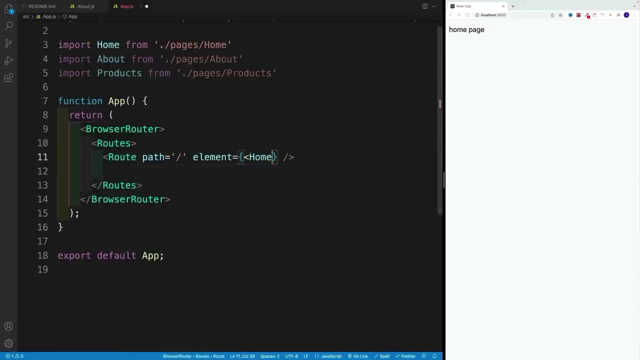 And I'll actually pass here the home component. Let's close it. It's also necessary And check it out. Now we have that item to let's copy and paste And let's just change the round where going to be about, And this one will be product. 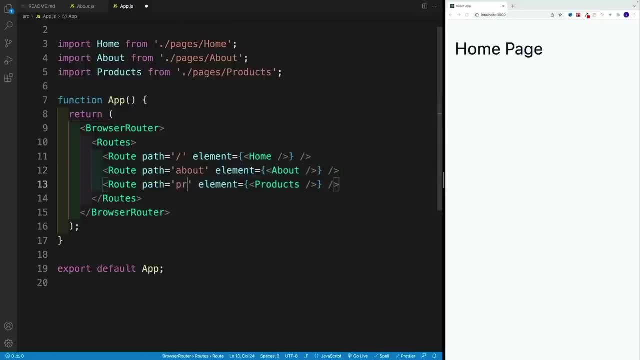 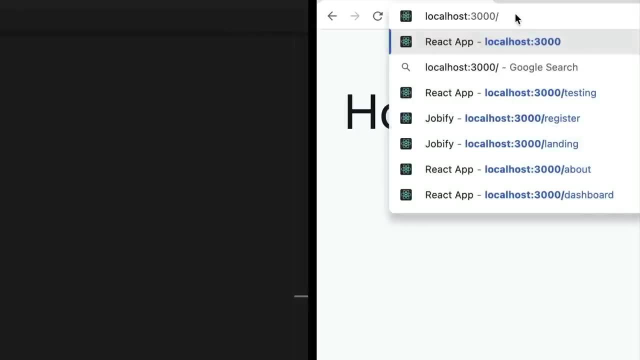 And when it comes to path in here we'll say about as well as product. And again, we can test it out if we navigate to URL And then if we go with forward, slash about check it out. Now we have about page. Now you can probably already guessed that if I'm going 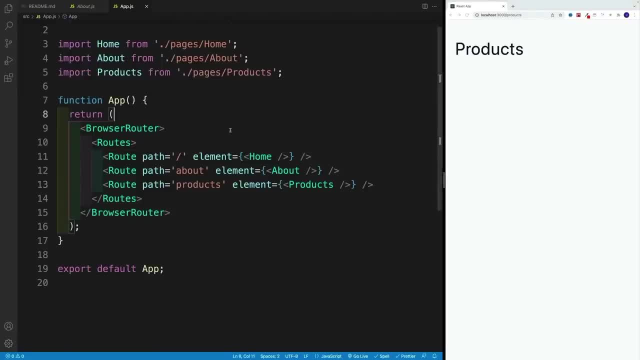 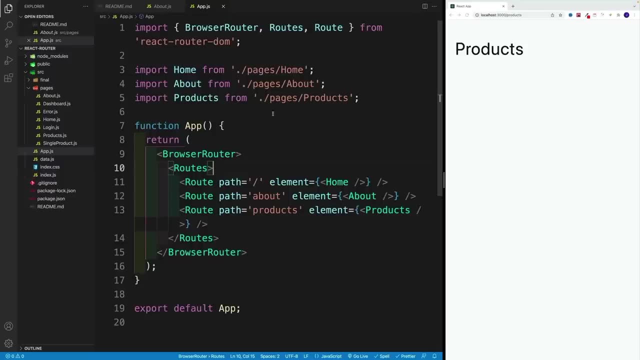 to go to product, we'll navigate to the product page. So that's how we can set up our page content as components. Again, we set up most likely a folder, Since there's going to be multiple pages, And we just set up straight up components. 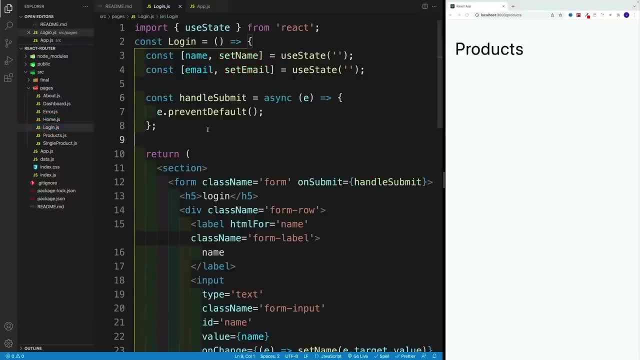 There's nothing special about them. Straight up components. The only one that has more info on here is the login one, But we'll talk about this one a little bit later, Once we actually get there. whatever you set up over here, whether that's a bunch of other components- 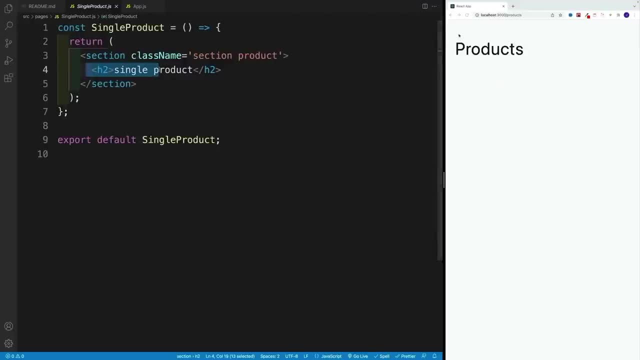 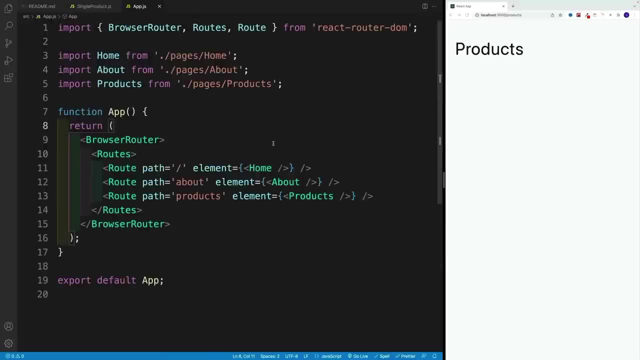 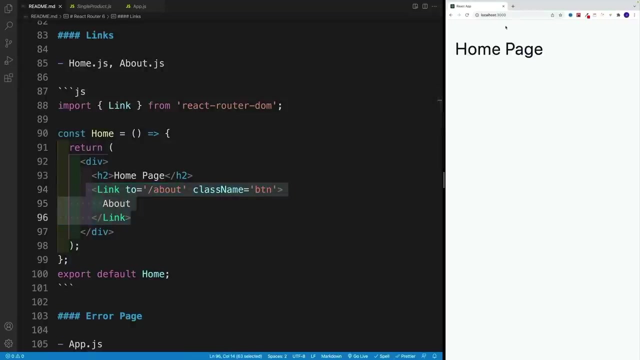 coming from other folders, and all that will be the content of the page. As a result, it's easier To manage your entire application, Alright up. next, let's take a look at how we can navigate around our project, Because at the moment, the only way how we can do that is using URL. 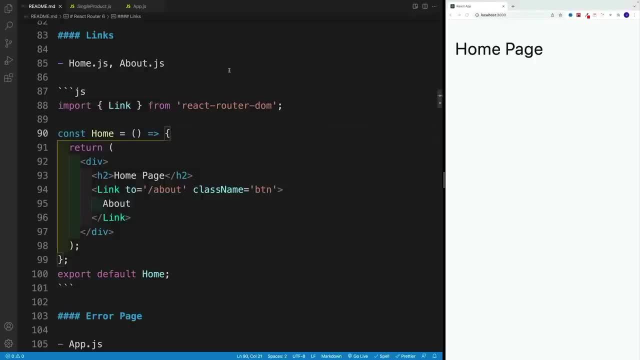 bar not as probably not the best user experience, Unlike the traditional multi page application where we use the href, the link element, In this case, if we want to navigate around our project. so, internally, we want to grab the link component from react router dump. Now, if we want to go somewhere externally, 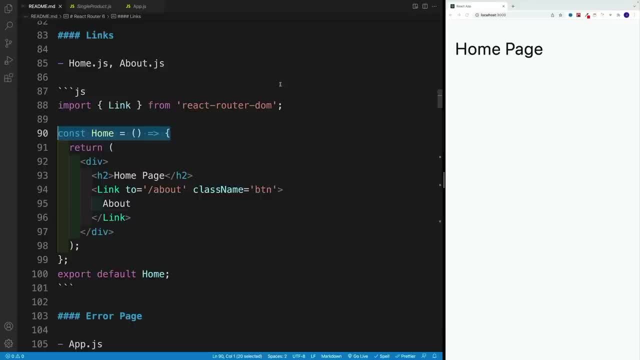 for example, if I want to go to googlecom or johnsmilkcom, then yes, you still need to use the link component, like so? So you'll set up a link component, href, and then whatever the URL, But in order to navigate around our project, we'll use the link component instead. 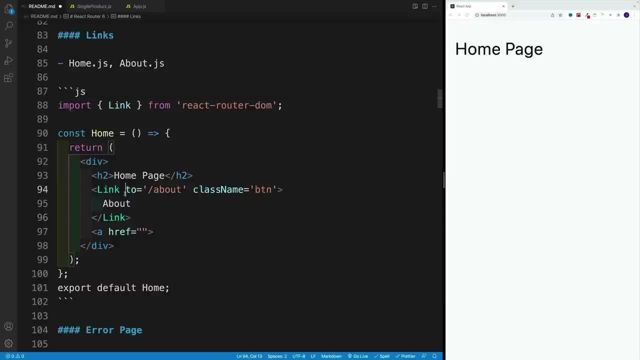 And then the link component is looking for one thing It's looking for to prop and the notice, which is pass in the URL. Now again, we don't need to go with full URL In here, we just need to go with forward slash and then whatever. 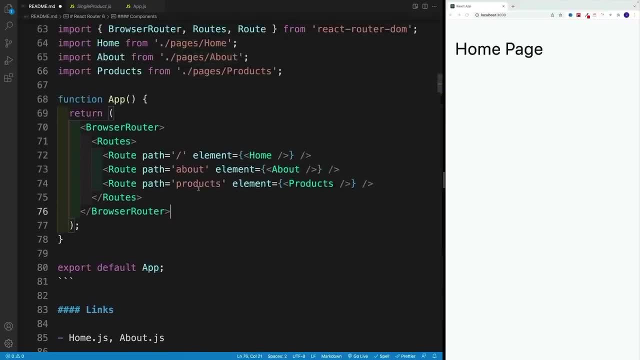 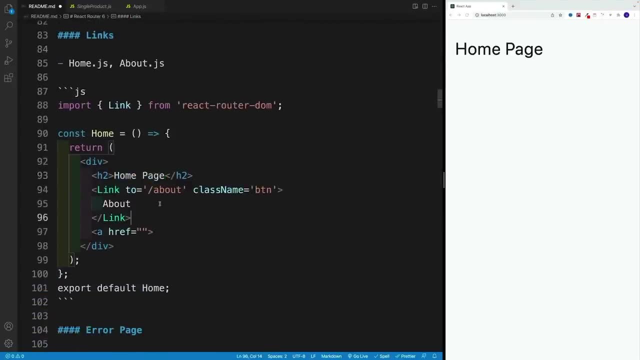 we have in the app. Yes, So since I have these pages forward slash, so the homepage about and product kind of makes sense. if in the homepage, if I want to go to a bold page, I need to go forward slash and then the next page is going to be the previous page. Here I'm looking for a 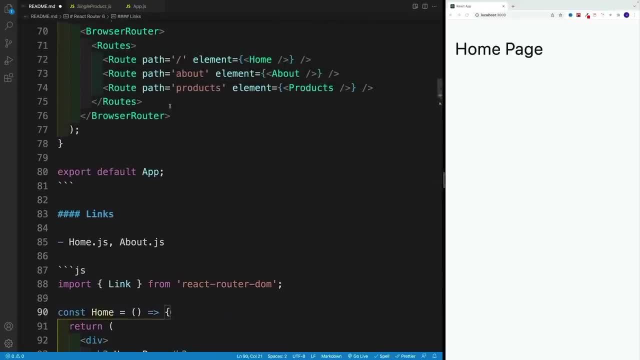 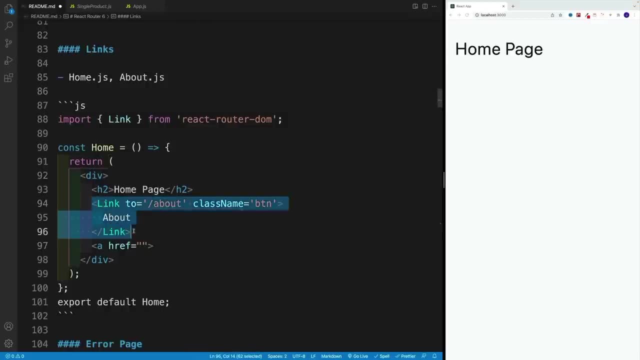 the name is about. now these ones do need to match, So make sure that the syntax is correct. So in HomeJS I want to set up a link to about just, right after the heading two, And in the about just I want to set back the link to the homepage. So let me try this one out. 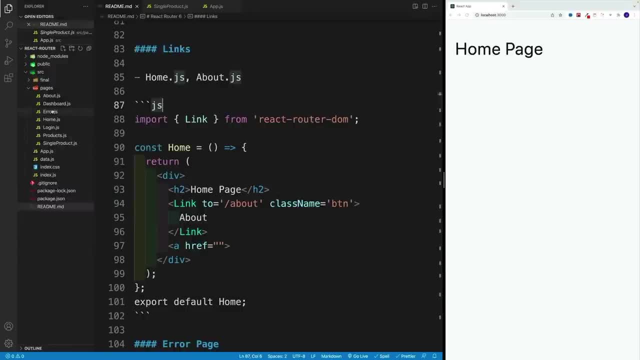 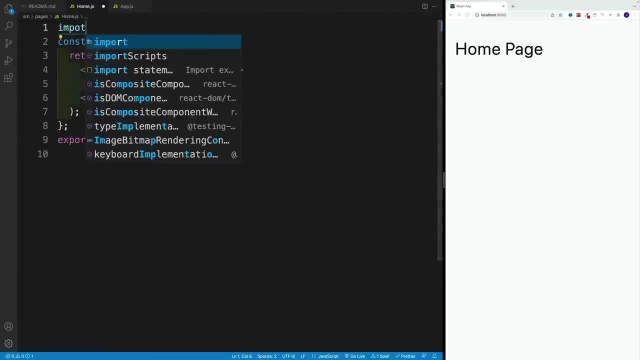 Where first I guess I'm going to go to the homepage. So let me navigate through the pages. And we're looking for HomeJS when we want to get the link one. So import, it's a named, imports a link from react router, DOM, And then, right after the homepage, let's go with. 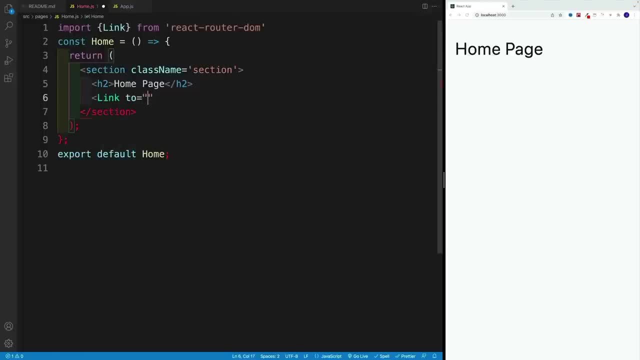 link to: And again I want to navigate to your product, I'm going to go with forward slash product. If I want to go to about, I'm going to go to forward slash and about, And let's add a name. So whatever we want to display here and a little bit of styling, therefore, 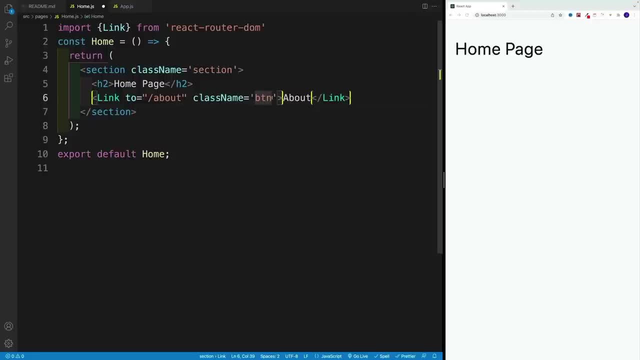 I'm going to go with product. So I'm going to go with product. And if I want to go to product, I'm going to go with product. And if I want to go with product, I'm going to go with class name. I'm just gonna say btn. So once we save notice, now I have this link. 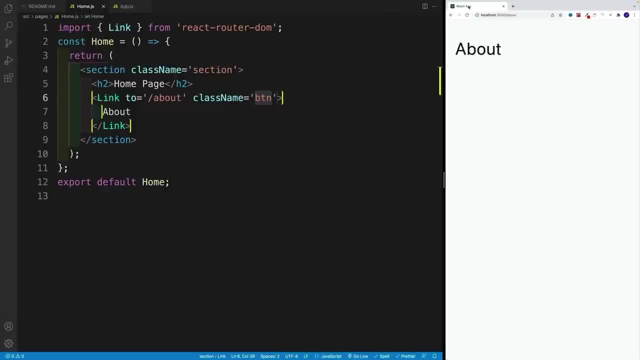 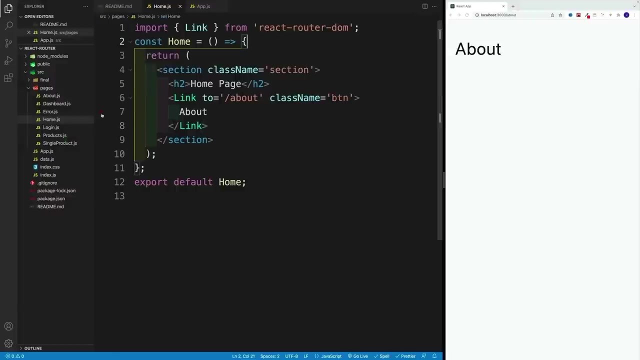 to the about page. Now we navigate to about without that full page refresh, And in order to make this a little bit more interesting, why don't we also do the same thing in the about? So then we'll be able to go from one to another one. So let's go to about j s. 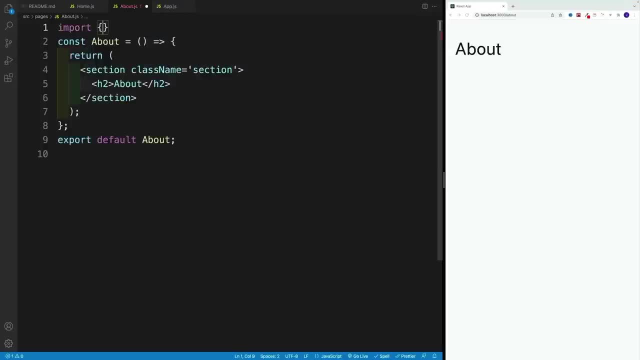 Same deal. We want to grab the link, import And link. probably should have copy and pasted, But anyway, so react router down right after the heading to. let's go with link to in this case. I want to go back to the. 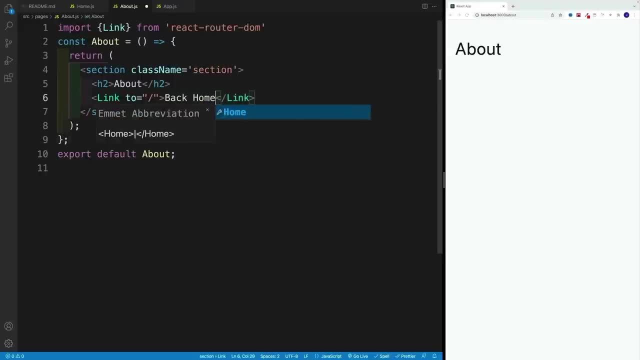 homepage, say back home, And then let's also add that class name- a little bit of styling- class btn. So now we can nicely go from page to page without that full page refresh. Again, if we want to navigate around our project, we want to grab the link component. it's looking for one thing and 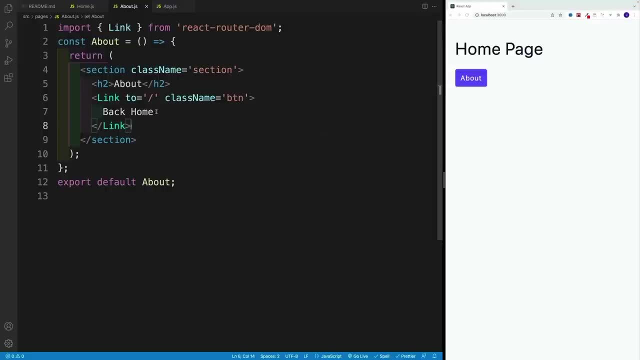 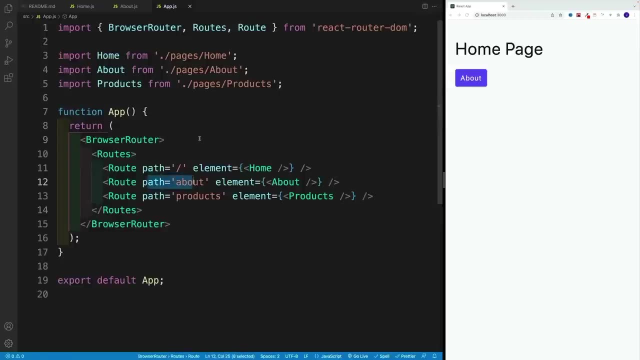 one thing only looking for: to prop, And in here you want to pass in the same value that you already have here as far as the path. So if you want to go to about, you go forward, slash about. And if you want to go to product, you go to forward, slash product and hopefully, 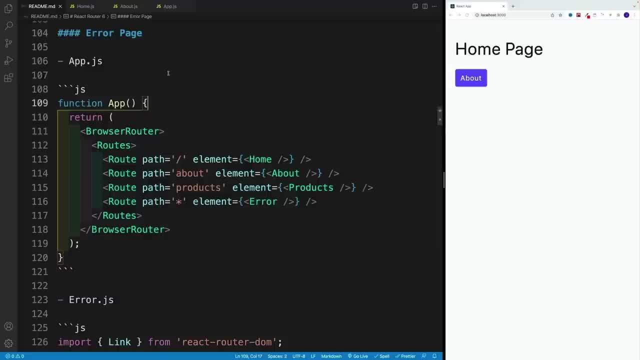 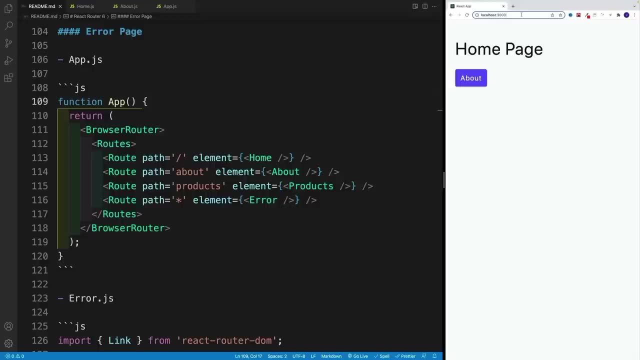 you see where I'm going with this. Okay, well, what if, by mistake, the user typed the product? they typed some kind of path that doesn't exist. So let's say I'm going to go with forward slash And then hello, the moment basically will display nothing. Why? Well, because if 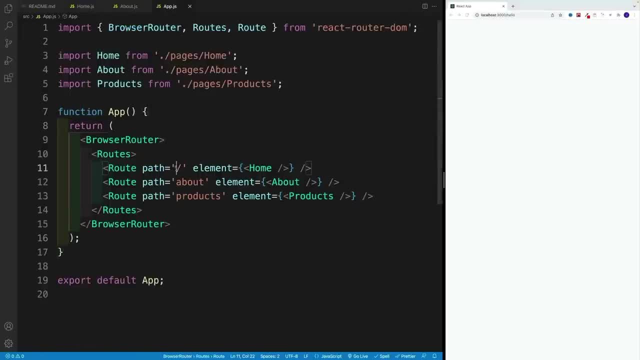 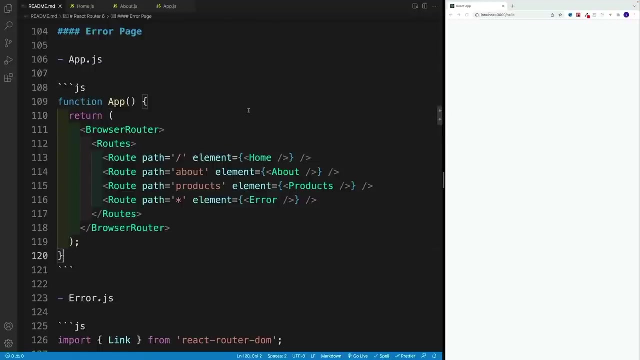 we take a look at our app, Jess, we're only handling these routes. we have forward slash on and about on product And in order to handle this type of scenario, we want to set up an arrow page. essentially will display some kind of error message for every request that doesn't match. 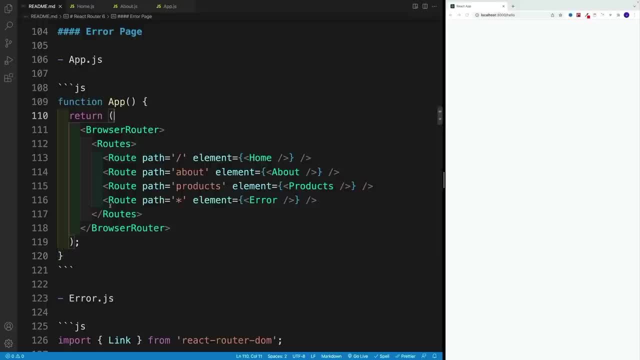 any of our routes And we want to do that with a route component. we want to pass in the path with a star, So essentially this will match everything. So if we cannot find those pages over here, then this will collect all of them. And then we want to set up some. 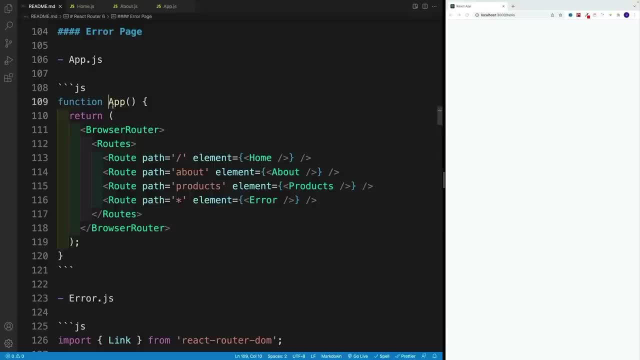 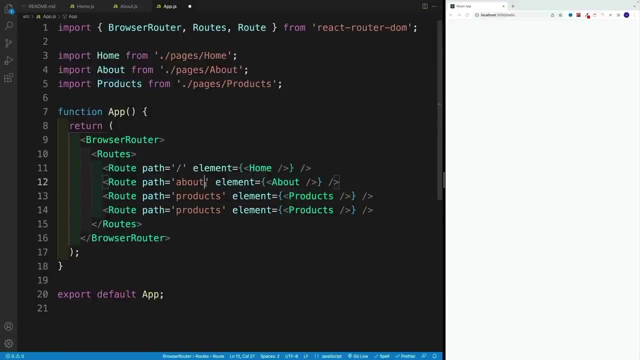 kind of error page. So first let's set up this in the app dress and then we'll work on the error page. Now there is already a page in the pages, But I just want to add a little bit more content. So first let's go to address, let's copy and paste And yes, 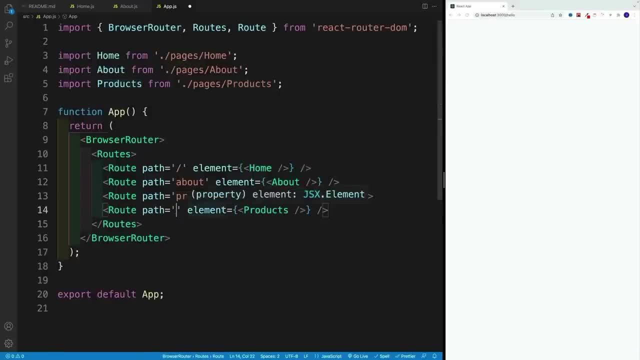 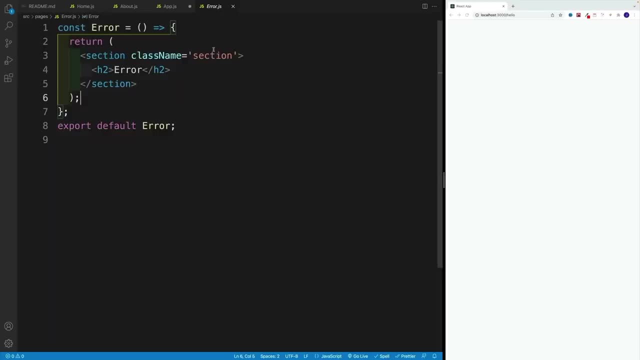 we want to place here all the way at the end, because this catches pretty much everything. So we want to go here with a star And now let's work on the error page, Or essentially, at the moment, again, we have this. 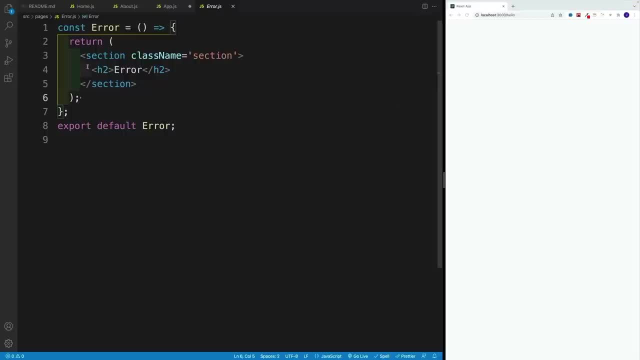 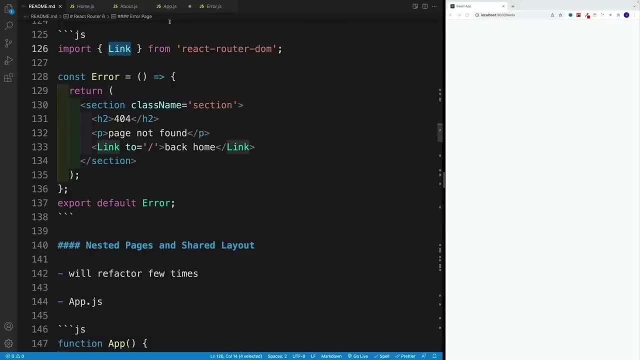 section with a class of section and heading to with an error. But I want to set up a link back home And, as I know, this is what we're going to be working on. So we want to get the link component from react router down. we want to add some kind of logic. So 404. 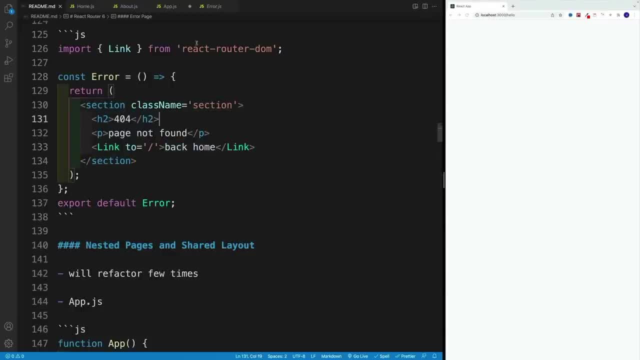 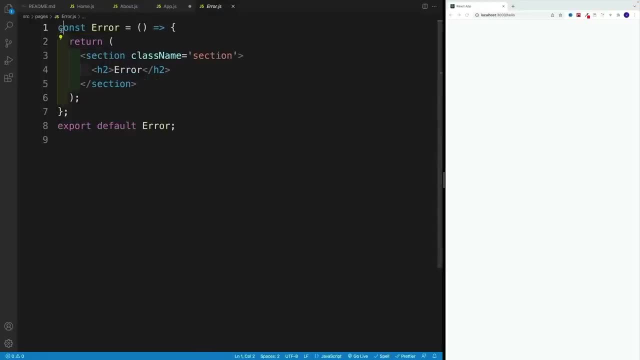 page not found, And then we want to navigate back home. So let's try this one out, where, in this case, I'll speed this up, I'll grab the link, Since we'll need that one. Then, after the heading to where you know what, let's change this one around where I'm gonna. 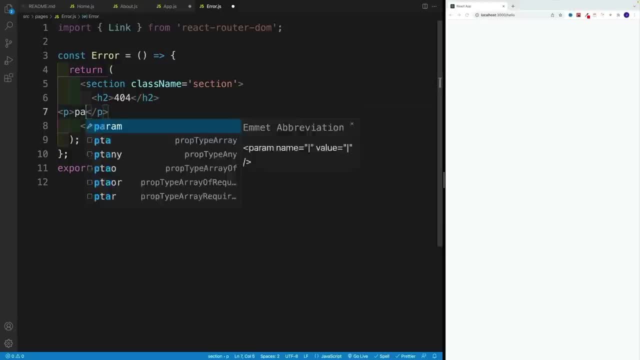 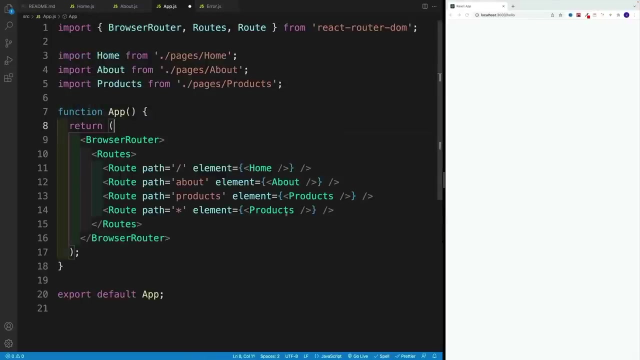 go for four. So page not found, a paragraph, page not found. And then we want to go with link component to where I want to navigate. well, I want to go back home, And in this case let's just say: back home, let's save this. we want to import the page, So let's. 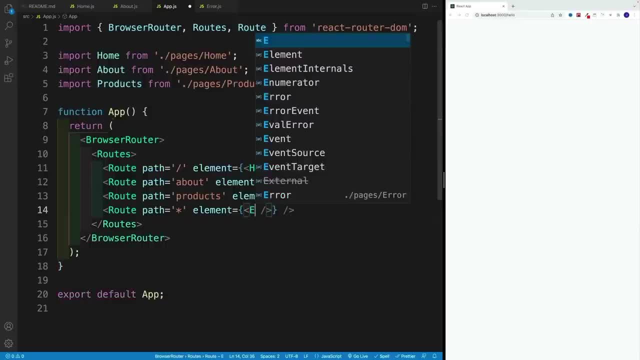 try out the auto import. So I'm going to go here with our and let's say that, And then it's in the in the dialog box here. So once I pull this out, I can just drag this one all the way down And we're going to create our page And then let's save the paragraph. 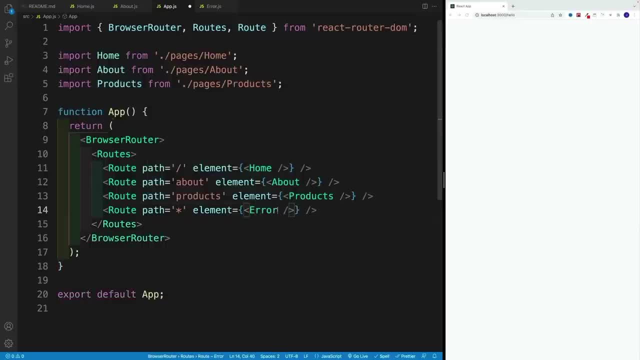 page And let's save this. So we want to import the page. So let's try out the auto import. So I'm going to go here with error And let's see how this works. You can see, you're see whether I got actually the page. now it doesn't look like it. So let me try one more. 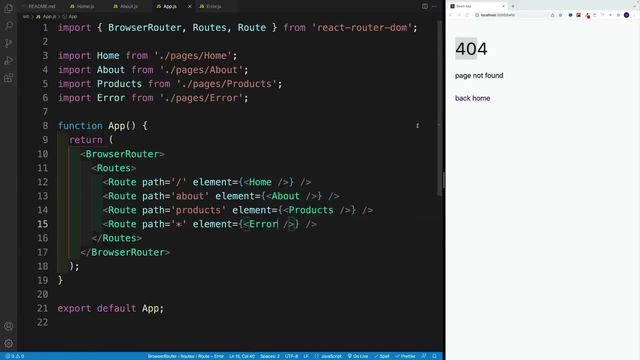 time, Yep. Or here I can use the auto import And notice: now we have a nice 404 page. So if I'm going to go with forward slash and this thing, same deal, we don't have that particular page in our project. So basically there is no URL that matches that And therefore 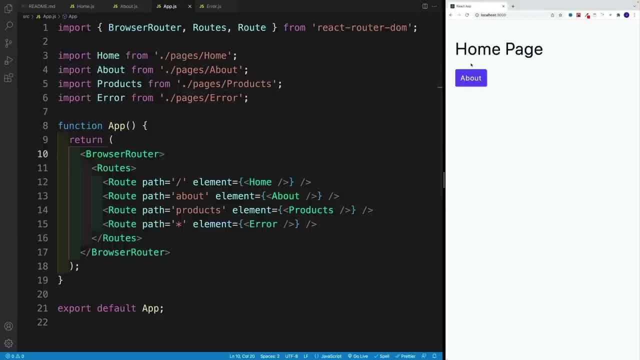 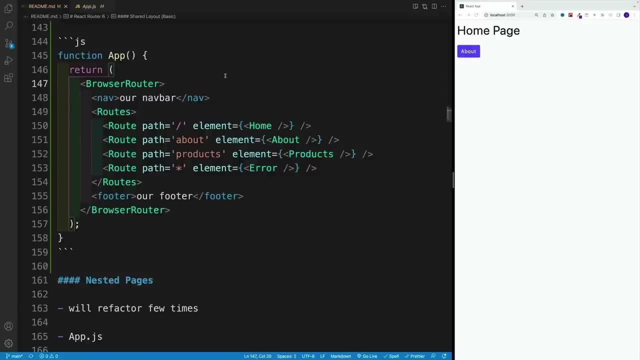 we display this error page Now. if we click on back home, we naturally navigate back home All right up. next, let's see how we can add navbar and footer to our project. Now, in this video, I'll quickly show you the most basic approach, which clearly has its limitations. 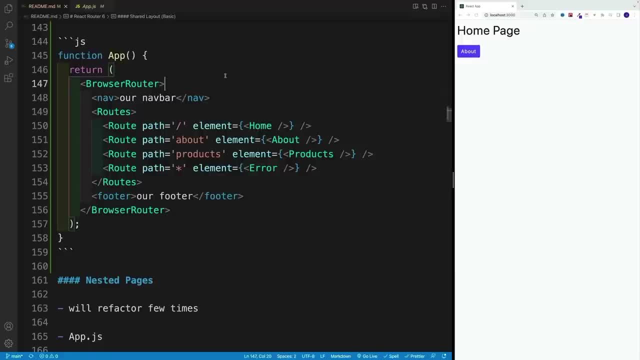 since it adds the same components or elements to all of the pages. But don't worry, in the following videos we're also going to cover more fine grained approach Where we will nest our pages and set up the shared layout And as far as the basic setup, 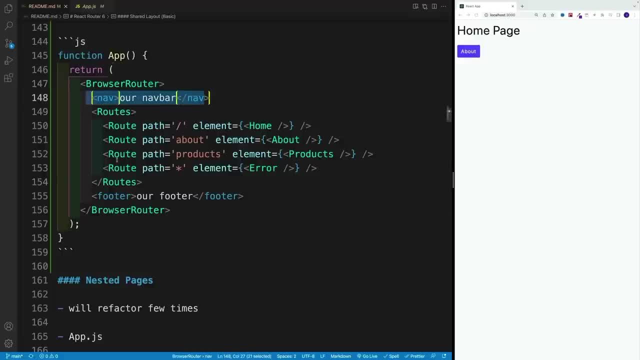 we simply want to set up the elements above or below the routes. Again, please don't make the mistake and place the element inside of it. you will get the nerve, But if you place it above or below the routes, this will be added to all of the routes, like I said, most. 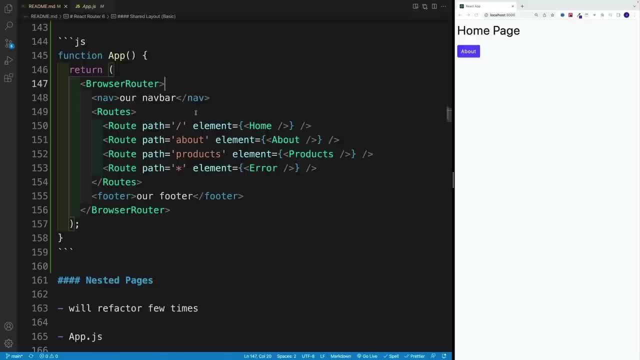 basic approach, But there's definitely situations where you're going to have to add elements to all of the routes. And if you're going to add elements to all of the routes, you can add elements to all of the routes. like I said, most basic approach But there's definitely. 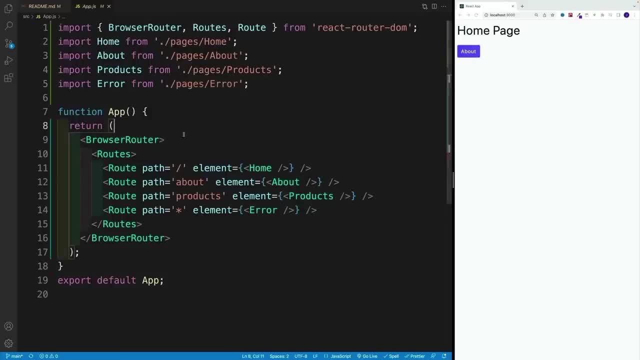 situations where this is a nice solution. So let's navigate back. Let me go above the routes. Let me set up the nav component, basically an element, And yes, of course, you can set up the component imported here, And also, of course, you can add the links. 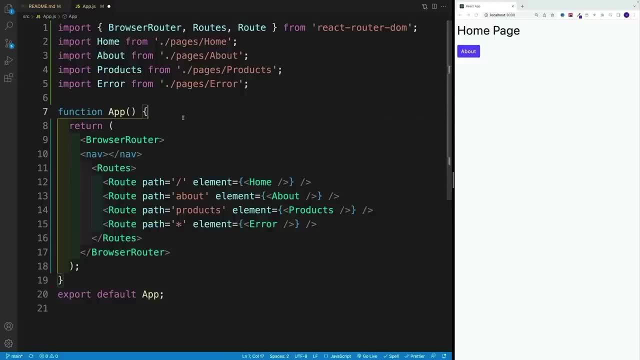 Now I'm not going to add the links in this scenario, since we're going to do that in the upcoming examples And I don't want to repeat myself and waste your time. Basically, I'll go here with our bar And the same thing we can do with footer. I'll say our footer And once you save, you'll. 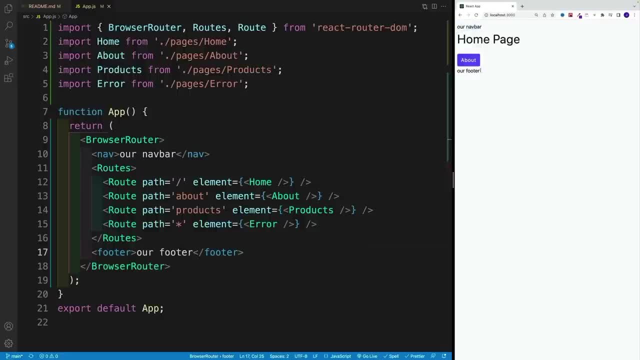 notice that in all of the pages we have the navbar as well as the footer. If we navigate to about same is going to work with product And it's not going to be surprised if we navigate to another page and we get the same result. navbar and footer gets added to all of the 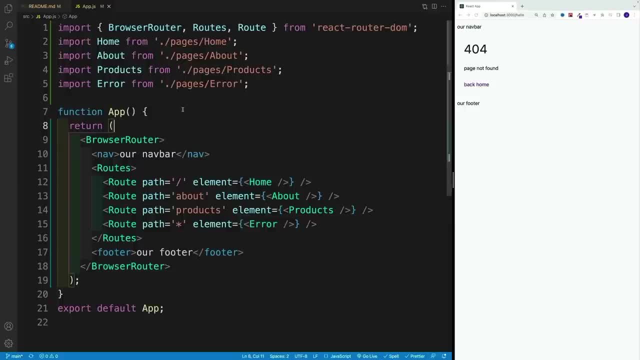 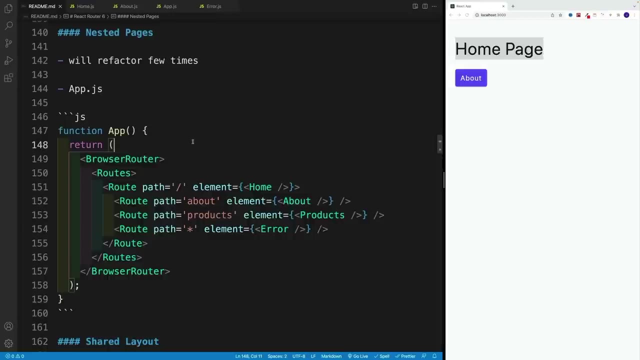 pages. So this is the most basic approach, how we can set up some shared layout where essentially, in this case, we're adding both of these elements to all of our pages. All right Up next, let's add a navbar to our project And, in the process, 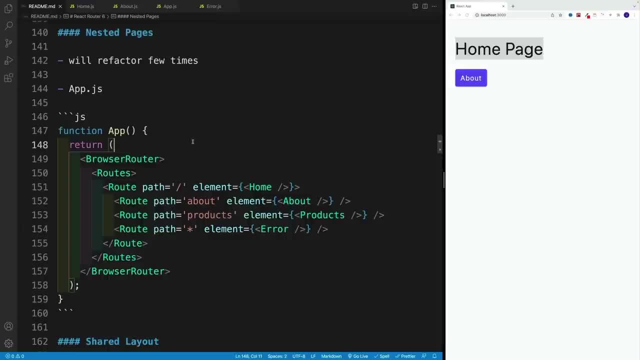 we'll learn how to set up nested routes, shared layout and index page. Since I want to cover everything step by step, please be prepared to factor our application a few times. And if I want to nest some routes inside of the another route, I just need to go with. 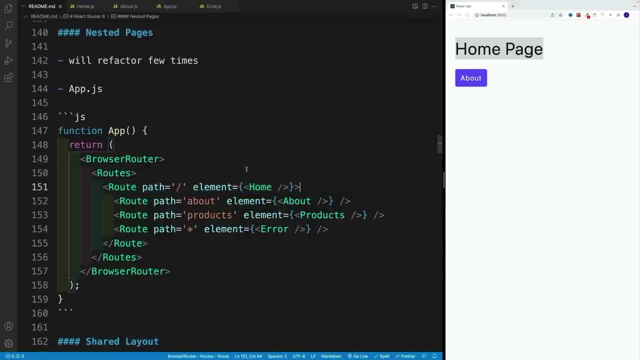 the parent route. So notice, instead of self closing the home one, I'm going to go with an opening tag and the closing tag And then I just decide which route I want to set up in here, And there's going to be multiple issues with our original setup. The main focus. 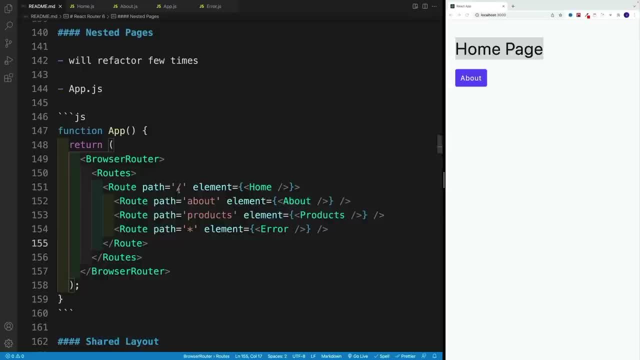 is that now all of these routes will be nested inside of the home one. Basically, they will be relative to whatever we have as a path to a home route. And don't worry, I'll show you also with another example, just so you can see better again. we'll refactor our application. 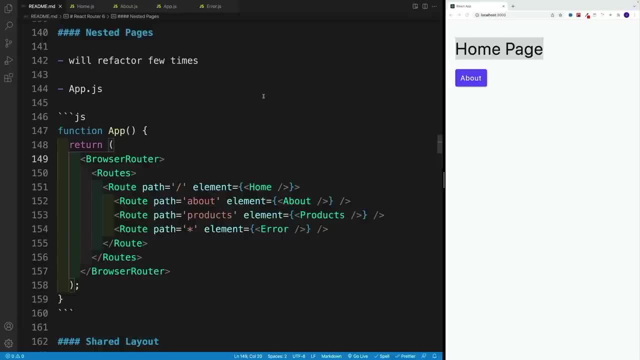 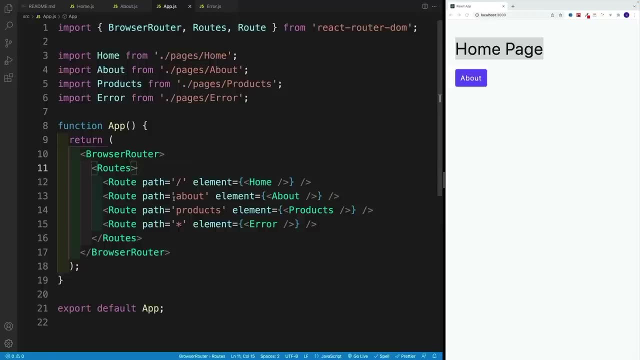 multiple times. So don't worry if in the beginning some stuff breaks. So let's navigate back to app js And, like I said, I want to nest about product and the arrow page inside of the home one, because I do want to set up a shared layout And I want to set up also a navbar. So let's. 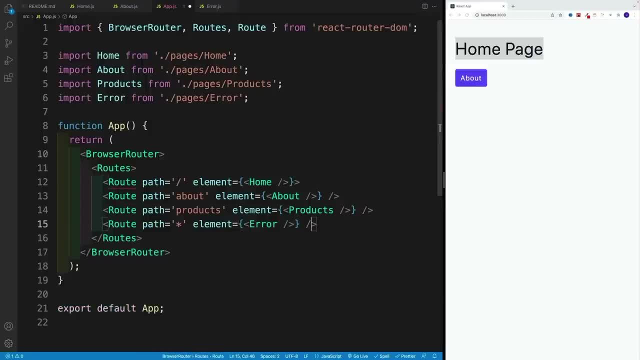 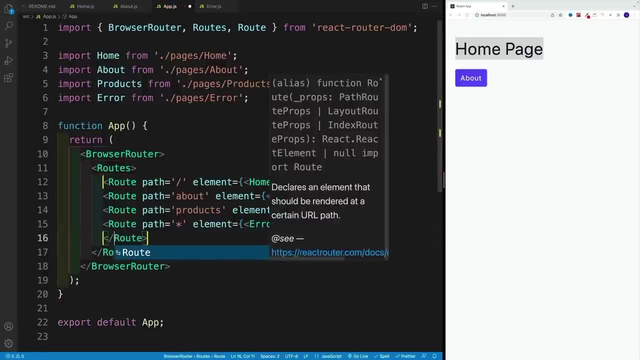 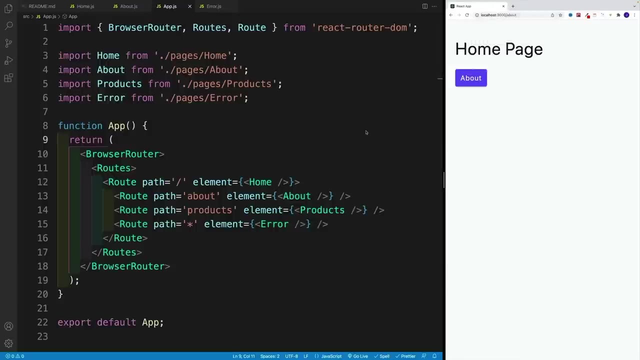 try this out where, instead of self closing, go here, let's say route, and then close it and, as I know, of course there's a syntax error like so, And, like I said, there's going to be multiple issues. If I go to about, I'll actually see the homepage And, yes, that is. 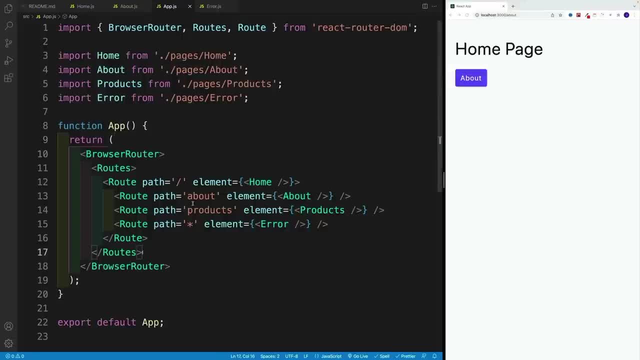 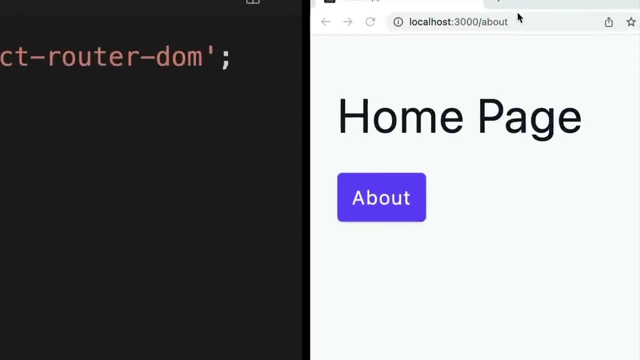 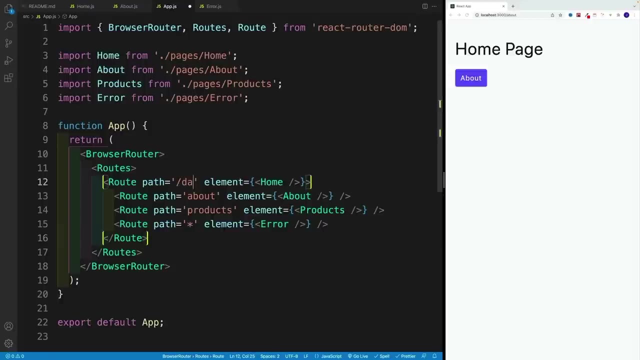 something we're going to fix in a few videos. Now, the main idea right now is the fact that these are all relative to the homepage And it's kind of hard to see, since this is homepage, since we're doing the setup on homepage. So therefore, let me showcase that, if I'm going 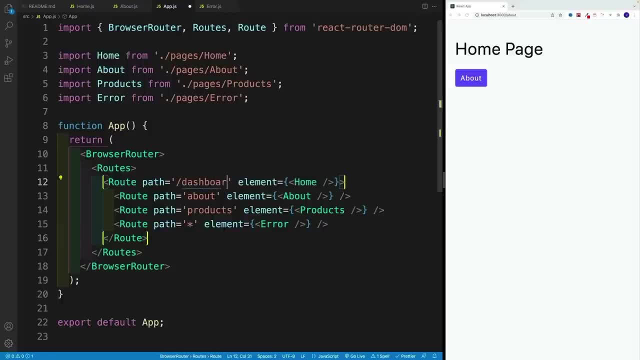 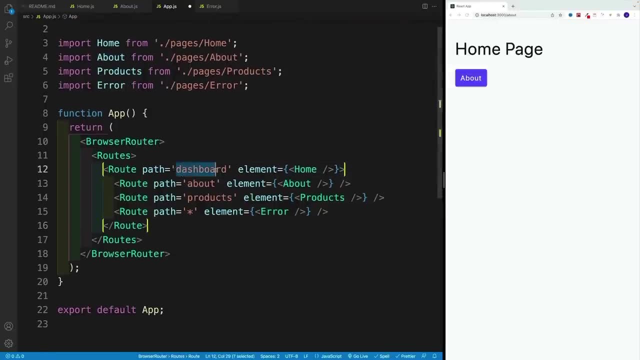 to go here with dashboard Instead. right now, you'll notice that you won't be able to navigate to an about page. you'll have to go to a dashboard forward slash about. So that's the key about nesting routes, where whatever you have here as a parent will be. 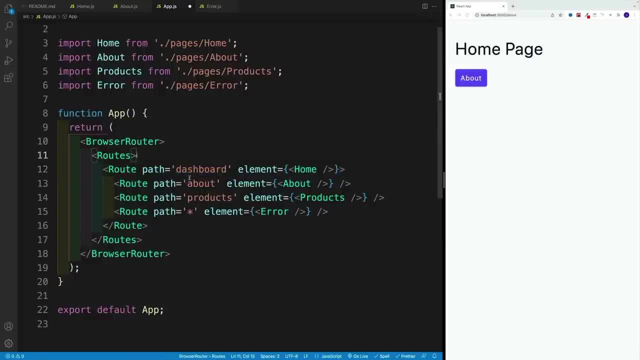 the main route And then whatever is inside is going to be forward slash on whatever path is over here. So let me save it. Notice I cannot see anything. But if I go to the dashboard and I'm going to go to the dashboard and I'm going to go, 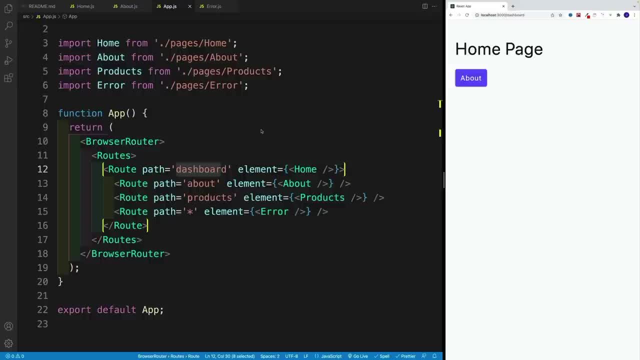 if we go to dashboard, which is technically our home run right now, and then about when everything technically works. Now we still don't display the about one, but we'll fix that in a second, So hopefully this is clear- where again, in our case, we're using as 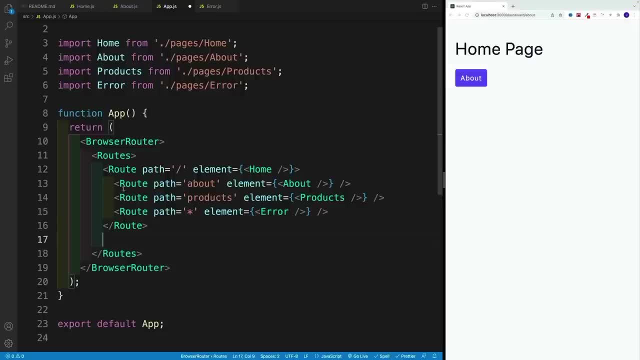 a parent, our home one, But, for example, if I'm going to go outside of this home one, if I'm just going to say, Okay, let me set up the dashboard, You'll see how basically this works. Again, you won't be able to see actually what is. 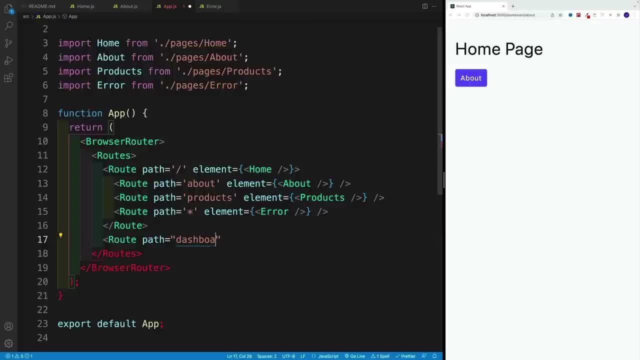 displayed in the stats, for example, the page that I'm about to set up, but you will be able to see that this is how it works. So, element, And then let me go quickly with Dave over here. I'll say dashboard show, And then we want to nest this. So let me go here with 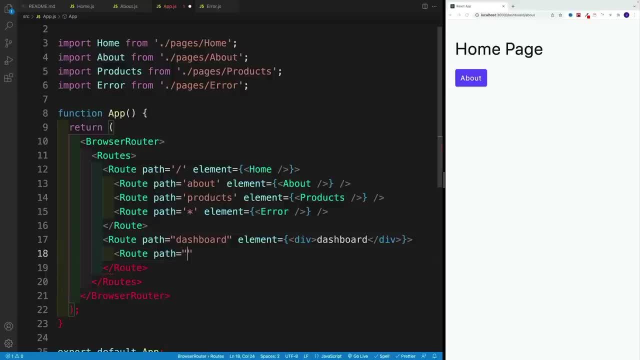 the route And then inside of it we'll set up path And then whatever path I want. So in my case I'm going to go with stats. So now we're looking for dashboard and then stats. So this is how normally will nest routes And again, 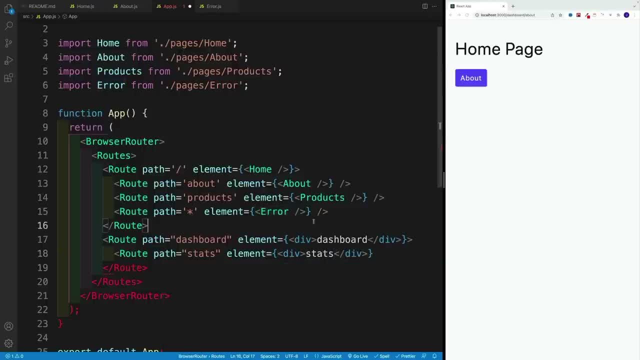 we won't be able to see this stat there Because we need to add a little bit more logic, which we'll do in the next video. this is just showcase. all this nesting is going to work, And if we're going to go to a dashboard and stats Now, you'll see that we'll have this dashboard one, but the 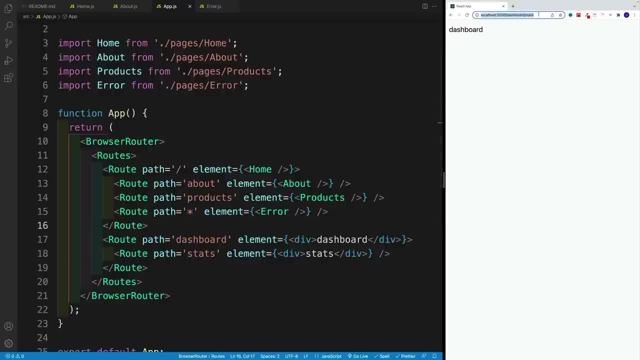 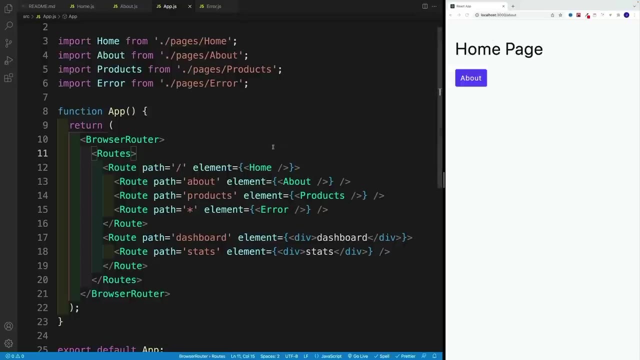 route exists, So technically there are no issues over there. Now, if I go to dashboard, this is what I'm displayed. And now if I go to about again, since our parent over here is the home route, that's why we see the about page Again. that's the first step how we can nest routes. 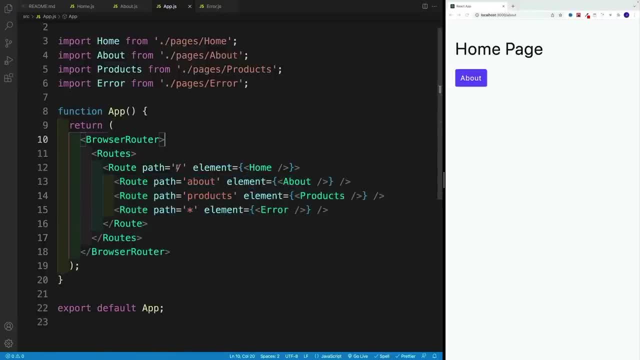 inside of the parent route And then whatever we have for a path is going to be the main path And whatever we set up over here is going to be the parent plus this value over here. So if you go here with dashboard, then it's going to be dashboard about dashboard product. And since 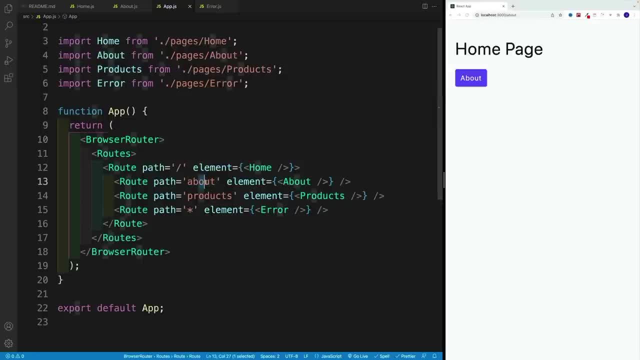 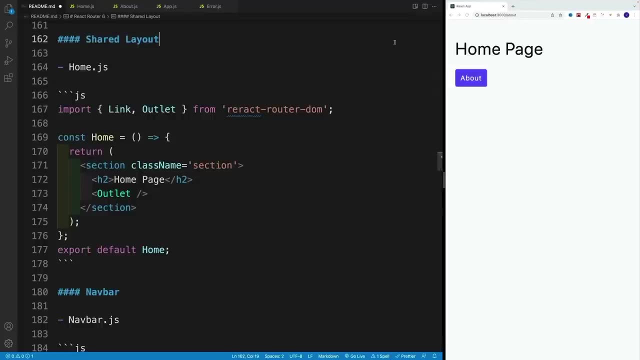 in our case it's a homepage we go with about and product, Okay. so our initial setup works somewhat all right, where URLs are matching Whatever we set up there with nested routes. But the problem is the result we keep seeing all the time: the homepage. So how we can fix that and how we can also. 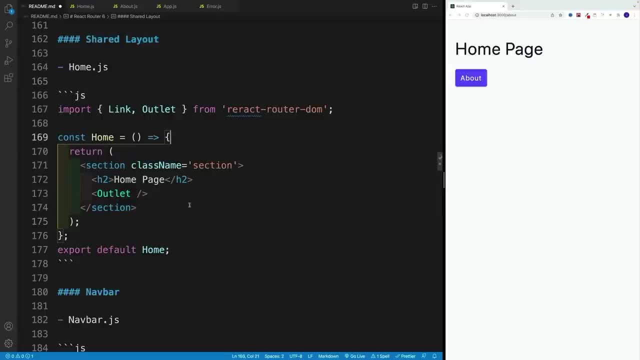 set up a shared layout. Well, we need to go to the parent- in our case home- and import, outlet the outlet component And then we just need to display this output component And whatever we'll set up around this outlet component is going to be the shared layout across. 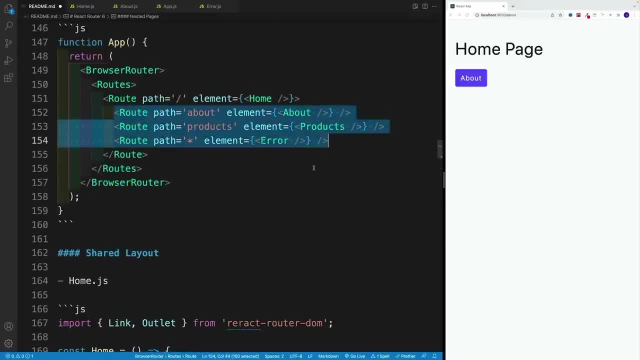 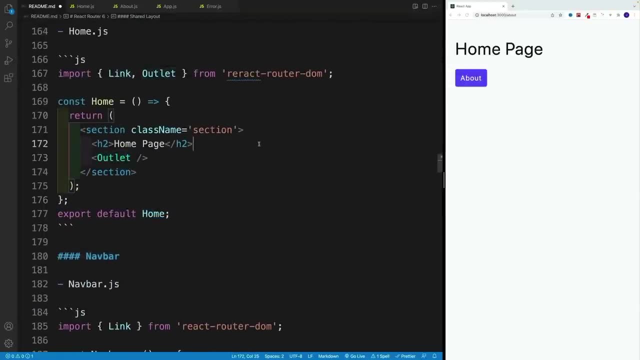 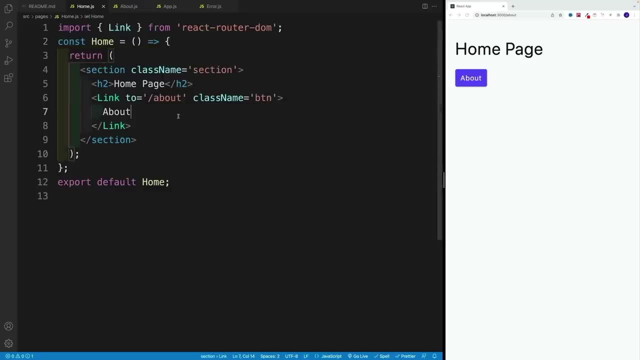 the pages that are nested inside of the parent, And then the actual page content will be displayed here in the output one. I think it's going to make a little bit more sense if we set it up, And that way you'll right away see what I'm talking about. So let me go to home address. we want to. 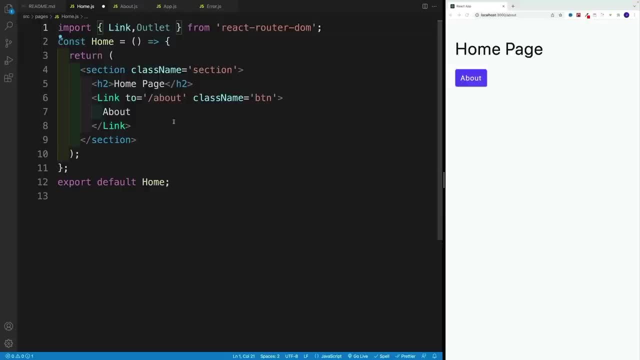 grab this outlet component And the position is really up to you Again. you'll see once we add navbar. But of course, however you set up this return, that is going to be how your shared layout is going to look like. Now I'm not going to keep this link. I think we're good to go, So I'm going. 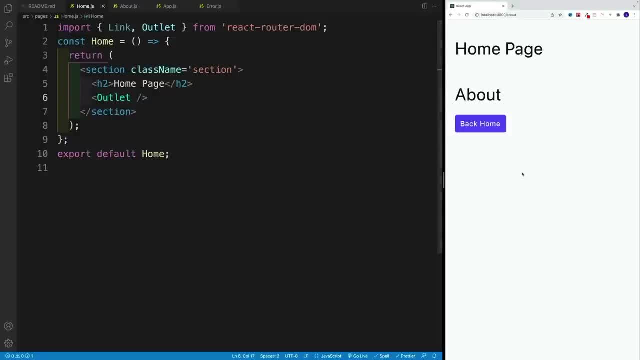 to go with outlet, And now, once I save, actually I see this homepage. So at the moment this will be shared all across the pages. But I nicely also see the About page And if I'm going to navigate to a product, same deal, I still see this homepage. So this one is shared all across. 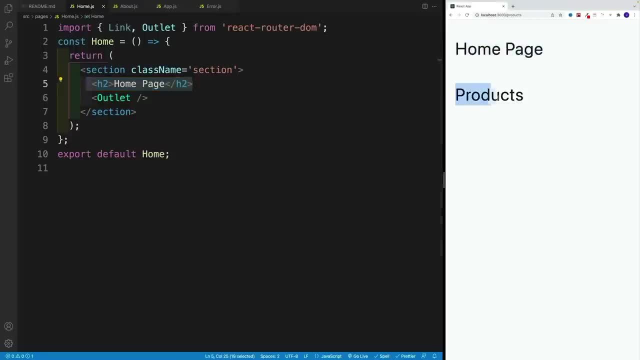 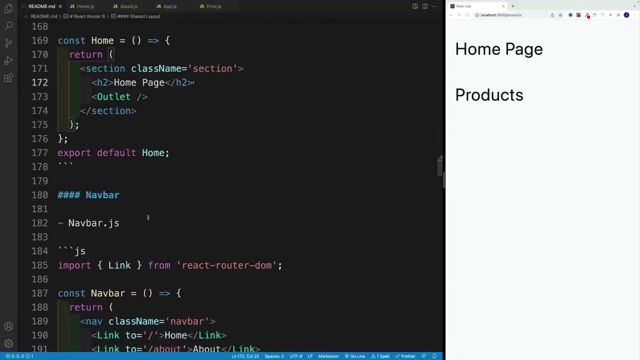 these nested pages And also I see the actual content from the product page, So now we can put two and two together. If this is shared all across the nested pages, why don't we set up the navbar and add some links And, as a result, 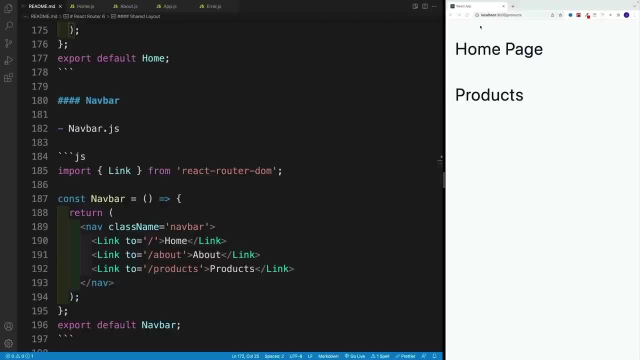 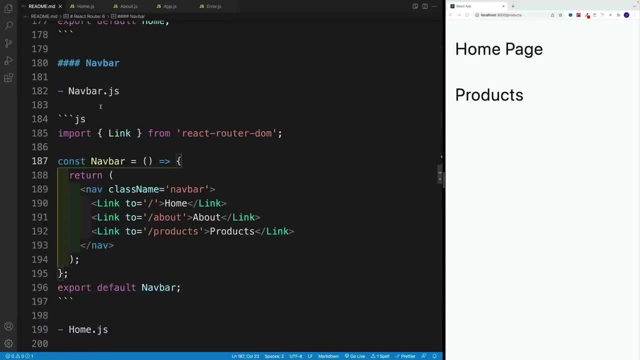 we'll be able to navigate from page to page, from home to about and to the product. Now, in order to set that up, we need to go with new components. So I'll set up the components folder And in there I'll create navbar j s And we want to import a link one, And then let's set up the. 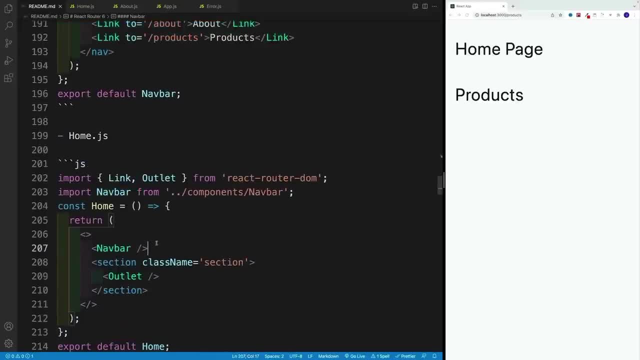 nav, Then let's add a link, And then let's add a link, And then let's add a link, And then let's import that in a home dress And again, whatever return you set up over here. that's how all those 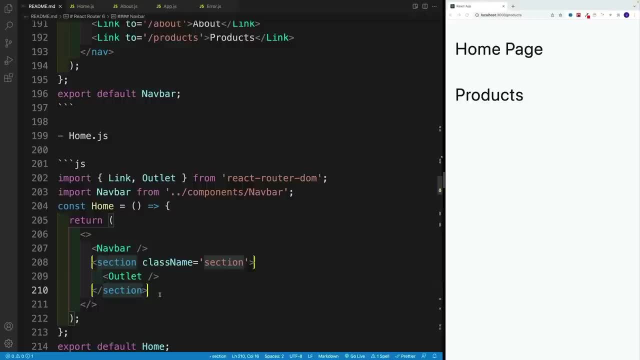 pages will be displayed. So if you do the side, let's say underneath the section, to set up a footer, you can definitely do so again, this is going to be that shared layout all across the pages And, don't worry, the homepage- the actual parent- is gonna look somewhat funky. We'll work. 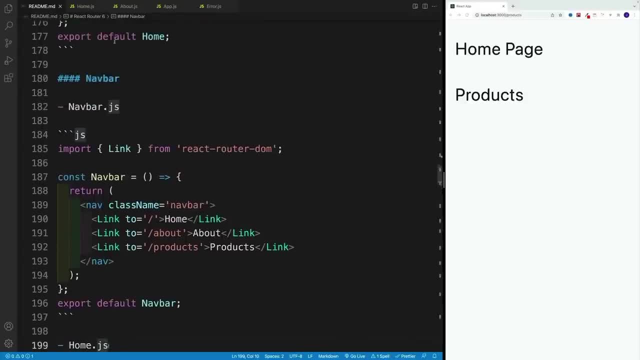 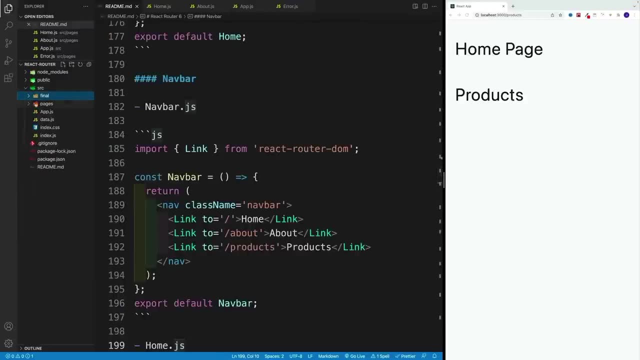 on that one next. So first let's worry about the navbar, And I want to do that by navigating here. please don't set this one up on the finals, Because it's already there. we have the components, So in the source. 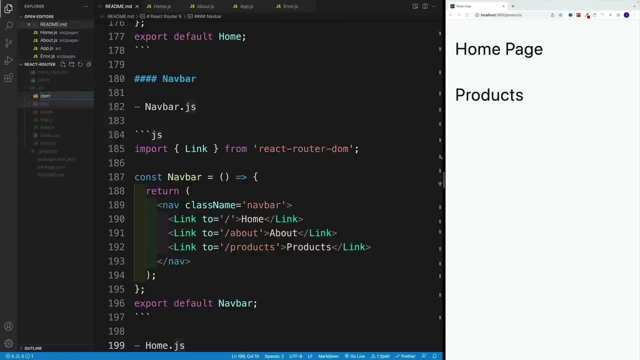 I want to create actually not a new file, I want to create a new folder component And this of course also showcases that. of course, like I said, in all of the components in the pages we can use other components because they're just good. all the regular components. I'll set up navbar. 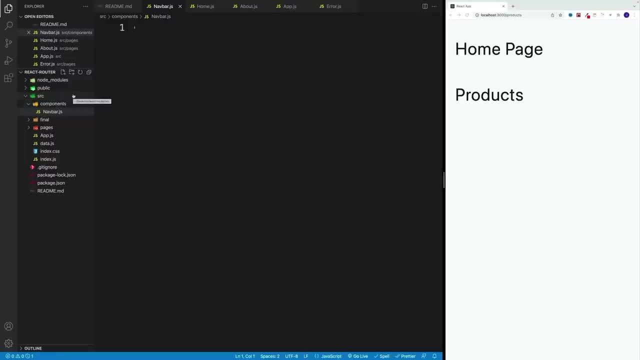 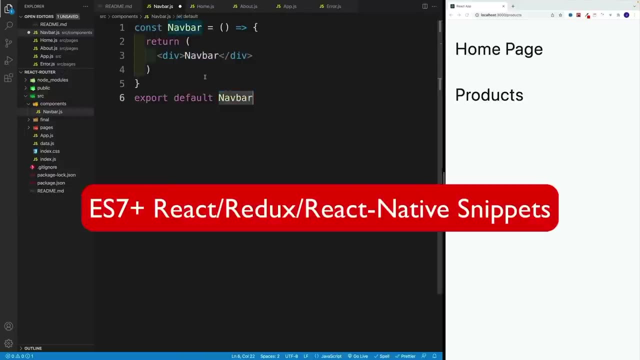 j s. Now there's going to be one more file, because I'll show you the active link as well, But let's not worry about it. right now I'm using this extension to create my component. this is going to be navbar. Like I said, I do want to get the link, So let me close. 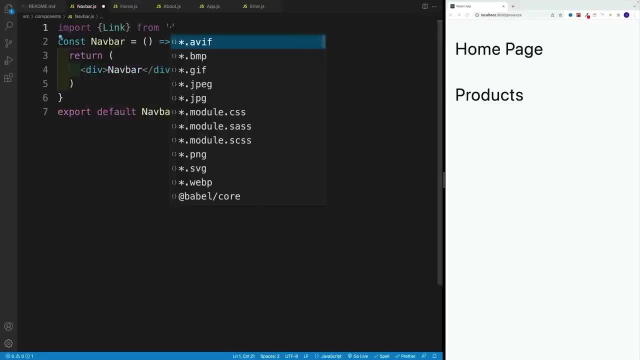 the sidebar. here I'll say link from, and then looking for react router DOM. And then we want to go with a nav. Now I did add a little bit of styling in the CSS. That's why I'll add here class name navbar. And then we just want to set up the links. Now I will set up links. 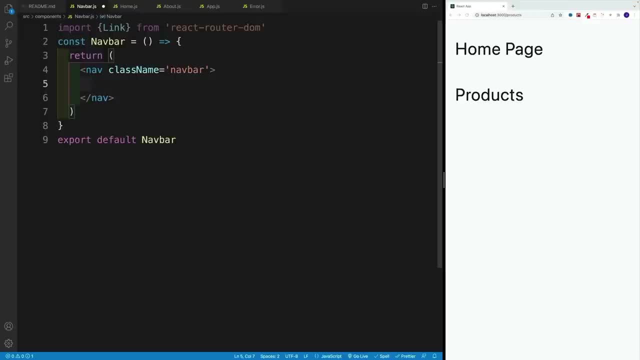 for about product and homepage, but we might add one more for login, one a little bit later. So let's go here with link to this is going to be to the homepage, And then let's add a text, let's copy and paste. Now this one will be to about page again, whatever pages you have, So in 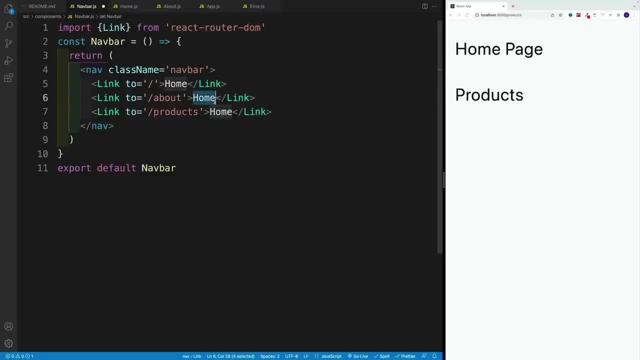 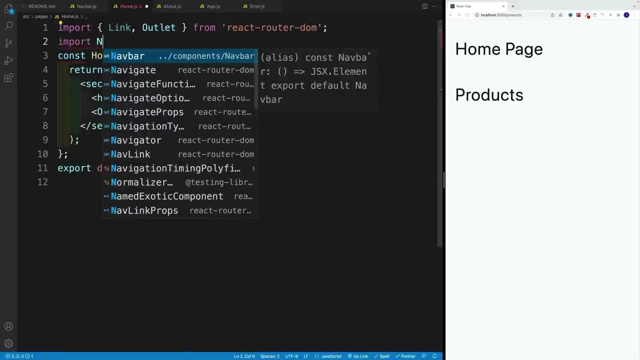 our case, we have about and product as well as the homepage Let's set up about. let's set up our product And now we want to navigate to the home one and import that navbar. So let's go with import navbar And basically you want to get the component. 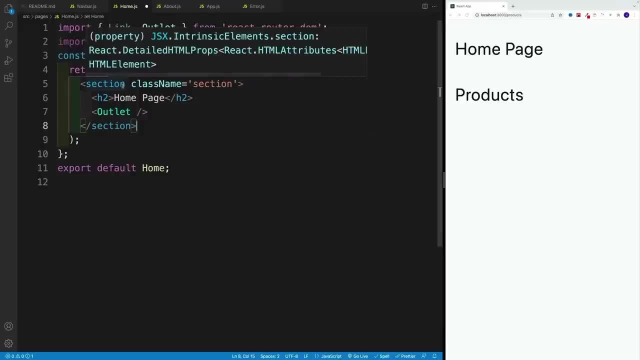 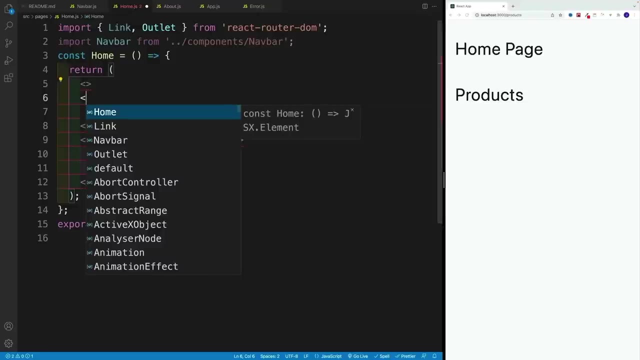 Like I keep saying, whatever structure we will set up over here is going to be the in the browser, So I don't want to keep this section right now as it is. instead, I'm going to go with react fragment, since we need to return one element. then I'll place a navbar on the top. 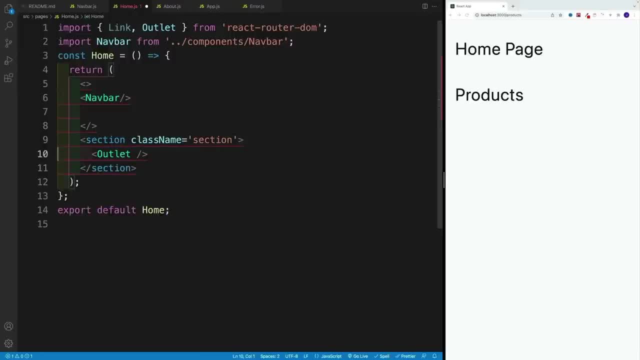 After that I will remove this homepage And then let me bring this section up. So I'll display the navbar like so with these links, And in here in the section I will have have that outlet, basically whatever we have inside of the page, So whatever we have in the. 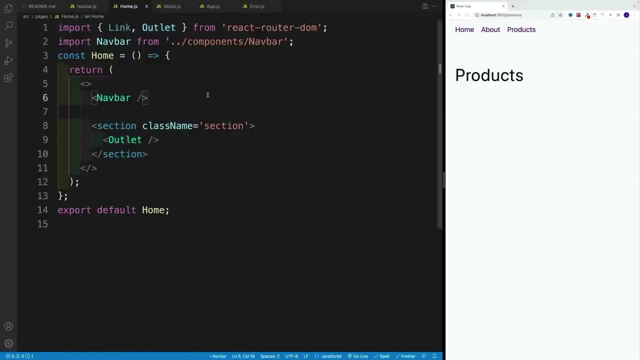 about in the product, essentially all the pages that we have nested And, as a result, notice not only I display the contents of the about page or the products page, but we also have the number. So if you want to add the footer, go ahead. Most likely you'll want to do that. 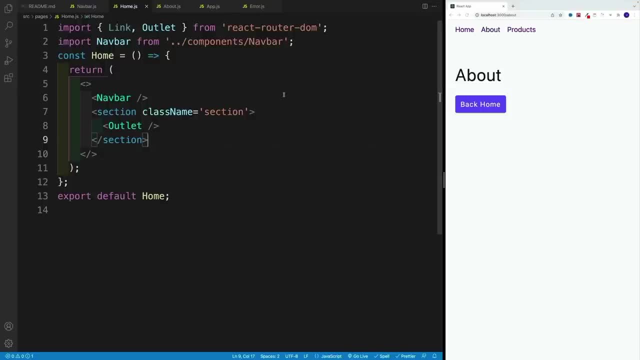 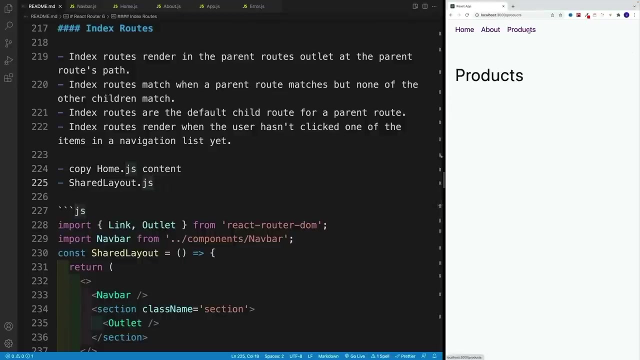 beneath the section. With this in place now we can set up the index page, because at the moment, if we navigate here, nothing is displayed, So let's fix that in next video. All right, so our functionality is almost complete. The only thing that's missing is the content in homepage. 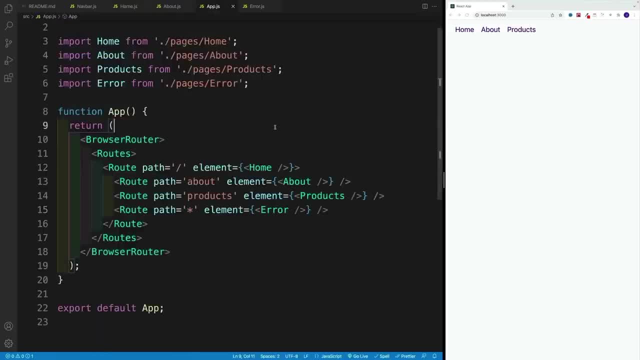 First, let's understand why that is happening. In the app js we have nicely nested the routes And for the parent we have the home. on inside of the home we have the outlet And there we display product about as well as the error page, something that I actually forgot to add. 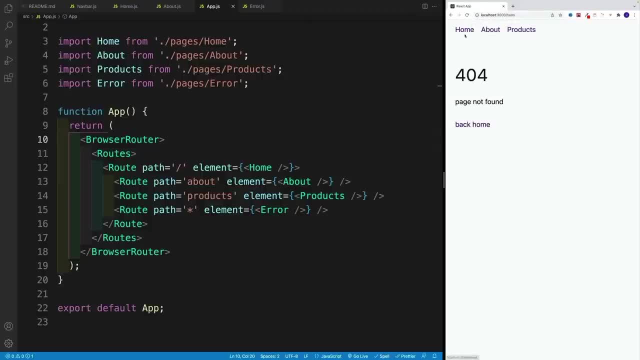 as video. So if I'm going to go with Hello notice again, will still have that nice layout, the shared one with an appbar and all that, And in here we display the content. But when it comes to actual homepage, well, we don't have any specific content here. That's why we 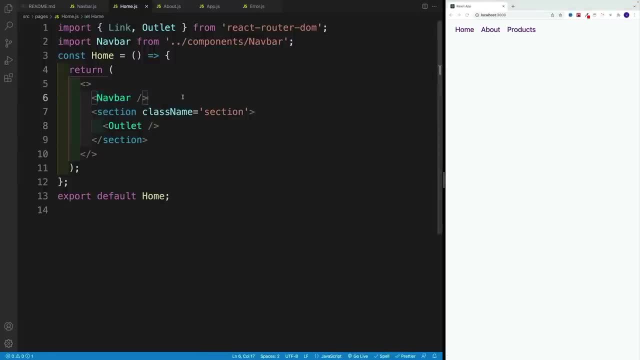 render pretty much nothing. So because, notice, here we have that Western home page, Here our page is pretty much nothing, we just have the number And technically, if you want, you can add that heading to or whatever content you want, But just keep in mind that that will be shared all across the. 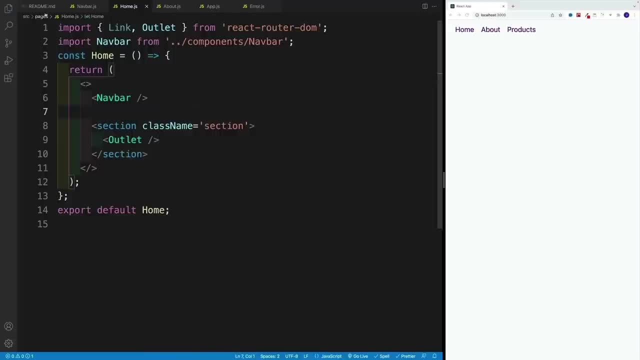 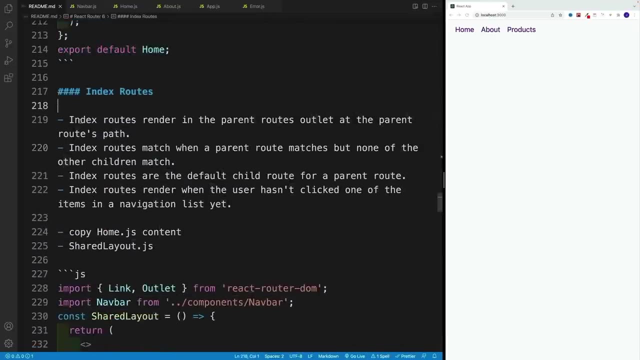 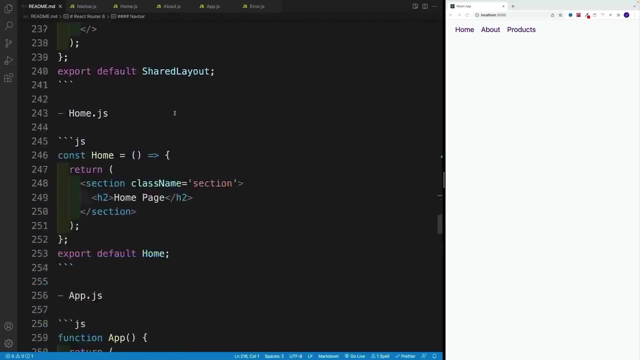 components, basically the pages we have nested. So what is the solution? Well, the solution is to set up index routes. And here I just added some text from the React router docs. you can definitely read it through, but I think it's going to be faster if I just showcase the syntax. So if we 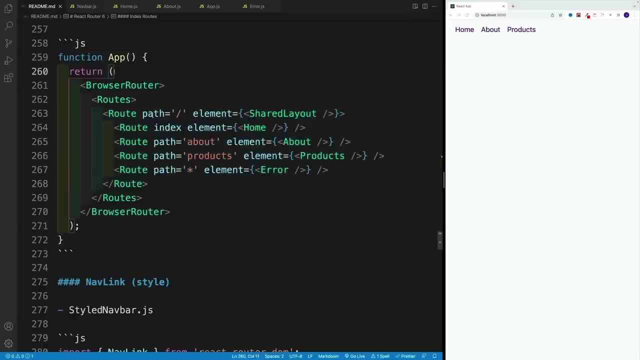 have these nested routes. for the main one, for the parent, we can set up the index road and it has a special syntax. where we go route, then we pass in the prop by the name of index And this will always, always, always match whatever we have here for the parent path. So if this is going to 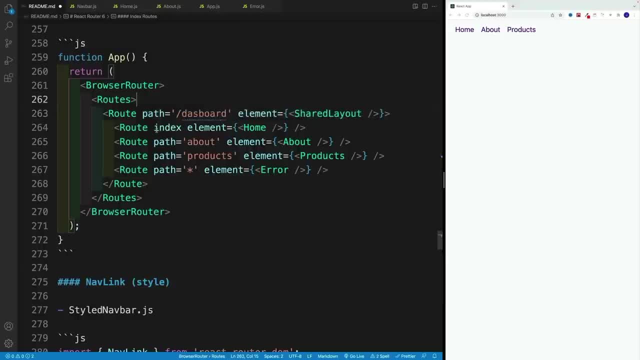 be dashboard, then yes, this index is going to match the dashboard. However, since in our case, we have home, we have home And then again the same deal, we go with element. Now, the gotcha here is that we still want to set up some kind of shared layout. 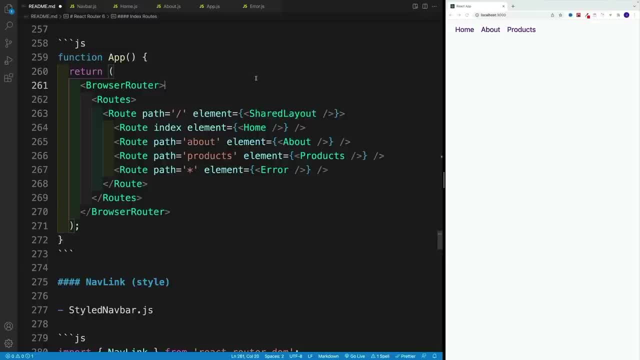 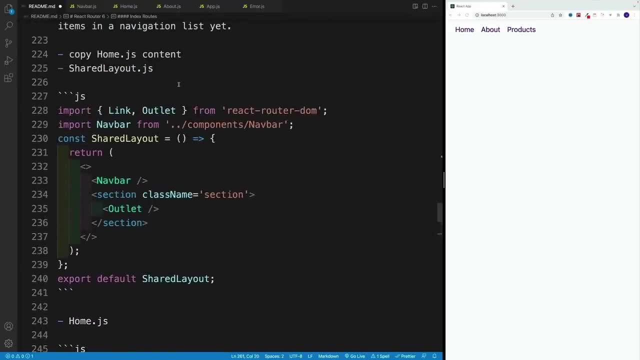 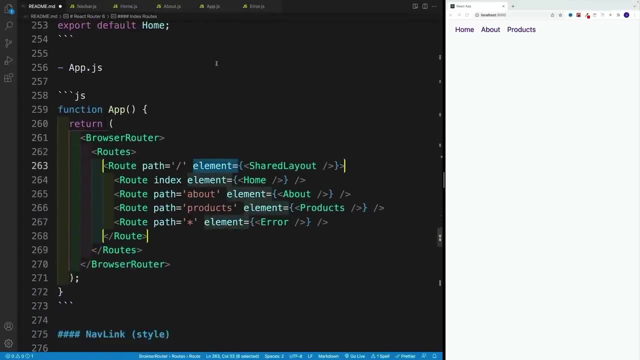 correct And therefore we'll have to create a new component And in that new component we'll basically take whatever we have right now in the home one And we'll add that one as a shared layout in here as an element. So whatever we have right now in the 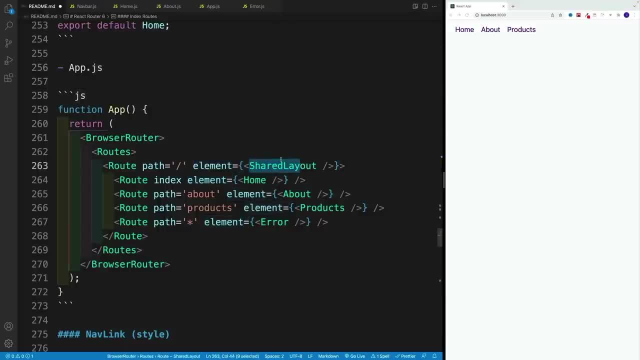 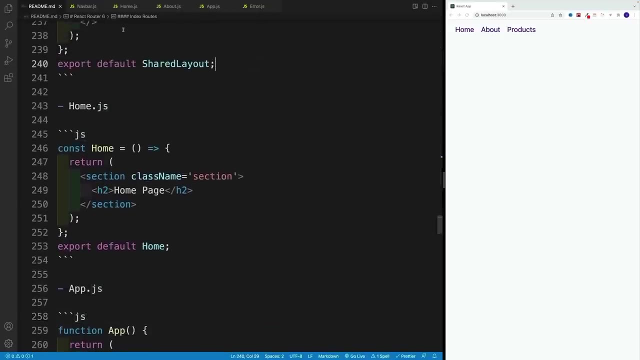 home. we'll create a new component. we'll call this shared layout. So now, always share this layout all across these pages, but then the home one will have its own content. Hopefully this makes sense. So now let me save this. Let me first go to a pages, then we want to create a new one. 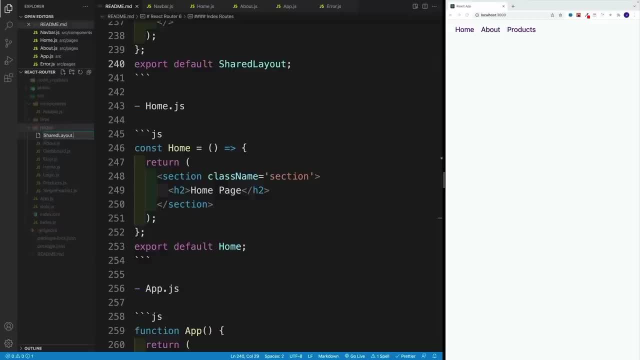 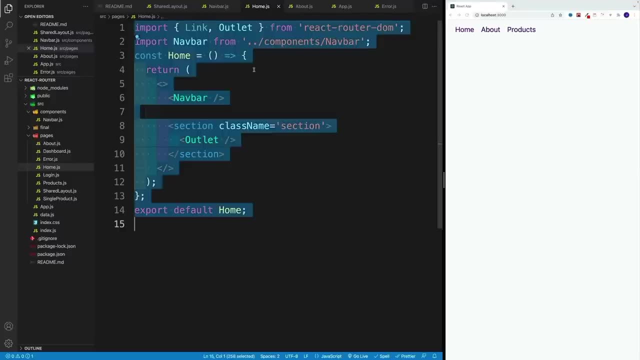 I'm going to call this shared layout. So as you can call this, shake and bake, doesn't really matter. Let's grab the home one. And you know also, as we'll be setting this up, we're gonna remove that section, because each of them have already that section with a class name. 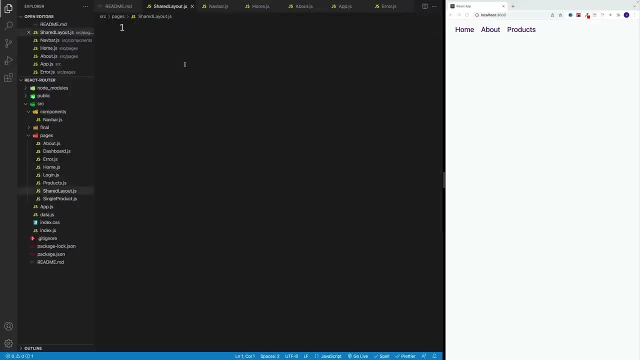 of section. So that is an overkill. So let me navigate to share layout: copy and paste. Now let me remove this section, we don't need it. So now we have only two things. We have layout, which will have the page content, whatever is the page: the homepage, the about page, 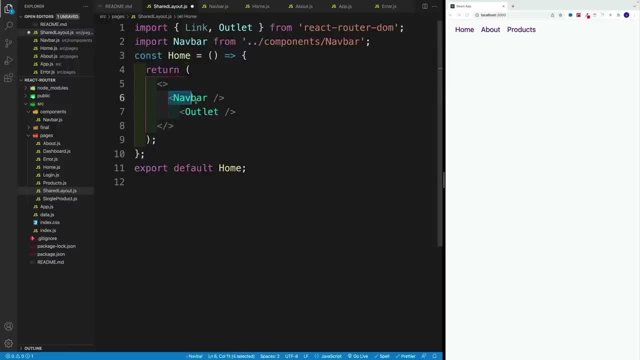 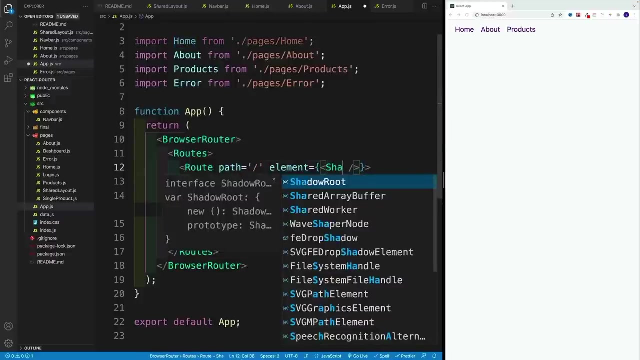 the product page and also whatever we want to put around it. So in my case that is just a number, And once we have this one in place, let's navigate to app js. we want to set up that shared layout first. So let's say here: shared layout, Yep, push, it breaks. 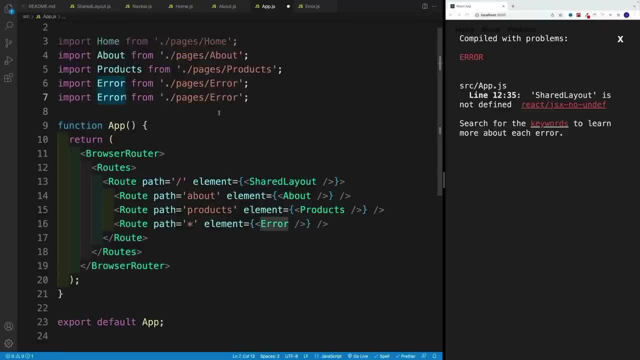 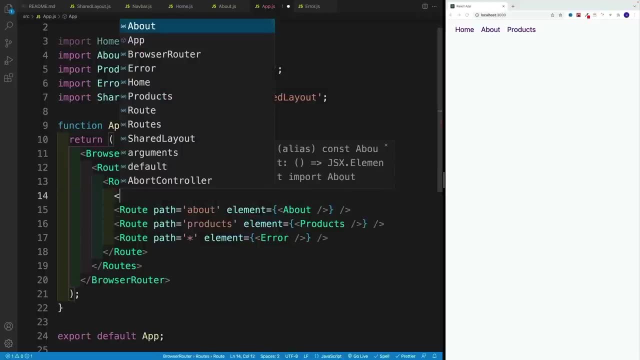 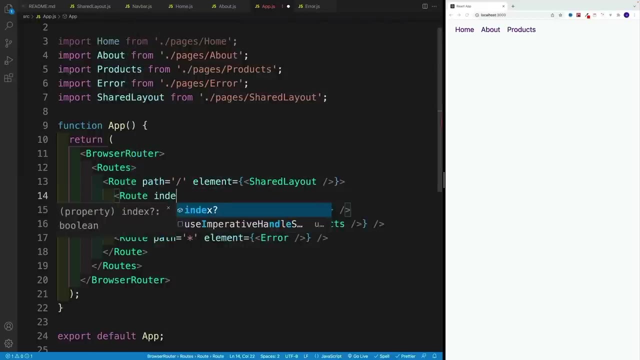 So let me copy and paste. I'll say here: shared layout And now we just need to work on that index page. So if we want to set up a page that will match the parent in this nested URL structure, we go route, then index and then we pass in the element. So in this case you want to go with home. 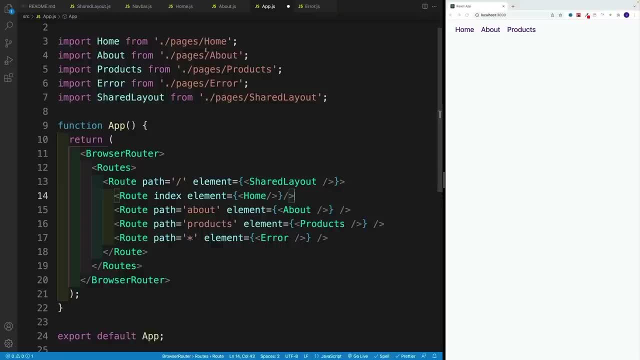 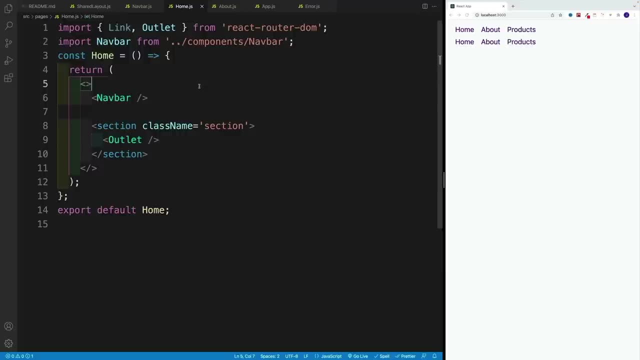 And now we need to navigate And first of all we need to close it here When we want to navigate to the home one. And since the moment I'm displaying the navbar, we want to remove some stuff where I think I'll remove both the Lincoln outlet. I don't think we'll need it, since we already have the navbar. 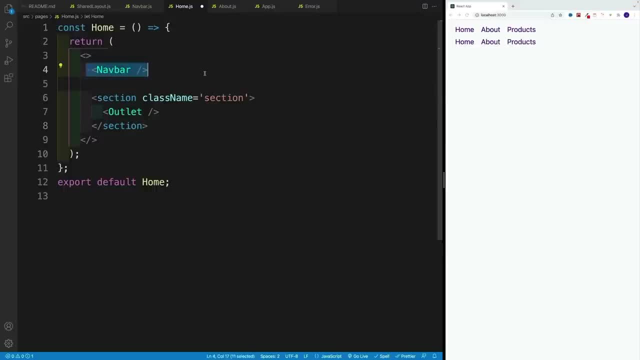 anyway, And then we just need to come up with whatever we want to render. So I don't want the outlet, I don't want a navbar, just want to go with my good old heading to, and I'll say homepage. And yes, we can also remove the second, like I said. yes, I purposely did this the long way. 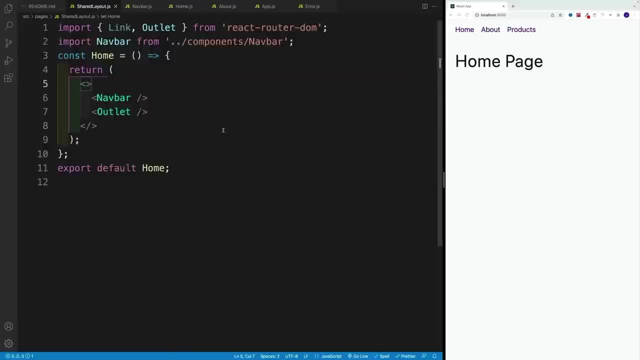 Kind of showcase how we get to that shared layout and what issues we're gonna get along the way. So yes, there was a little bit of refactoring. The good news is that checkout through our result we have homepage which displays home on about van products And then 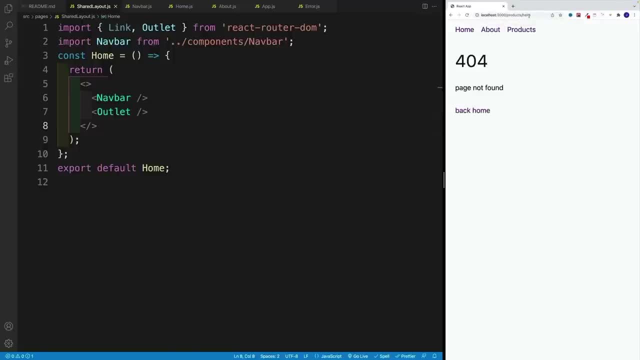 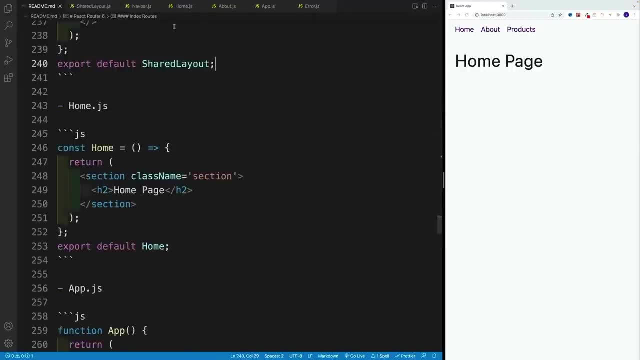 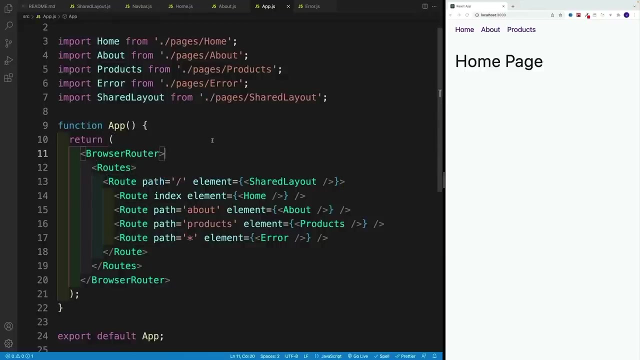 if we have some kind of page that doesn't exist, let's say products and Hello, when we display homepage and we nicely navigate back. So hopefully this is clear Where, if we want to set up this shared layout First we need to come up with a parent, in our case that. 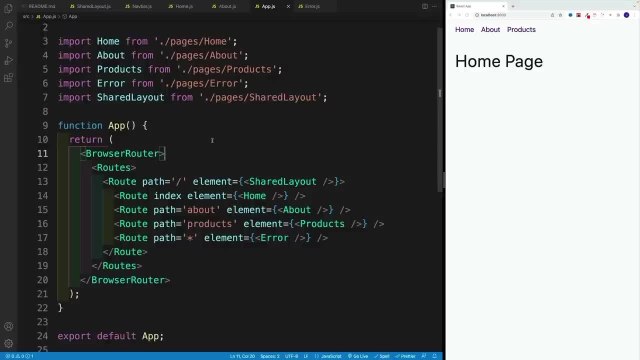 is index. But again, I showed you example with dashboard. whatever you type over here that's going to be the parent. then most likely you'll come up with some kind of shared layout, So what you want to share across those pages. And as far as the parent, you'll set up the index So that 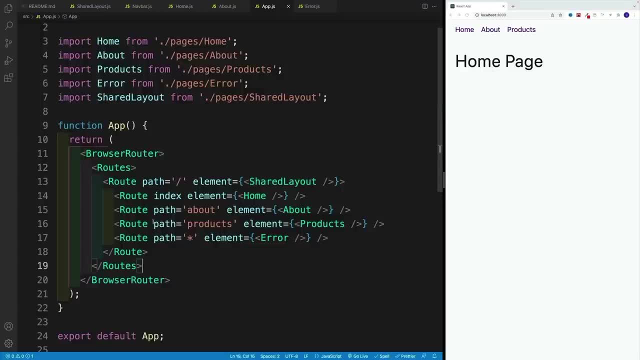 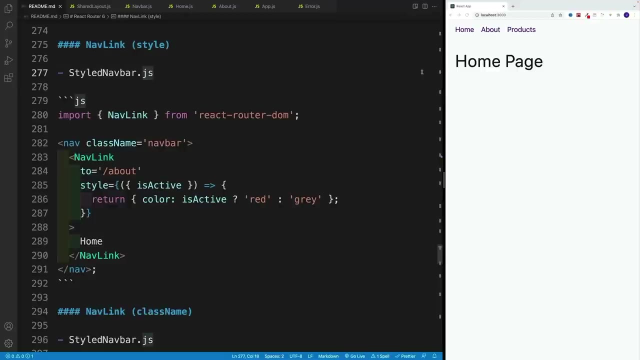 will be the content: only 40 actual index and then the rest of the pages. And remember, we need to use outlet to render those results. All right, And before we start working with URL parameters, let's also see how we can set up active links, And effectively. what that means is that 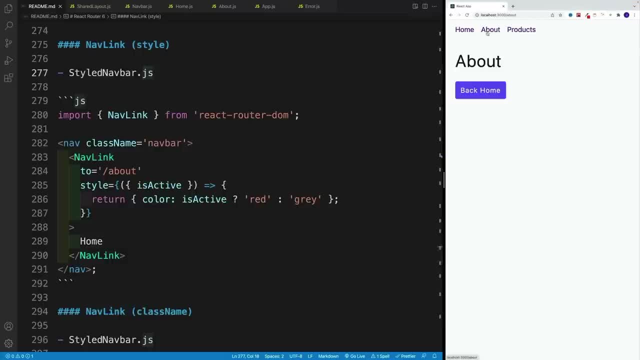 once we're on the page, this link will have specific styling, whatever we want to set up, And in order to do that, I will create a new file, just so. let's set up space for your reference And instead of link, we want to grab the nav link. Now what's? 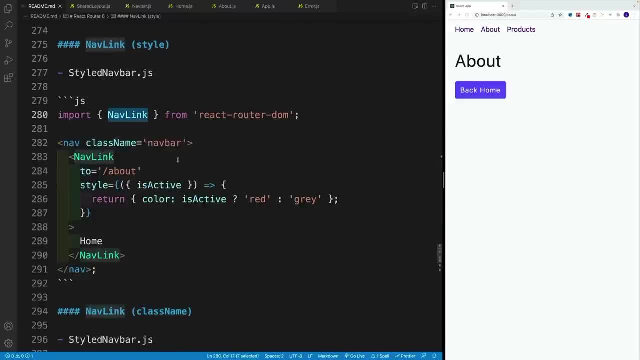 special about the nav link is the fact that in style and also in the class name we can pass in the function where there's a property better now is active Again. this is provided right away by react router And then based on that value. 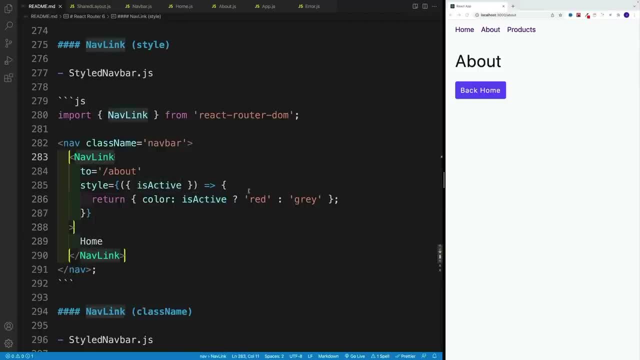 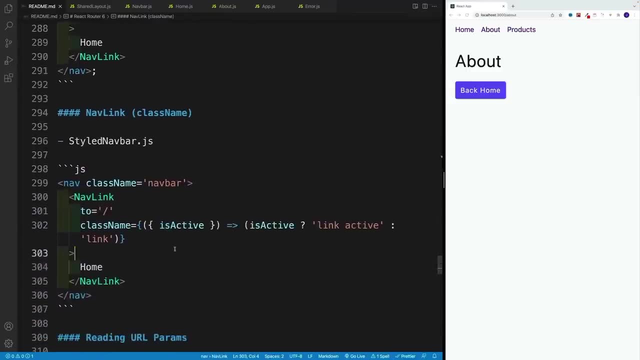 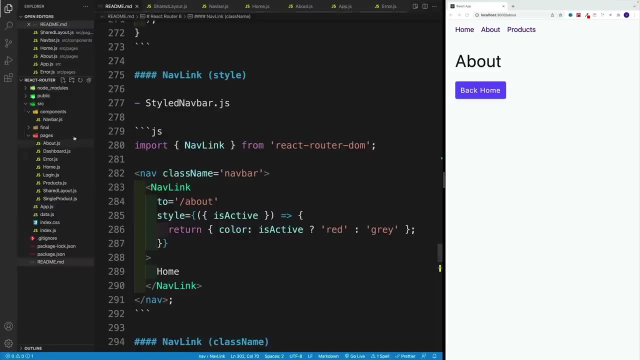 we can set up some type of styling. Again, this is the straight up inline CSS approach, But we can also do that with classes And of course, we'll take a look at both examples. Let's start working on the main setup first, where, in the components, let's create styled navbar. 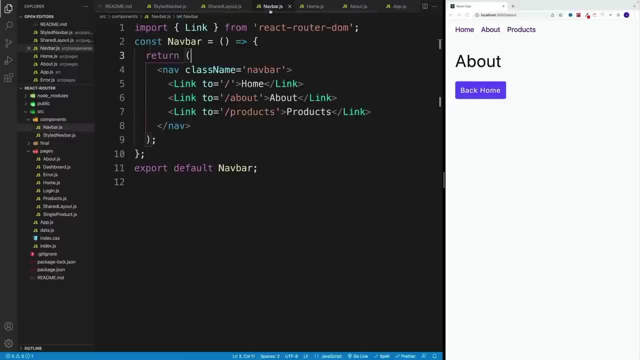 And again, the reason why I'm setting up a separate file is just so you have right away a reference for the basic setup And if you'll notice in the components we can set up a separate file for the basic setup. Let's copy and paste Again. we're looking for nav link instead. 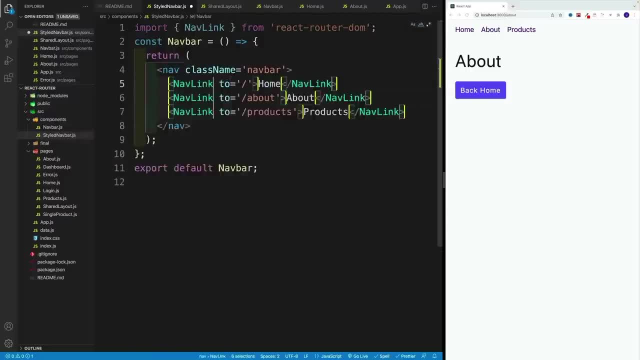 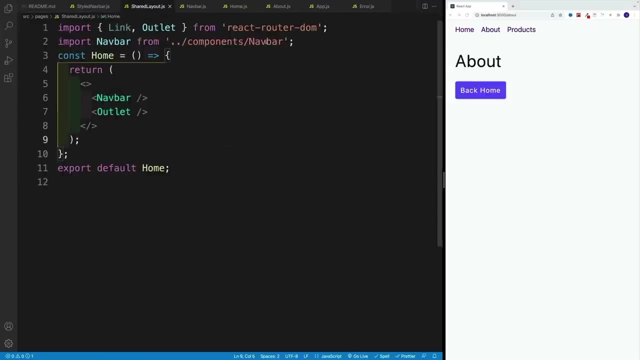 Let's change the suckers as well. We're looking for nav link For now. let's not do anything, Let's not add any kind of logic. We simply want to navigate to bubba, bubba, bubba up, Jess, Or, I'm sorry. what app is shared layout? my bad, And I'll copy and paste. I'll just say: 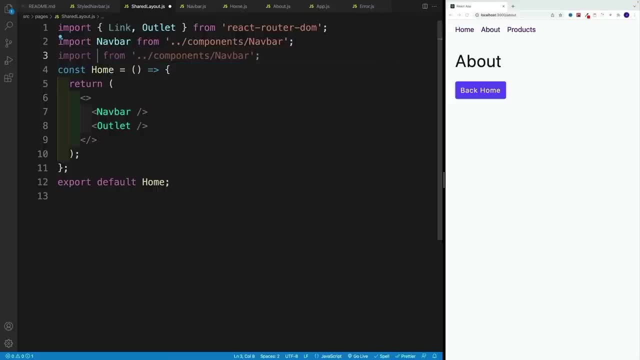 shared layout. shared or, I'm sorry, not shared layout. For some reason I'm totally tripping here. So styled and navbar. of course, my apologies, And for some reason I didn't change this one as well. Instead of typical navbar, let's go here with a styled navbar. 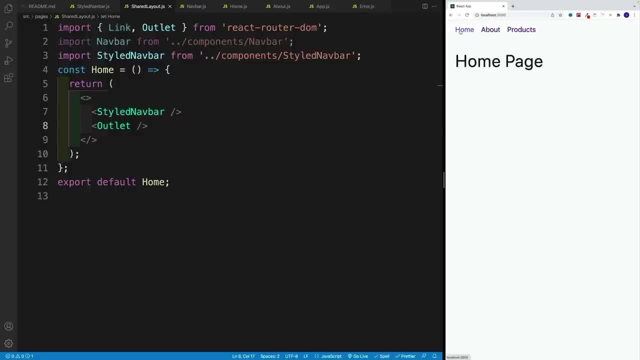 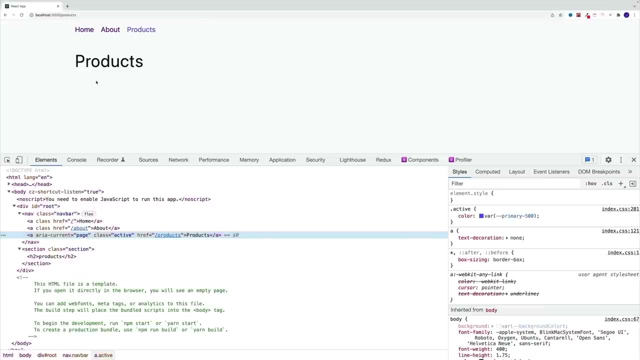 And once we save, we right away notice that our active link gets different styling. And first let's just quickly cover why is that happening, And second we'll take a look at the code that controls that. So first, why is that happening? Well, again, by default, if we use that nav link, the react: 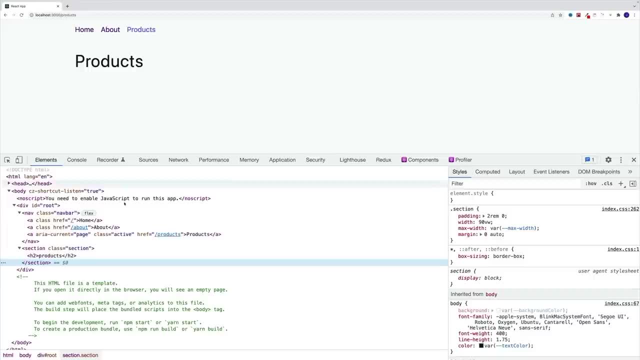 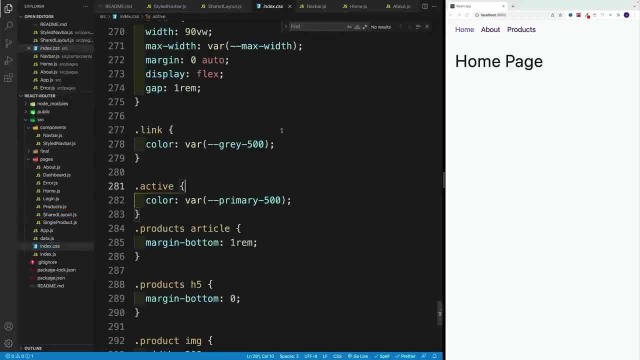 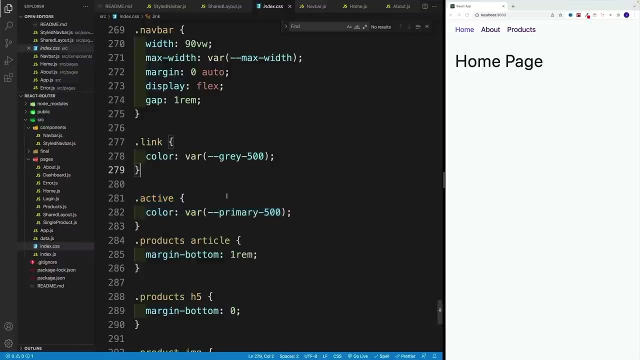 router by default, even without us doing anything, adds this class of active to it. And if you take a look at index CSS and, more specifically, if you just keep on scrolling somewhere on the navbar, you'll find this active class. So if you just set up an active class, if you use nav link, the class will be automatically. 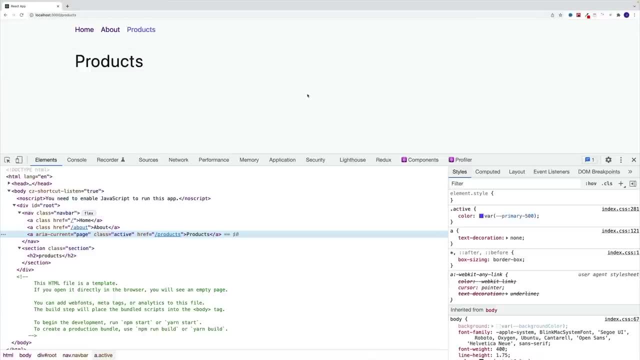 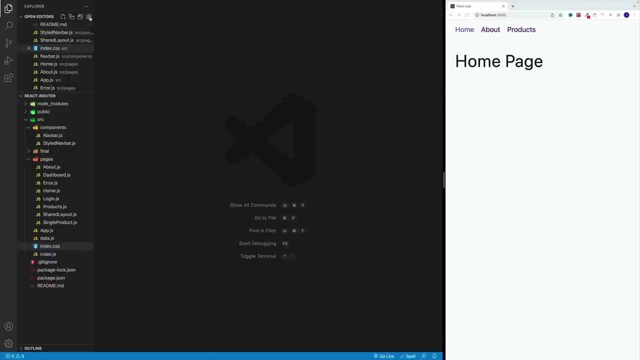 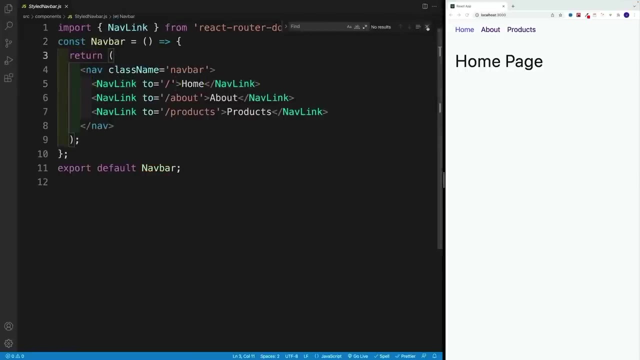 added And, as a result, you'll get the styles. So now let's see how we can control that code a little bit more. First of all, let me close all my files and all that here, So let me start from scratch. I think it's getting quite busy. Let's just take a look. Now we can add. 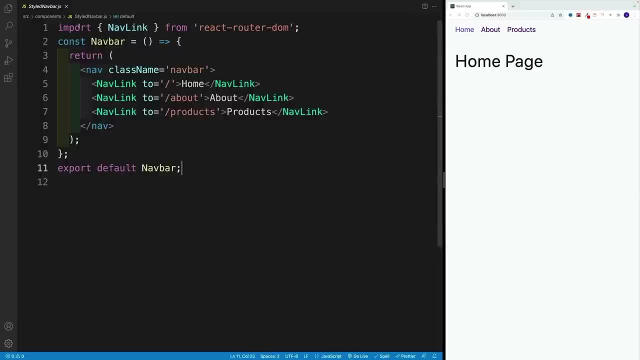 good old regular CSS to it. So I'm in the user interface. I'm going to add a new user interface. I'm going to add a new style navbar. Then we want to go with style over here And I'm not going to add to all of them, But I will showcase for the home one. So I'm going. 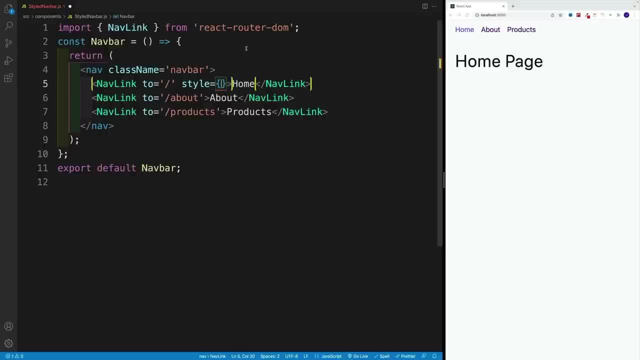 to go with style, I want to go with interpolation And, like I said, we want to pass here the function Again. this function, the value and all that is provided by react router down. Now, keep in mind, this is not just good old parameter here, So don't say: is active we? 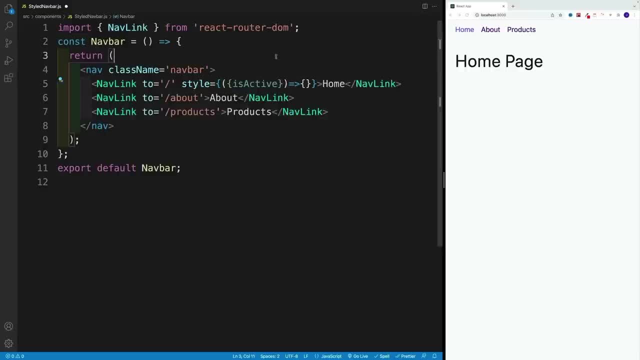 need to specifically look for object and then is active. That's how we can properly access that. And then, since we're setting up here inline styles, we can just use a ternary operator where we go with a return. So, whatever we return, 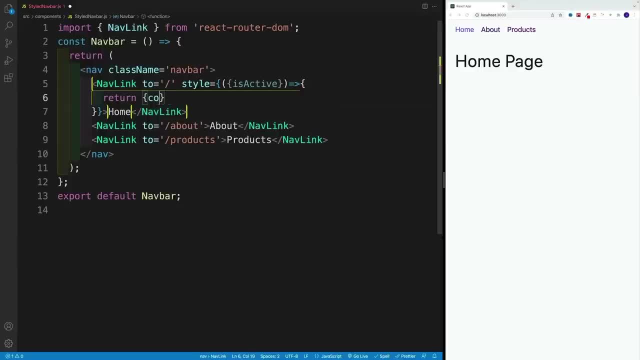 in this object will be applied to this link. And, more specifically, I want to look for the color And then I want to check: is active? So what is the value? So if it is true, I want to add color red, And if it's not, then I want to go with gray. Please check that. 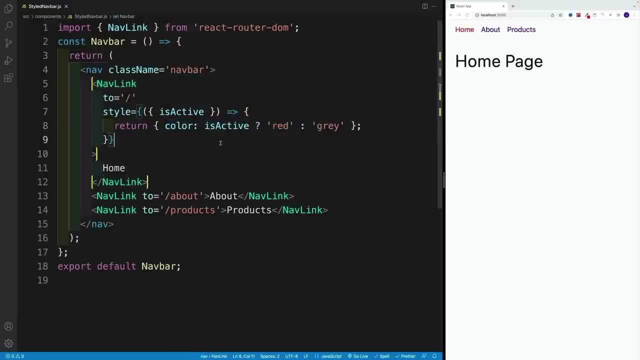 in mind that we can set up whatever functionality you want over here. I'm just going for straight up color. Of course, if you prefer setting up your CSS inline, you can add whatever the properties with values you want, And I'll check it out If we navigate to our page. 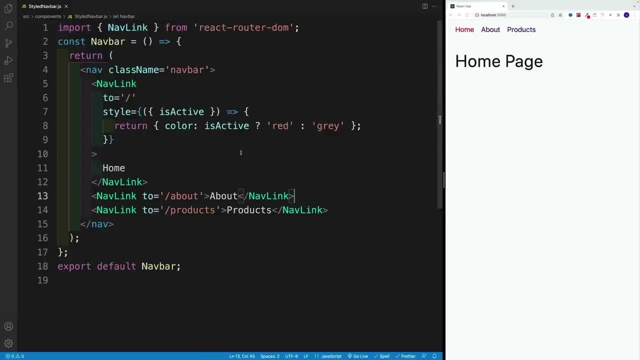 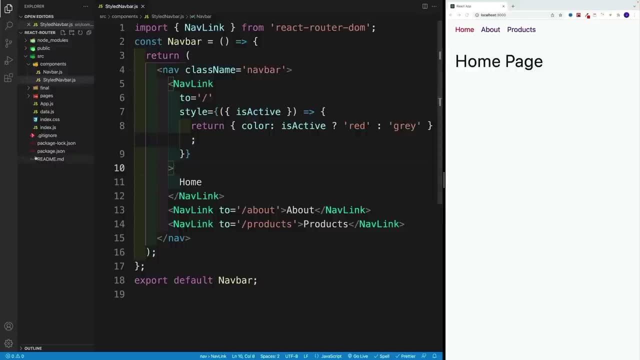 the style will be red, So the color of the link was going to be red. And yes, if we add this to the rest of links, it's also going to work. I already set up the reference for you over here, So in my case, in the style nine bar, I'll just showcase the class approach, since in 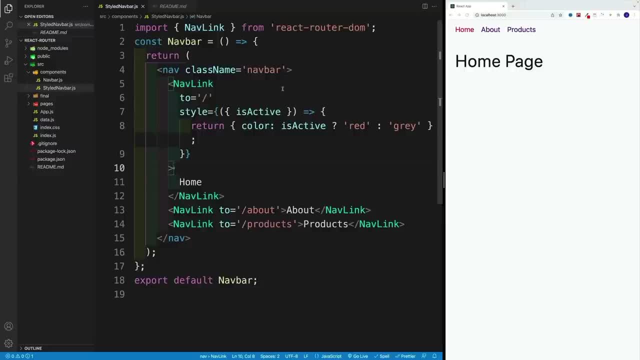 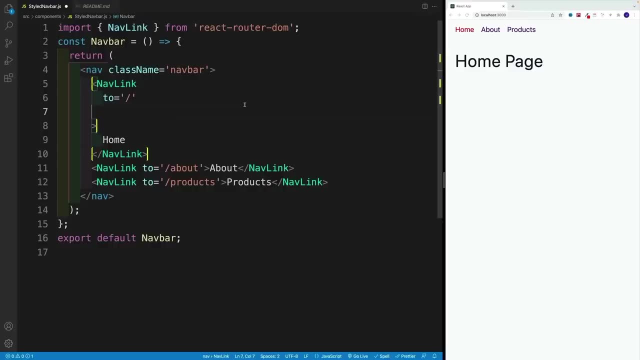 my opinion, that's probably is going to be something you will use more often. So if you ever need this reference, it's available in the readme. So let me remove this style here And now. instead of style, I'm going to go with class name. And if we take a look at 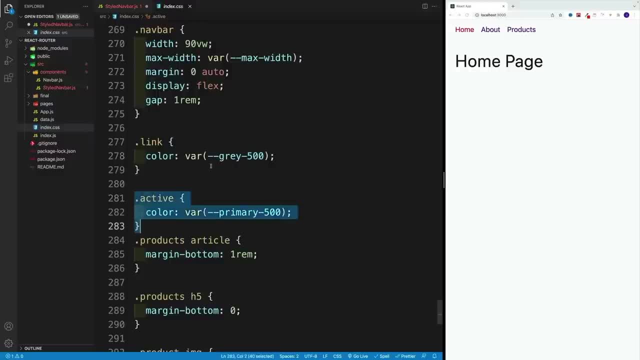 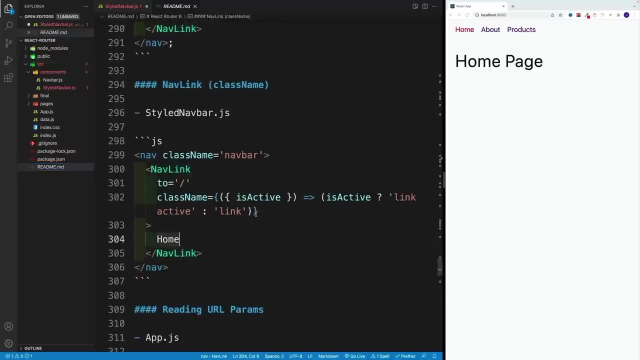 the CSS, you'll notice that not only I have the active one, I also have some general style for the link. And yes, of course, like I keep repeating, you would normally add more code over here. So instead of just relying on the active one, I'll say: Alright, what is the value for is? 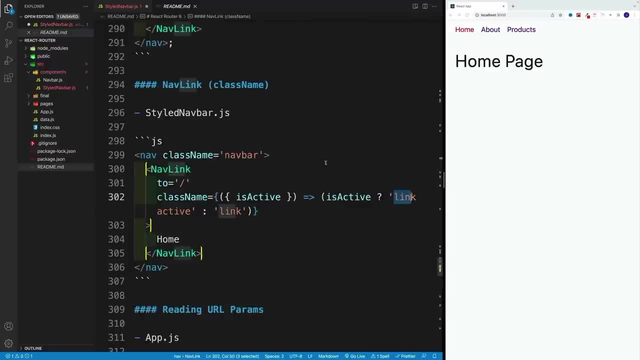 active. If it's true, then I want to add link class as well as the active one. Basically, this is where I'll have more styles normally, And if it's not, then just going to be Link class which just gives the link. 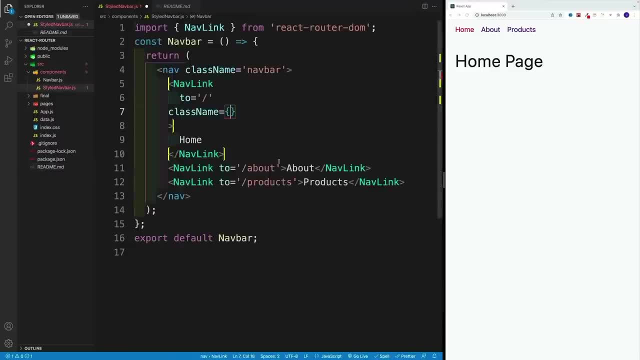 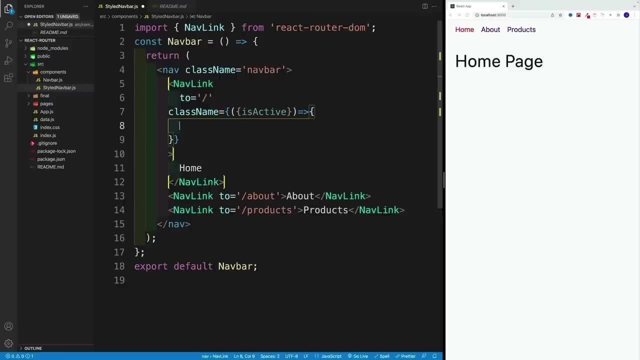 up that ternary operator where we want to go with is active, And you know what I think. in this case I'm just going to go with implicit return. So is active? if it's the case, then I'm going to go with link and active, And if it's not, then I'm just going to go with. 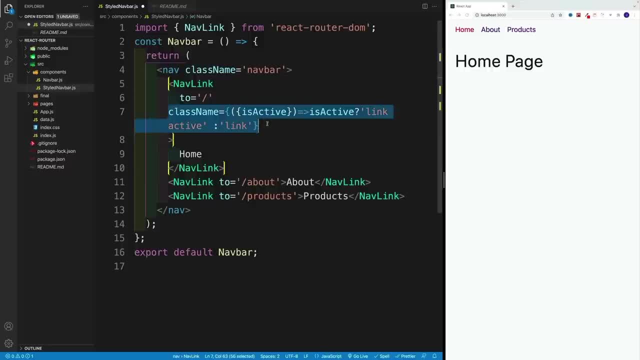 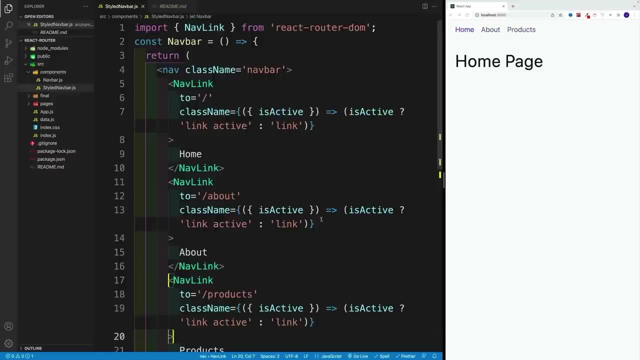 link one. I do want to grab this entire thing, So copy: hopefully there are no bugs there, And then we'll just set up on all of these ones, But save. this is going to be our default setup And then once we click now, of course we get that active class as well, And as you. 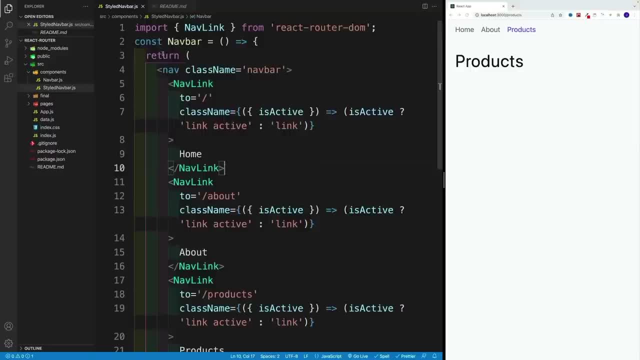 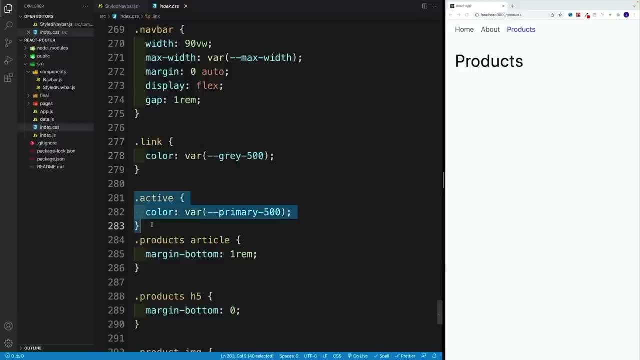 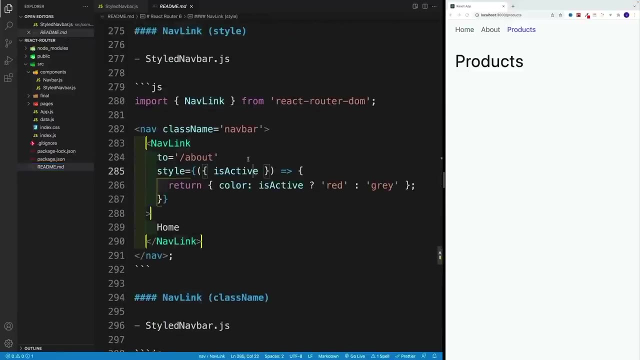 saw, there's multiple ways how we can set up. If you just have the active class, it will be added by default to that nav link. So technically you don't need to do anything, But most likely you will set up the class approach. Also, keep in mind that of course you do have this. 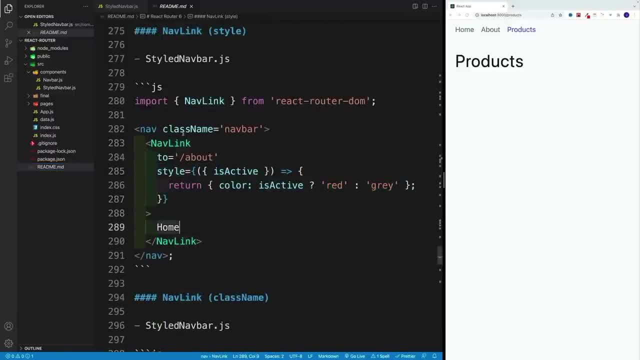 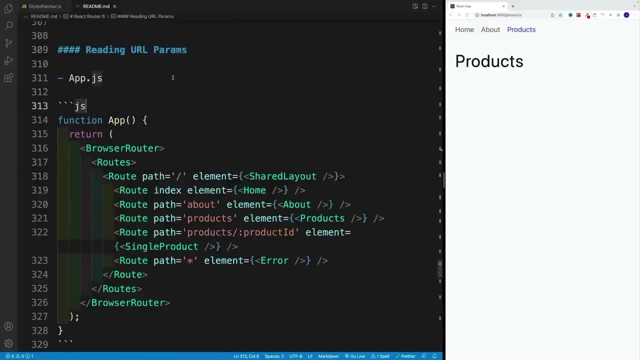 inline CSS option as well. Most importantly, you have nav link, then the function, then object in the object you have is active, And then you can use this value to set up the class. All right, and now let's see how we can read URL parameters And, as a result, we'll have: 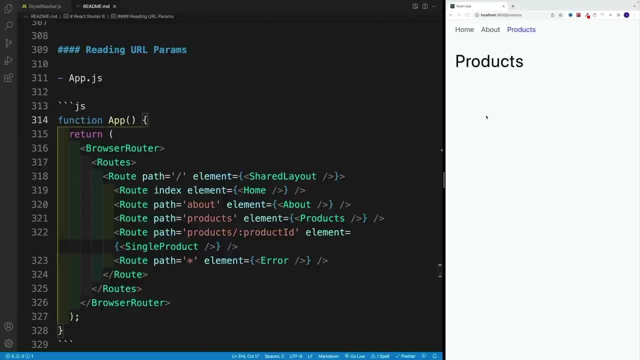 some dynamic pages, And for this I just want you to imagine a product page where we display bunch of products And then, once we click on that one specific product, we display it in a separate page. Or here's the key. I don't want to set up a separate page for every product. 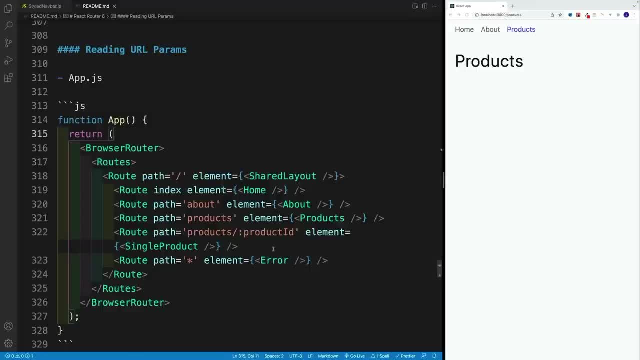 that I have. It makes more sense for me to set up one page which is going to act as a placeholder, And then I'll just get the data that I need to display, So that way I can use the same page for example, 4000 products or 3000.. And hopefully you see where I'm going with this. 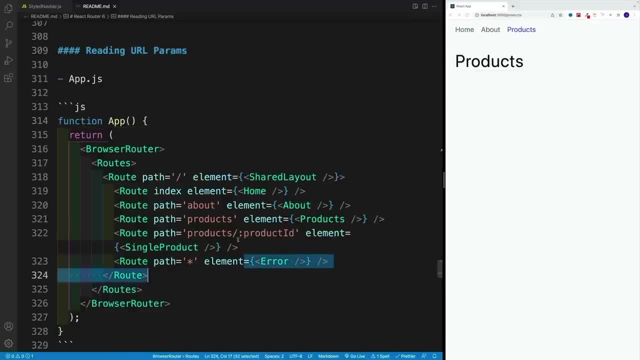 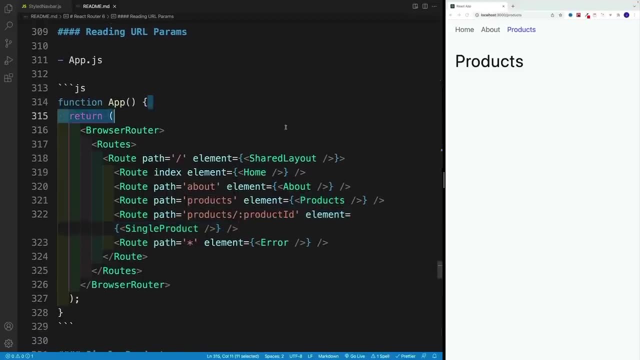 And, in order to set up URL parameters, you want to go with this colon and then whatever the parameter name, call this shake and bake, call this vegan food truck, And then you can go with this product. In my case, since we'll display product, I just thought it's going. 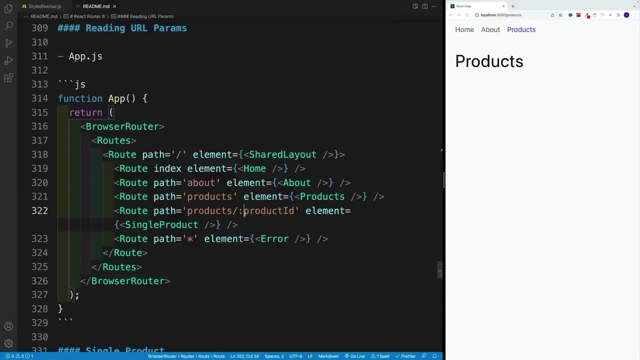 to make more sense if I'm going to go with colon and then product ID, But this name is really up to you. Now, as far as this URL, this can be straight up like. so, where we go with colon and product ID, this can be products stats and then product ID- Again this part. 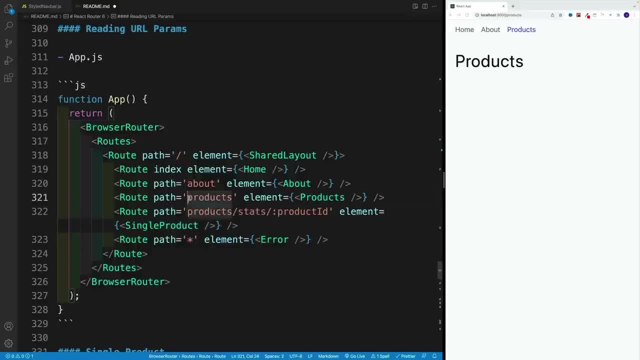 is really up to you. I just thought that going with product and then product ID is going to make more sense. Before we begin, I also want to quickly mention that, yes, you can set up that nested structure Like we did over here for a product and product ID as well. I just went with this setup for 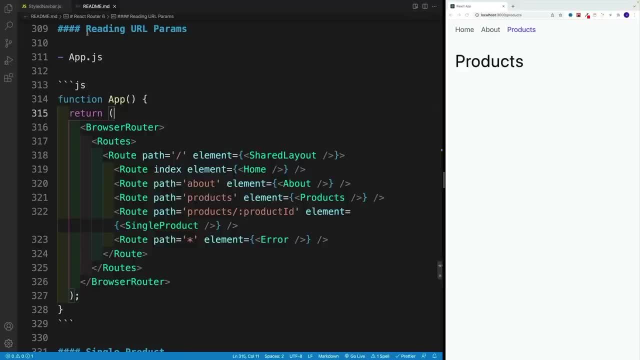 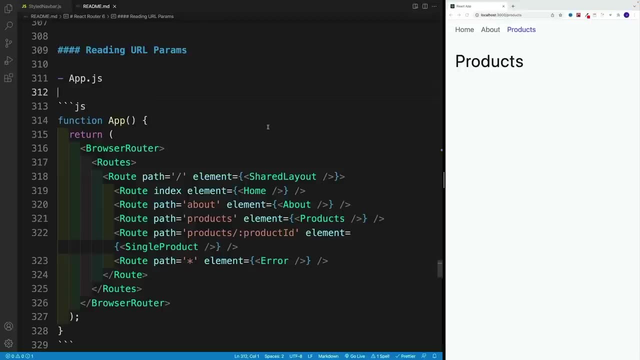 two reasons. First, I really really, really want to focus on the URL params, And I think it's going to be better if we use this setup, So that way, it's easier for us. we don't need to do this. 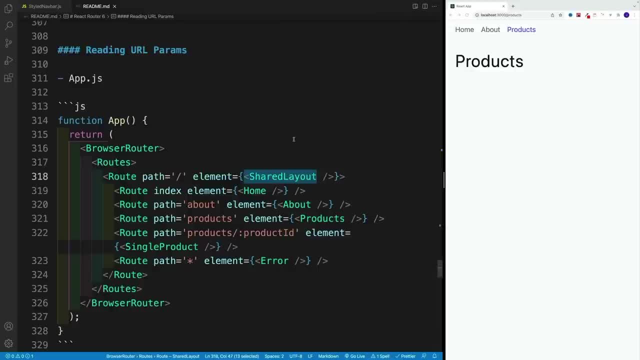 whole song and dance. And second, I also want to showcase that if you don't have the shared layout, which, in this case, we want, you don't always have to use that approach. you can also use this approach as well, where you go with whatever is the main URL, And then 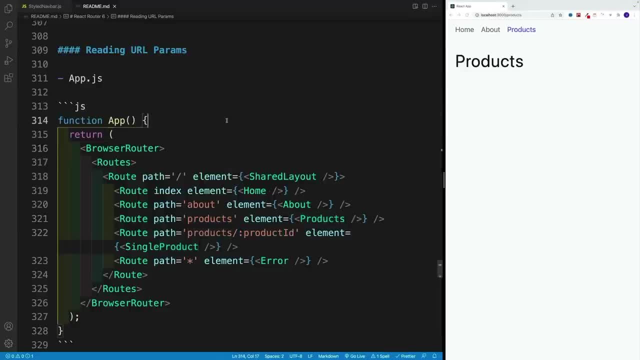 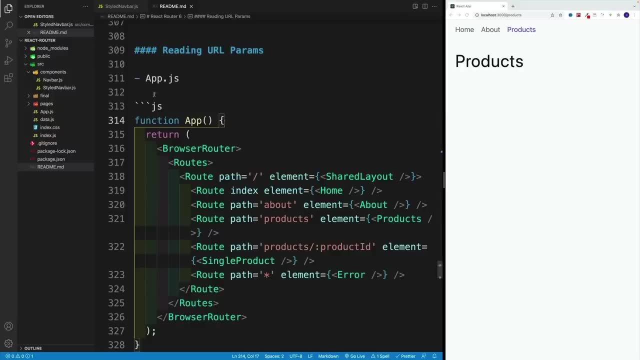 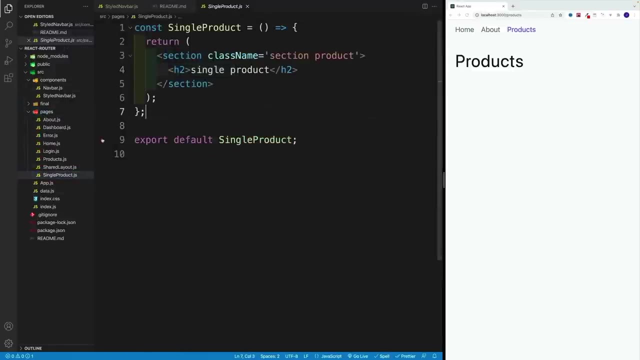 in here specifically, we go with this dynamic option. Hopefully that is clear. So first, let's navigate right now to objects and get that signal product. So if we take a look at pages, there is already a single product. just stay heading to. So when are we in the 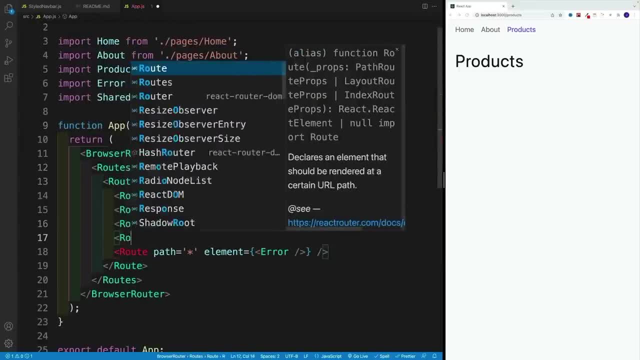 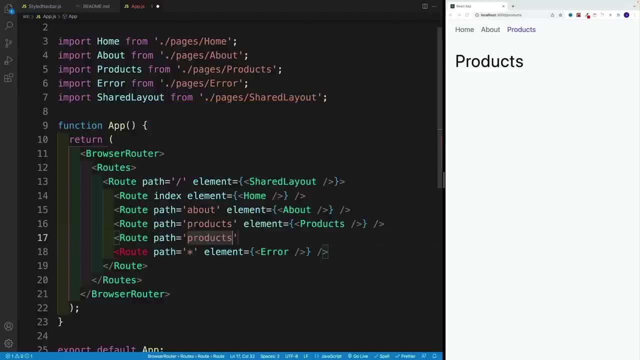 app, just first of all set it up, and I'll do that right after the product. So let's go with route of an path. Then we'll go with products. Man that product ID And you'll see that it is essentially a product. Preparation is needed here. So let's go ahead and see what that looks like. So when we go over here, we can see it's a standard product ID And you'll see that it is essentially a product with amenities. and then you'll get the option to have a contact with people. You'll 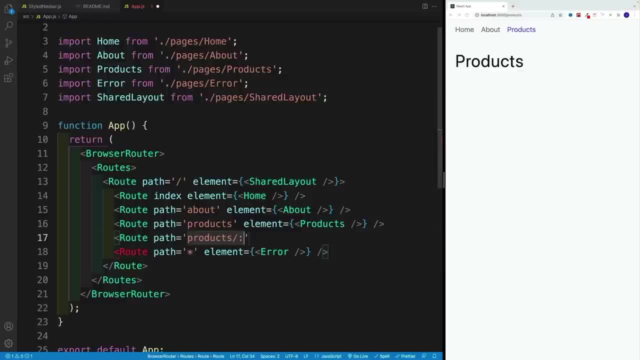 also see that the system is an app ID. So you have a product ID And let's see, we'll go here let's property. So again we can name it whatever we want. So go with colon product ID, And then what? 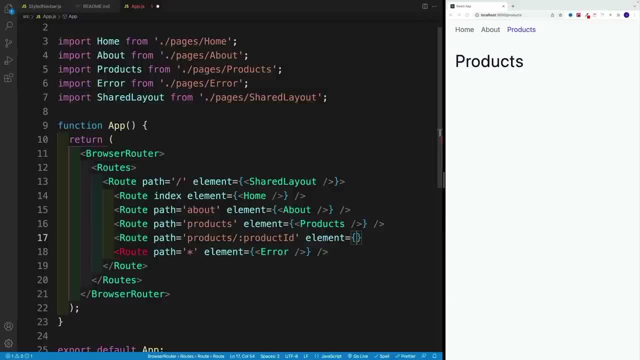 is going to be the placeholder. Well, we want to go with element, And then we want to go with that single product which hopefully is going to work but doesn't look like it. So that's why sometimes this auto import is annoying because it doesn't work. So let me save this. And yes, of course, 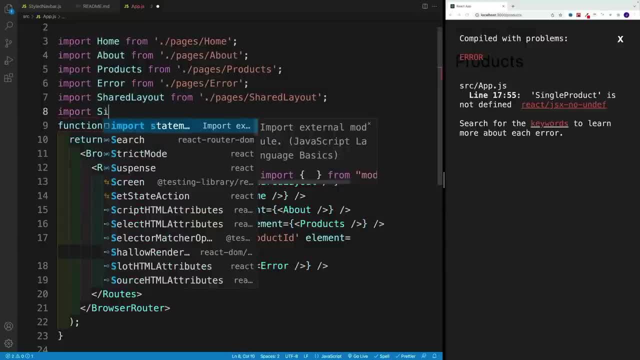 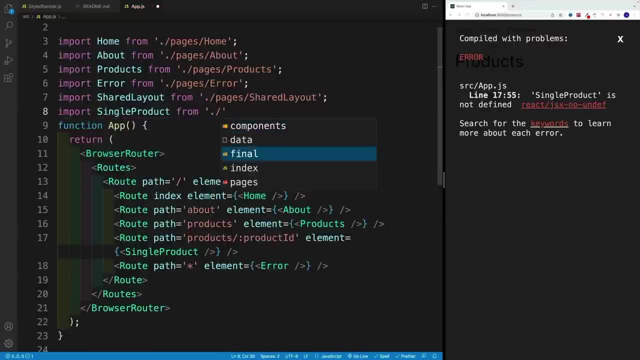 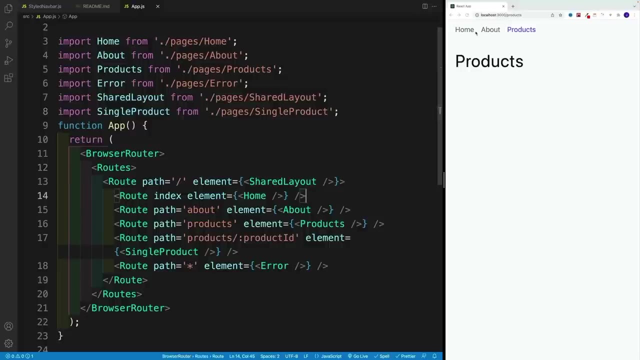 I have the error. So let me go here with import and then single, single product like so and that is coming from- and we're looking in the pages, I believe right- And then we have single product. So not everything works. we have that single product. And now if we go to URL, if we just type whatever, 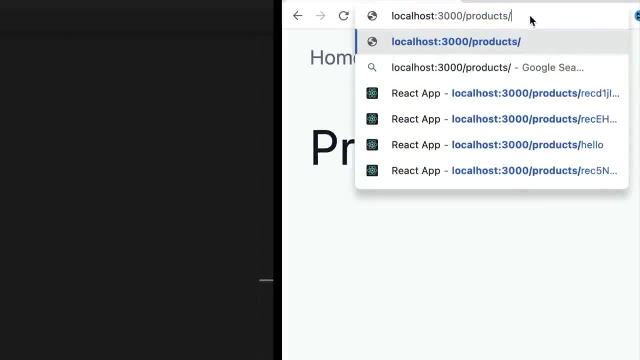 gibberish we want. so eventually there's going to be actual data, because I already prepared for you. But let's say, if we type 123, we have single product. if we type I don't know, three, three, three. 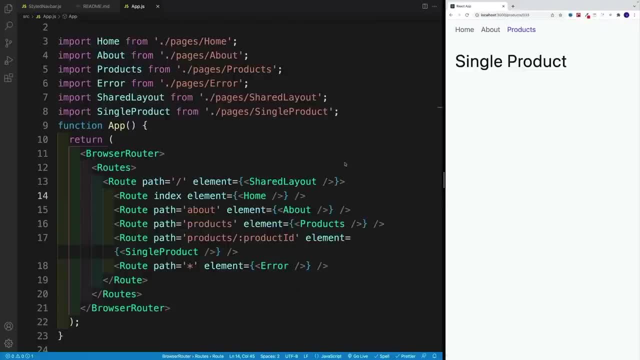 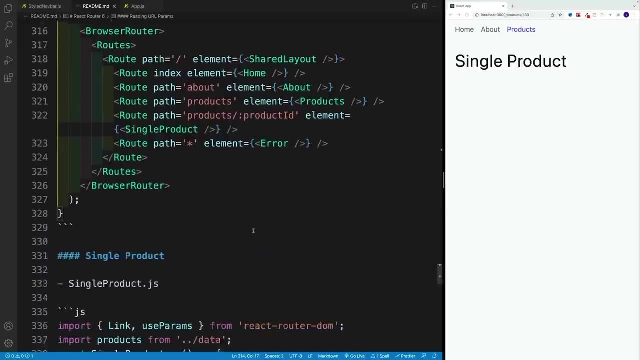 we'll also get that single product. So that's the placeholder we're going to use. So now let's navigate to the single product And let's take a look how we can access it. So this is the setup, where we go with that colon and then whatever is going to be. 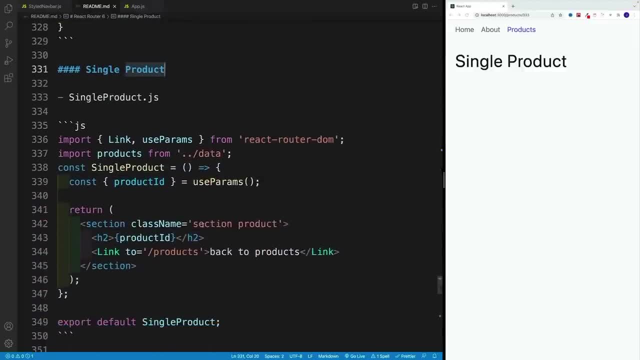 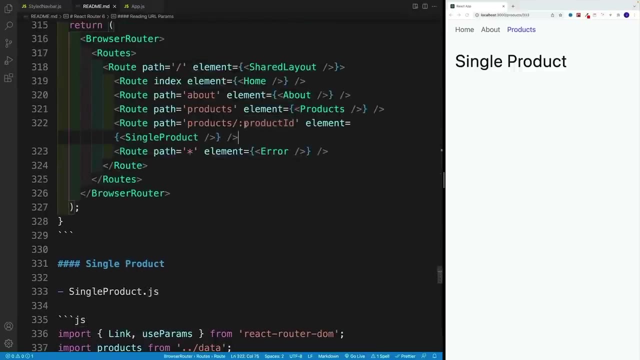 the parameter name, so in my case, product ID. Now, if we need to access it, we need to get the hook from React router DOM. So use use params and we'll also get the link. And then we want to invoke that hook And notice how this name now needs to match whatever we have. 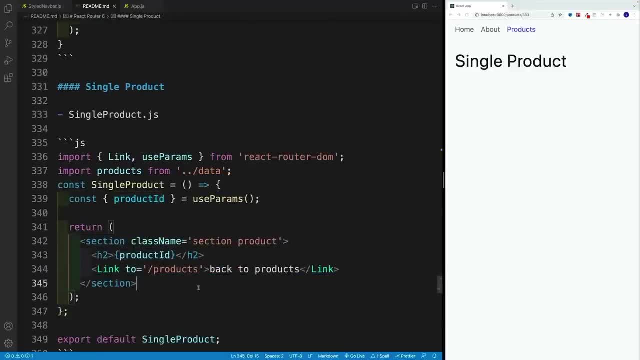 over here. So as long as they match, you'll be in good shape. And then, for time being, let's just display it And let's navigate back to the main product page. So let's set this one up where I don't think I'll need to style navbar and more, But I do want to navigate to style navbar. 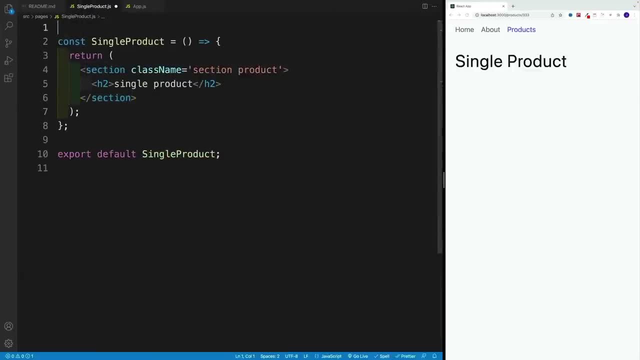 single product. Like I said, we're going to be looking for two things. we're gonna get the link first, And also we want to get that hook use parameter which is going to access those parameters in the URL, when all of that is coming from react And yep, it's not correct. 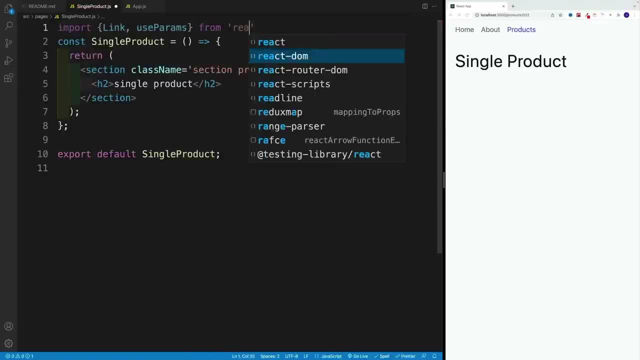 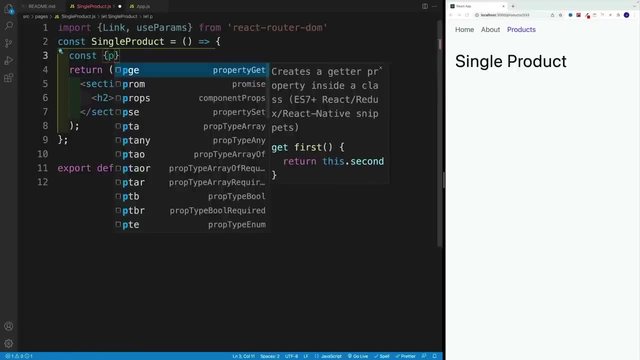 we need to go with import- My apologies, not const. So let's go with react router, DOM. And as far as the return, first we want to grab that product ID. And you know, as a sign out, why don't we do this? Why don't we just log this sucker? So let's say your use params. 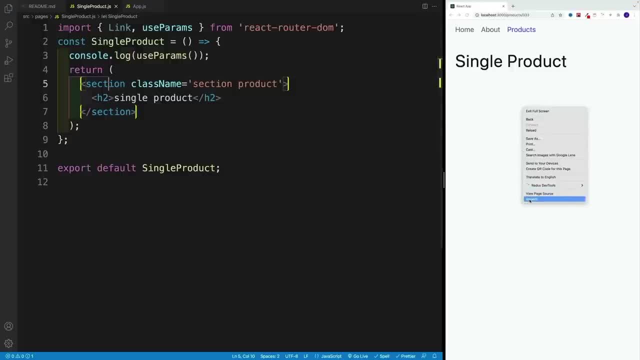 and you'll clearly see what am I talking about. So let's invoke this And then let's navigate to the console and check it out. We have the object- What do you know? we have product ID 333.. So if we'll change this around 123, then of course that value will be also you. 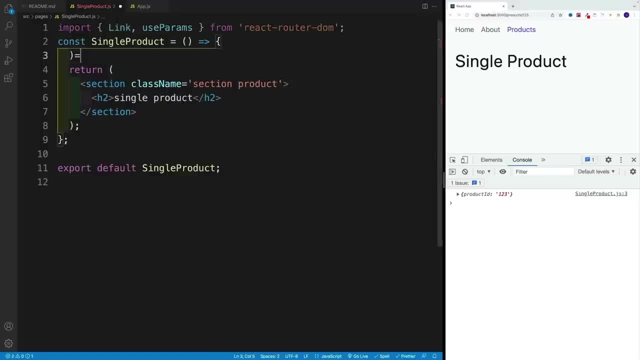 know 123.. So now we want to pull this out from the use params, from the object. So let's go with product and then ID. That is equal to use params, Let's invoke it And, like I said, let's set up that link back to the product Push. If you want, you can navigate also back. 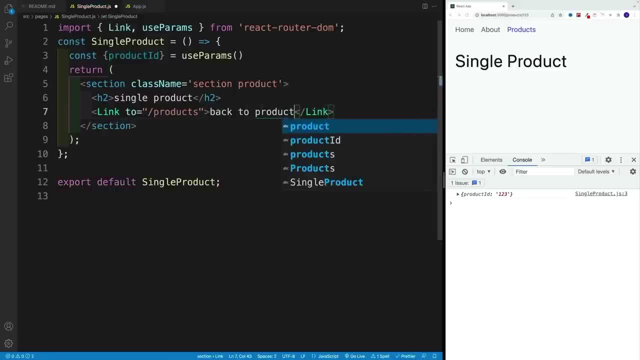 home. but I guess it's going to be back to the product back product And where we have right now the single product, go with adding four And let's display the ID. So let's say here product and then ID. 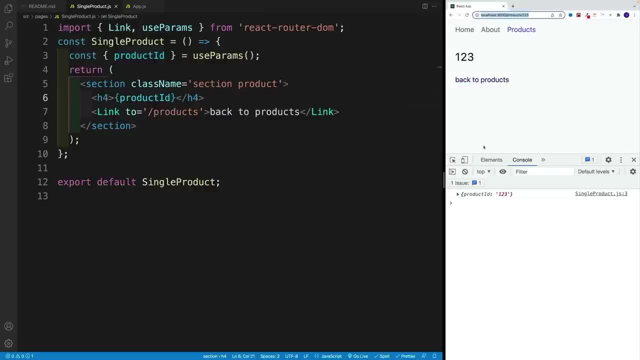 let's save it and check it out. Now we have 123. Again, if we'll change this around to 4567.. And this is going to be the value. So next video we'll iterate over the products that I provided in. I believe data js will render all of them in the products page And then from there we'll set. 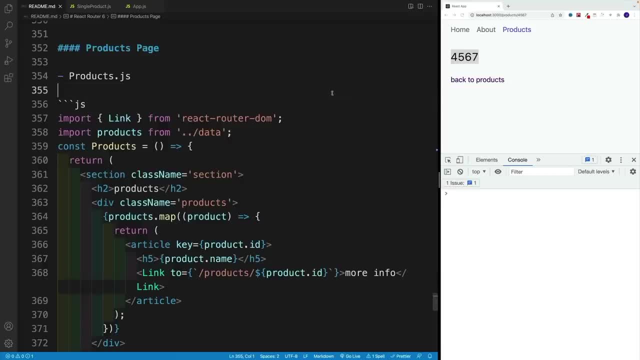 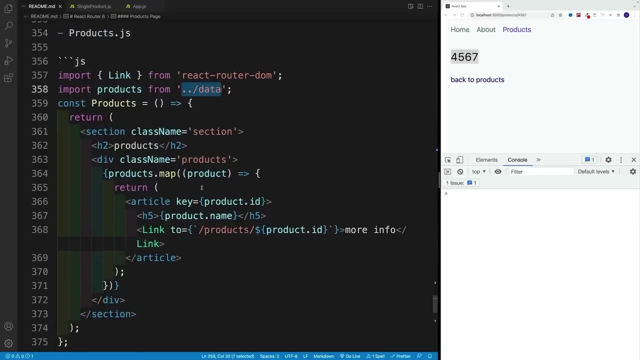 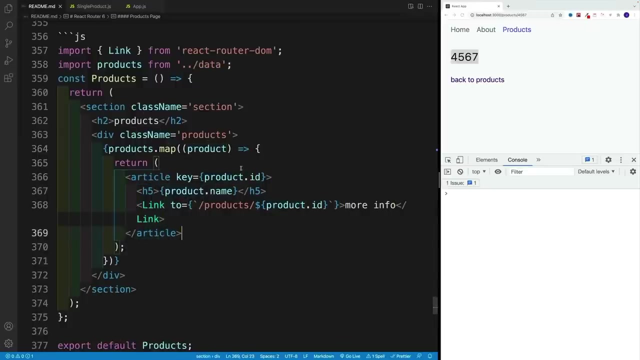 up a single product page as well. Alright, and once we have the single product page in place, now in the products js, let's iterate over the products that are coming from the data, And then, for every item I want to return an article, we'll have to use the key, since, of course, this is a react. And then I 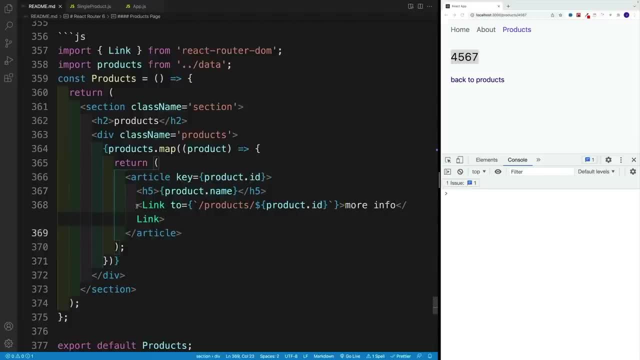 want to access product name as well as product ID, which I'll pass into this link And notice the URL. Again, this needs to match whatever we have in app js, Since in the app js we have products and then product ID. This is where we dynamically pass in the ID property, which is: 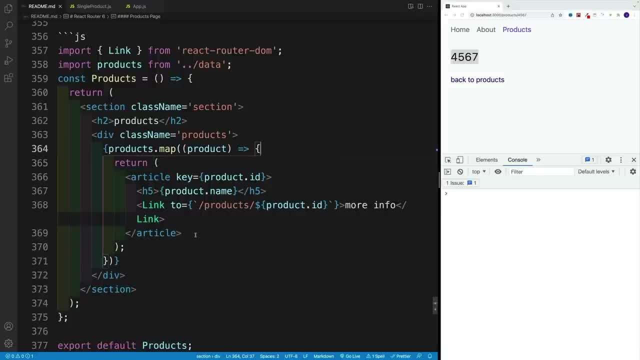 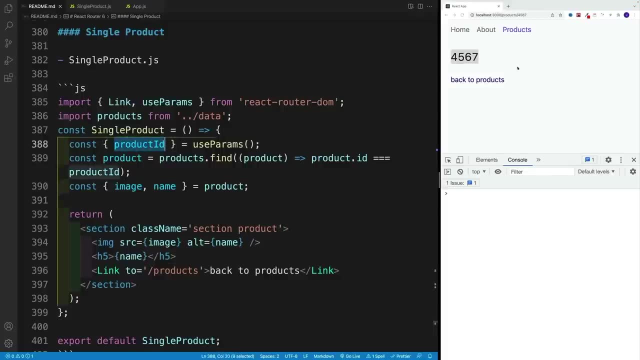 going to be in every product. Once we set this one up, then in the single product we'll use that ID And instead of rendering it on the screen like we have right now, we'll basically pull out that one specific product. 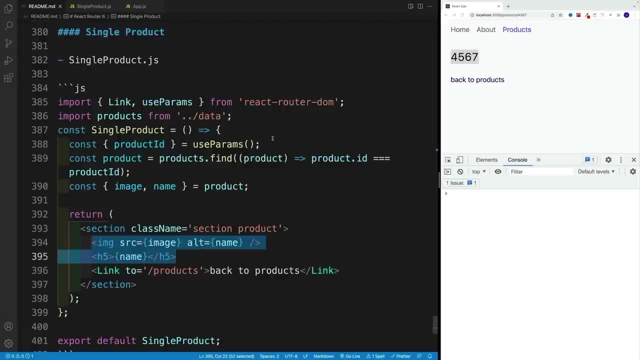 then we'll get the image and name And then we'll display it. Now, before we continue, let me right away say that, yes, normally we'll get this data from the API or database or whatever, But since I want to keep this nice and cute, that's why I prepared this. 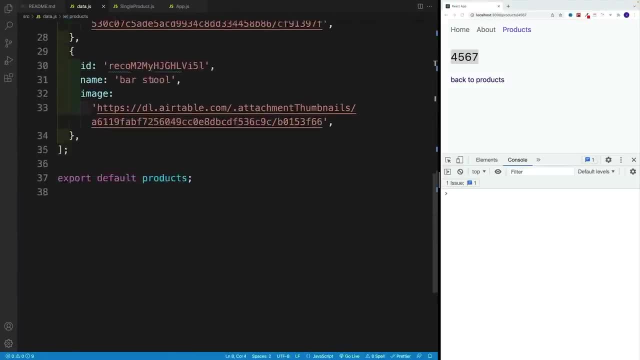 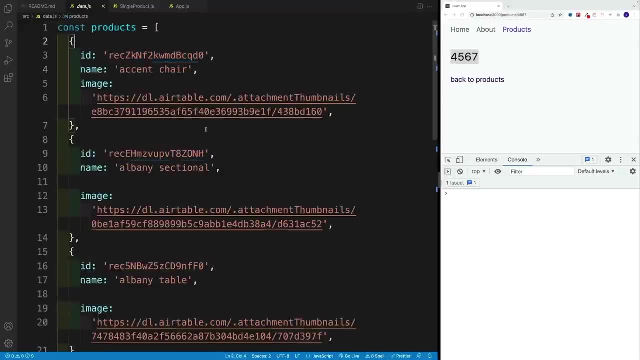 data js, which essentially is just an array of products. each product has the ID, So this is something we'll see, or here in the URL name, as well as the image, which is just an external URL, So these images are stored on a cloud somewhere, So that way we don't need to bother with the local. 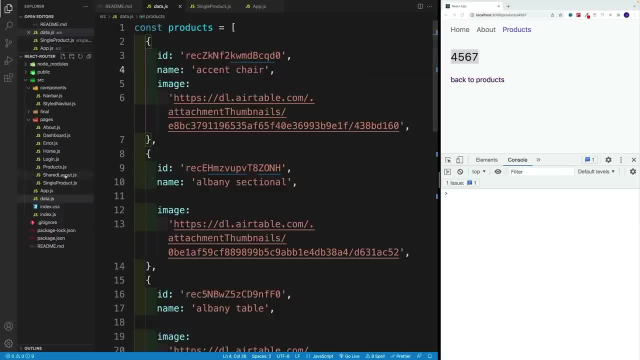 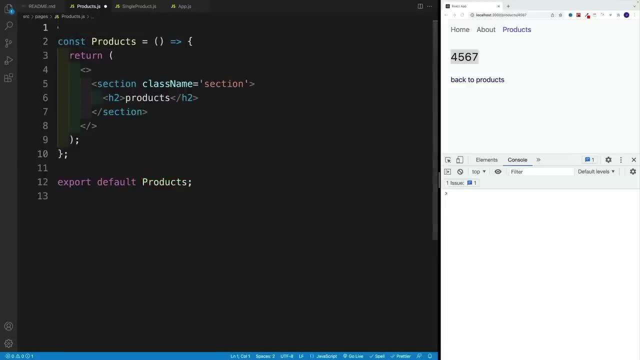 image setup. So first let's go to a product And we want to get the data Now. if you want, of course you can log it, but I'm just gonna assume that it's there, And also we want to get the link. 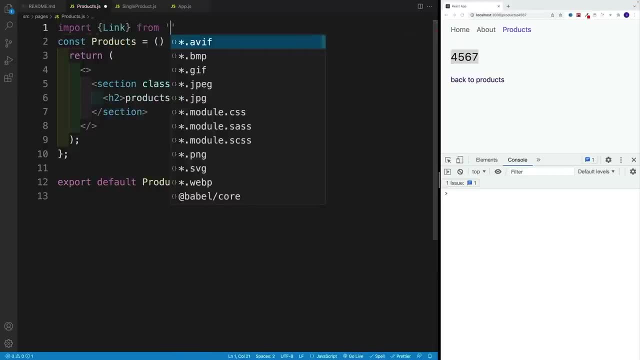 because each and every product will be wrapped in a link. So react router down, then after that let's go with import, then product from. like I said, we're looking for the data j s And as far as the return it looks like for some reason I set it up as a react fragment. 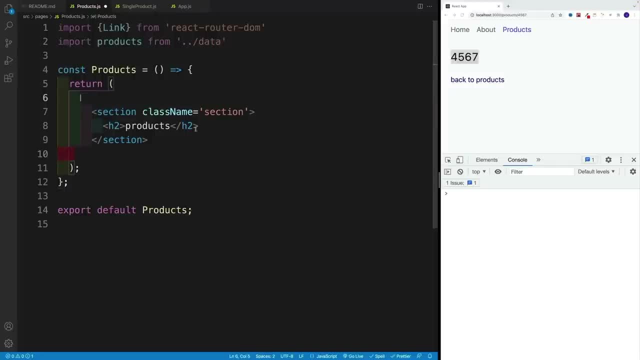 my bad, let me just remove. we'll have a section here, product, And then right after that we want to go with div, with a class of product. So then there's a little bit of styling over there. Let's go with product map or mapping over, And then as far as 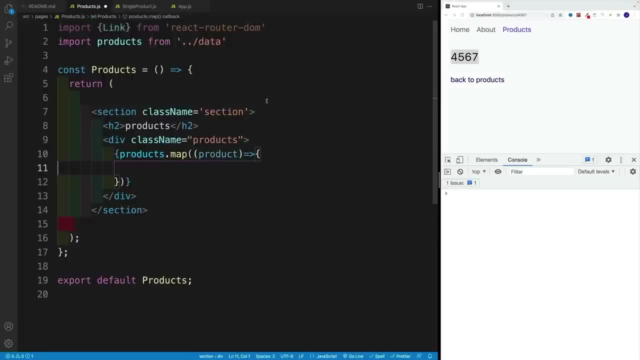 the return. let's go for product Again. if you want to log it, you can definitely do so. in my case, I know that essentially there is going to be all of those properties, So I want to return article. I do want to add right away a key And I'll just say here: 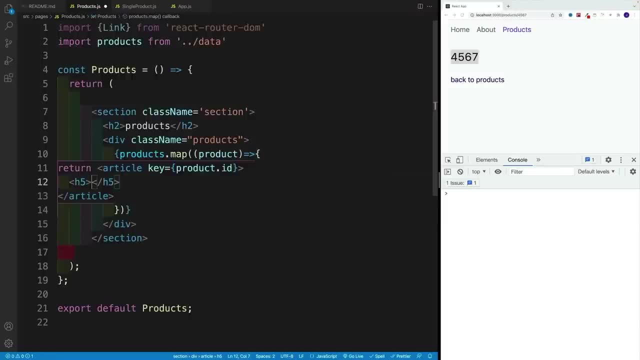 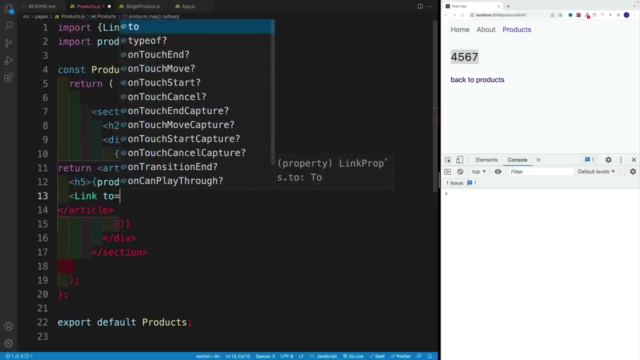 product ID one. I also want to go with heading five and I'll say product name And also we want to set up that link Now. I believe previously I mentioned that we'll wrap it. my apologies, we'll just set up the link here. So let's go here with link to now remember this is dynamic Now. 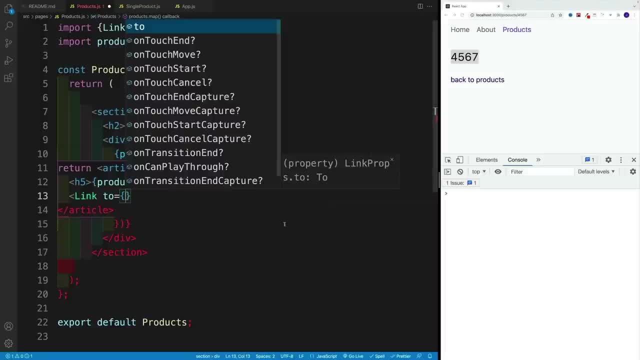 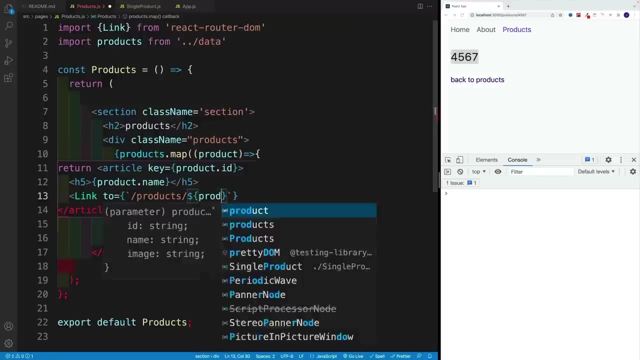 we are not passing this manually, 456 or seven. we actually go with product path and then that dynamic ID. All right, so let's go with template string, then product and forward slash, And now let's access that sucker. Let's say product, then ID And then set of it. let's just say more. 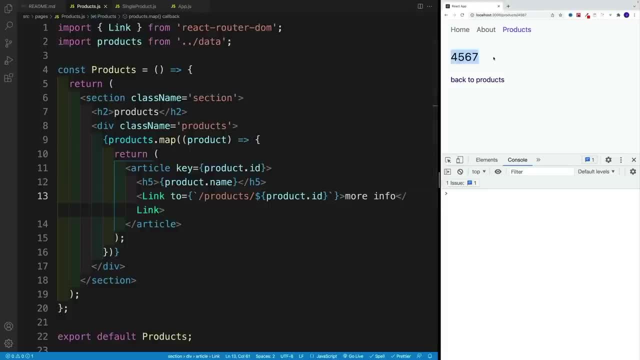 info. Let's save it. And this is that single product, So we won't see anything. But if we navigate back, check it out And we have a list of products title as well as the link. So this is going to be more info. Now notice: we have this unique ID in two places. We have it over here And 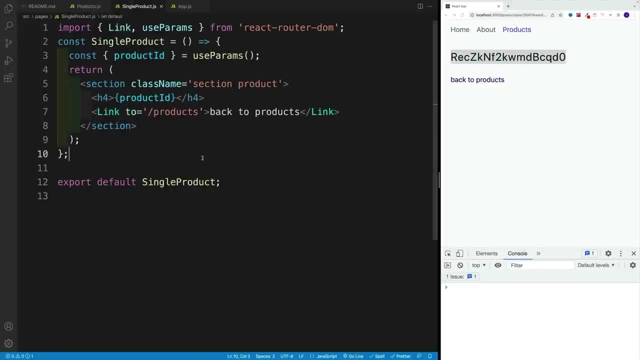 we also render it. So now we just need to add some code to single product Where First I'll grab it. Okay, that's good, But I also want to get the products from there right from the data. product from the data. Very good, Like I keep saying normally, this is going to happen with some kind 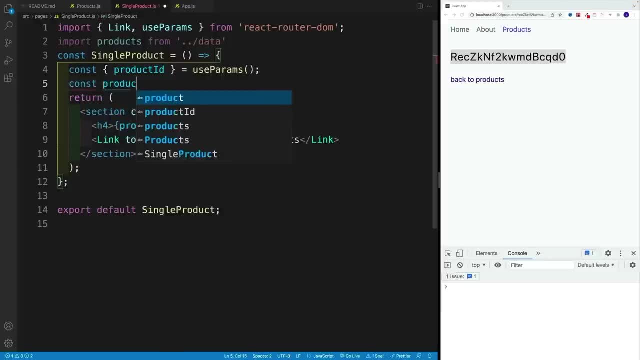 a fetch request from the API and all that, but not in this case. So I want to get the single product that is going to be with products. then use find And I'll just say: get me the product whose ID matches the product product here and then return. a product ID equals. 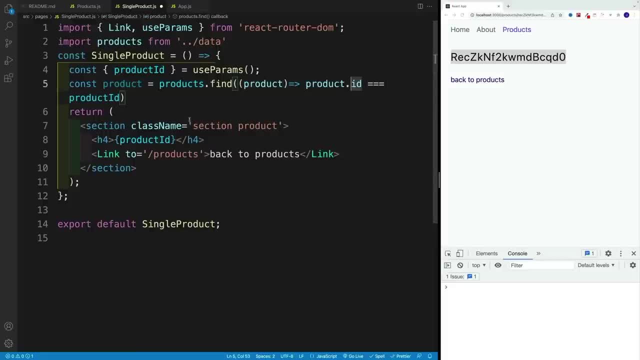 to product ID, like so. So product dot ID equals to product ID. Beautiful, Then let's pull out image And now we don't need the idea anymore, And then let's set it up in our return, where first we're going to go with a heading five, I guess, And instead 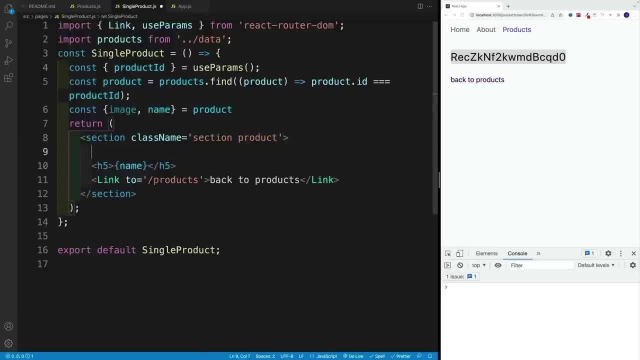 of product ID. I want to display the name and then right above it or below it or whatever, Let's just go with IMG. source now will be equal to that external image, So let's set up the image over here. If you want, we can also set up the. 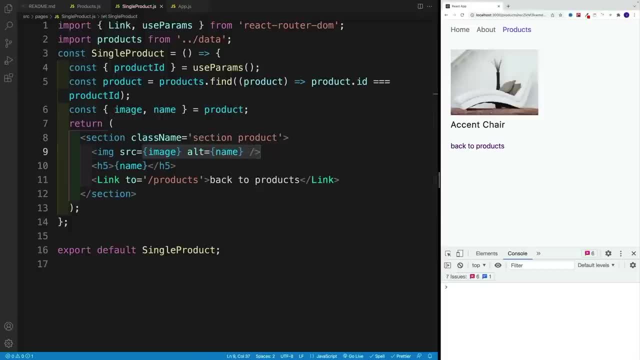 alternative. Let's close the image And, as a result, we get this single product And, like I said, now we can set up 1000 products So we can render them in the products page, And then for each product there's going to be a single product page, essentially, which. 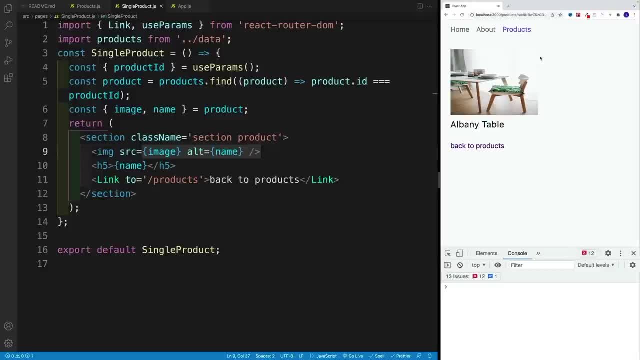 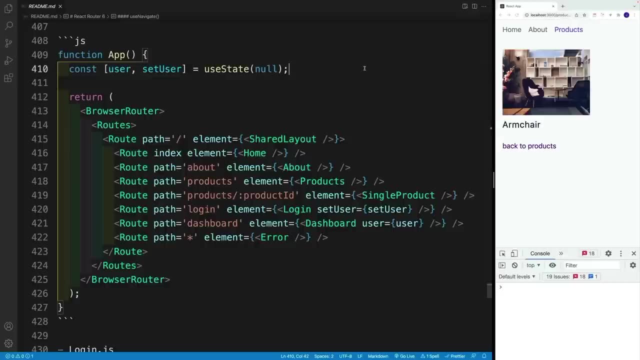 acts as a placeholder. we'll fetch the data about that one specific product And we'll render that in the single product page. And now let's see how it works. So let's go ahead and create a single product page And let's see how we can navigate around our project programmatically. In our case, that is going. 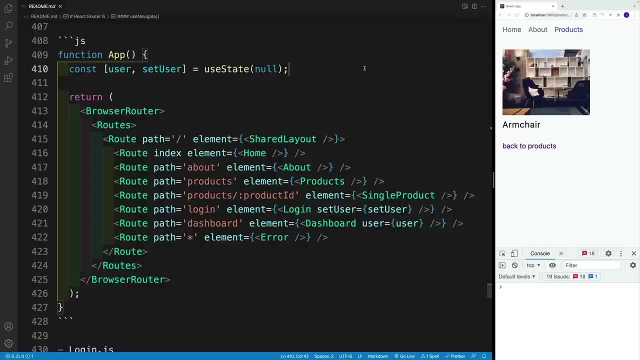 to be once we submit the form, And also let's see how we can restrict access to certain routes. Before we begin, though, please keep in mind that normally, we will use context to store our user value. In this case, I just didn't see the point of setting up the entire. 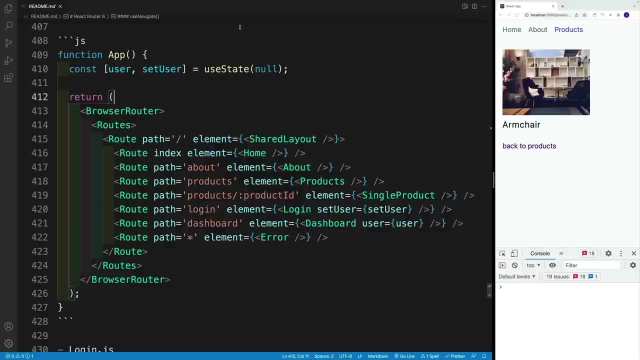 boilerplate And we want to start in the app Where you want to set up user state value with your state, and initial value will be known. then we want to import two more pages. we want to import the login page as well as the dashboard And again the boilerplate placeholders are already there And then in 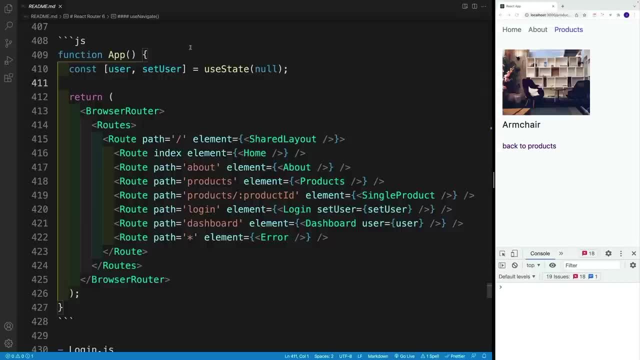 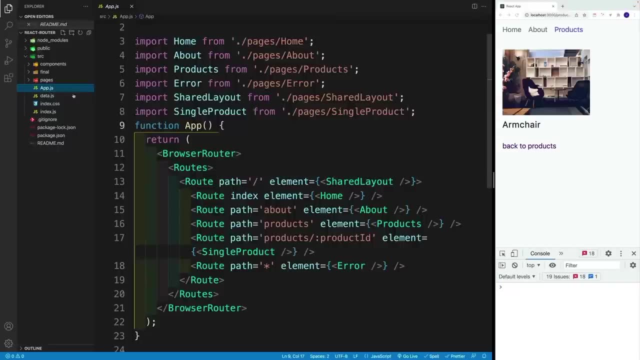 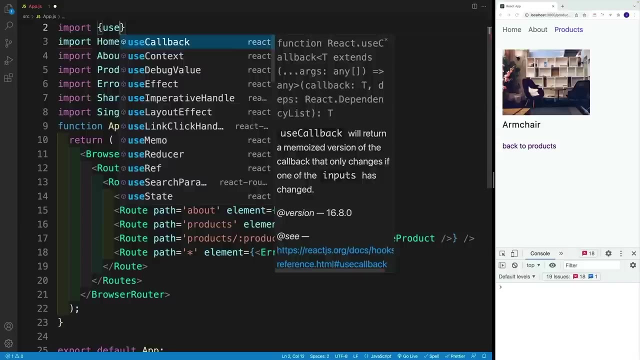 the login one, we want to pass in the function, the one that sets up the user, And in the dashboard, we want to pass in the actual user. So let's start in the actual user. So let's start in the app j s, where we want to get the use state from react import use state. 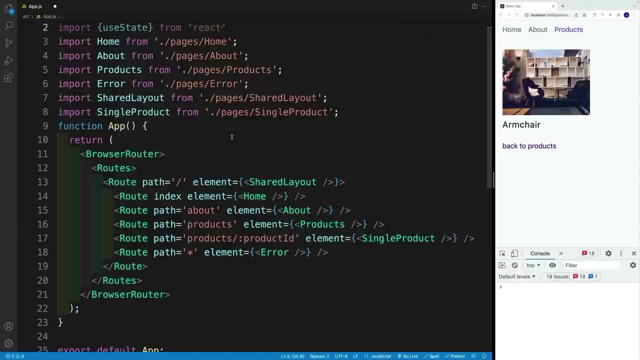 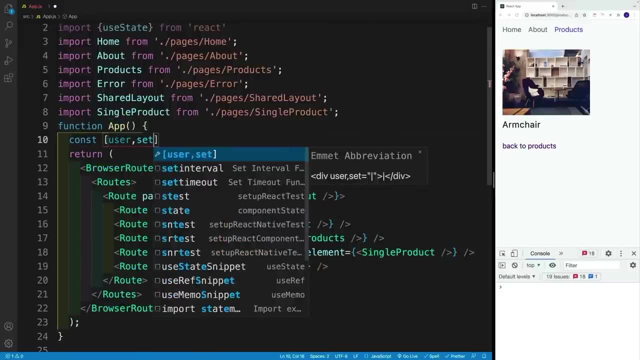 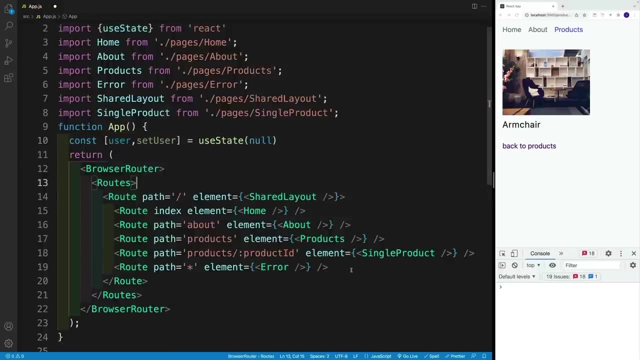 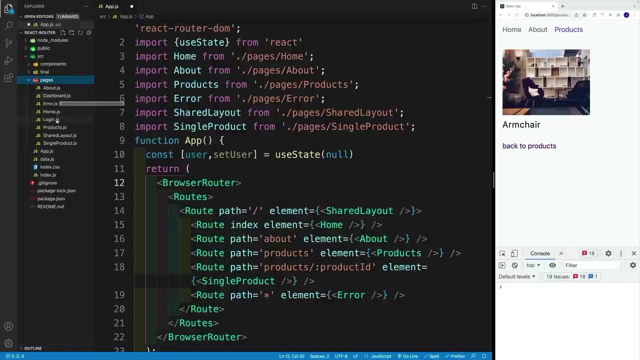 that is coming from react And let's set up that state value. So here let's go with const user, set user as equal to use state And let's pass in. Then let's grab both of those pages. So we're talking about the dashboard as well as the login one. Now dashboard doesn't have 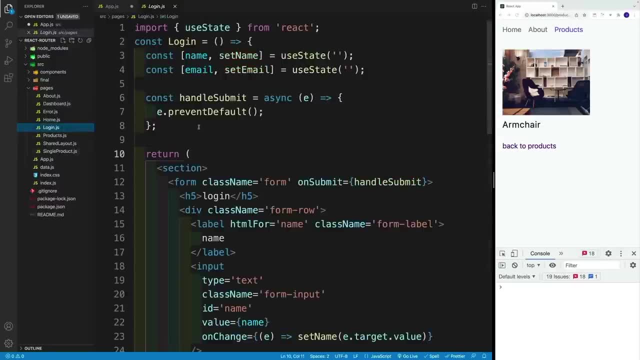 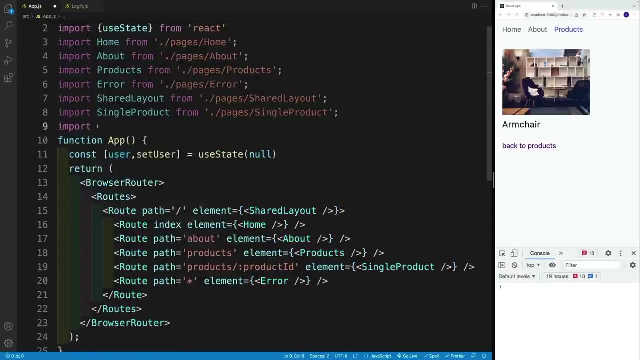 anything. pretty much it's the same boilerplate and login has a little bit more, and I'll cover that in a second. Now, since my auto imports were not particularly successful, let's try it here where I'm going to go with dashboard, dashboard, And again it's not working. So 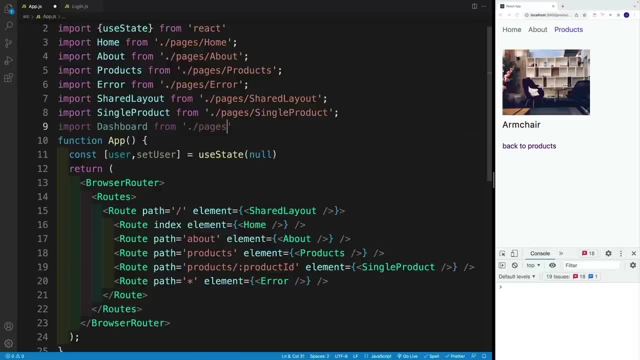 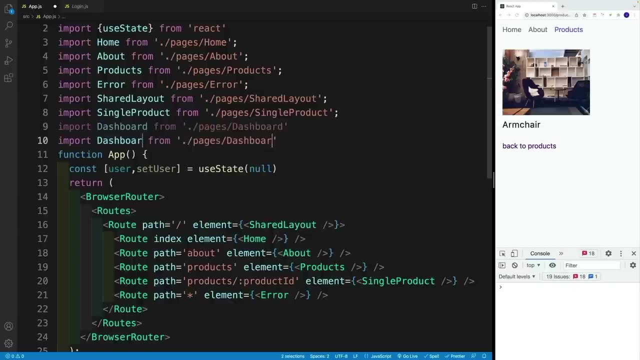 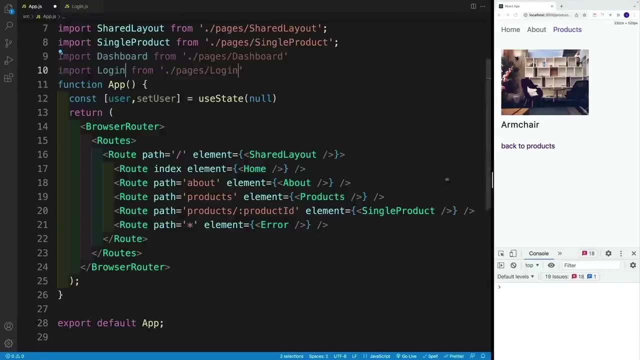 what's up with that? So let's go with pages, then let's access the dashboard And then let's copy and paste. In this case, let's delete And we'll just go with login Then right after that single product. first of all, I'll make my browser bigger here. I want. 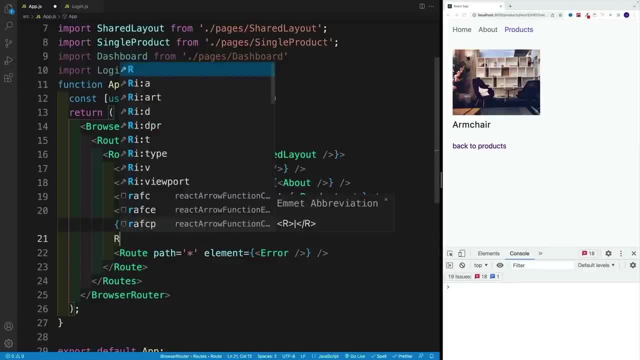 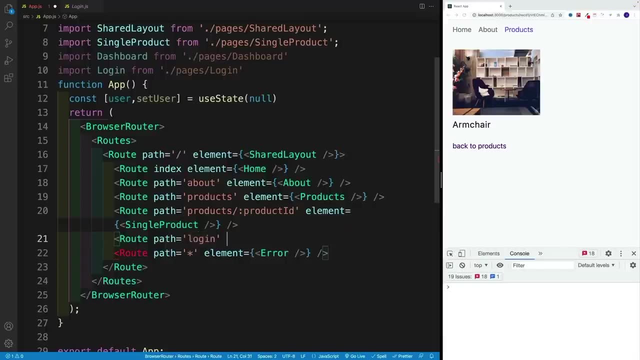 to go above the arrow one And let's set up that route, the login one, So path will be login. And then we want to go with element And let's pass in In the login one And then, instead of the login element, let's also pass in set user. 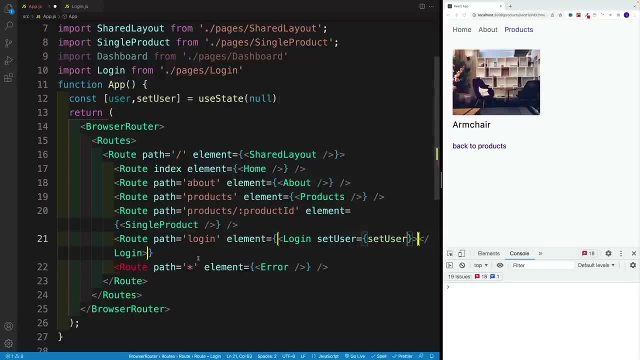 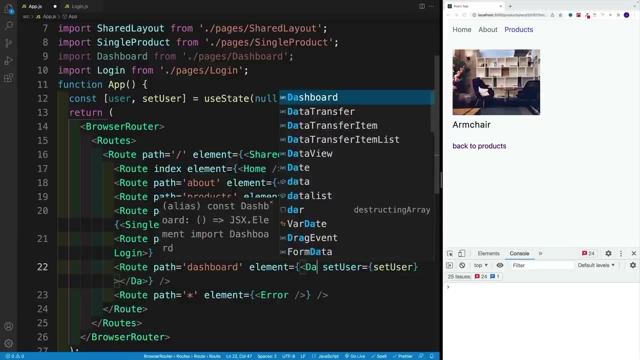 is equal to set user. So now we're passing in this function. Now we do want to close this one, meaning the route, So let's save this, Then we'll copy and paste. this is going to be dashboard, dashboard, and the component will be dashboard as well, And instead of 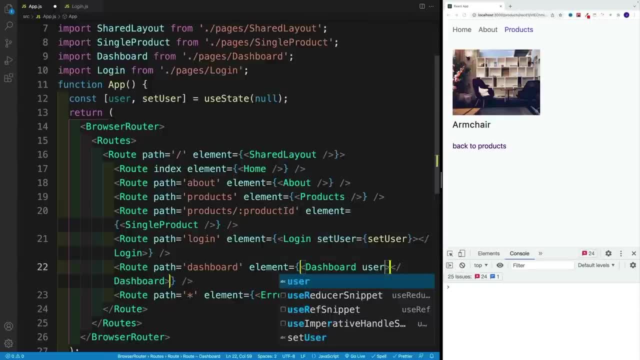 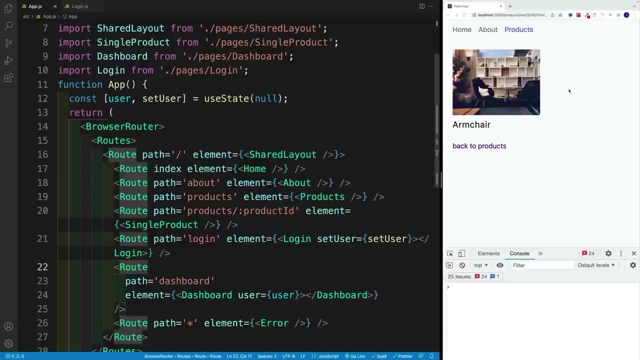 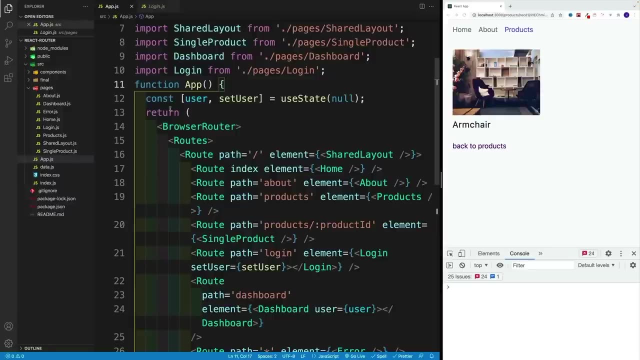 set user, go to user. So user is equal to user. Let's save this. Now let's navigate to the login one, And you know what? actually, I also want to add the link to the login one, So not to the dashboard. 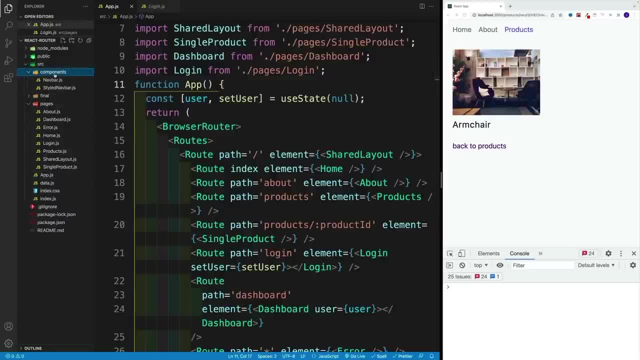 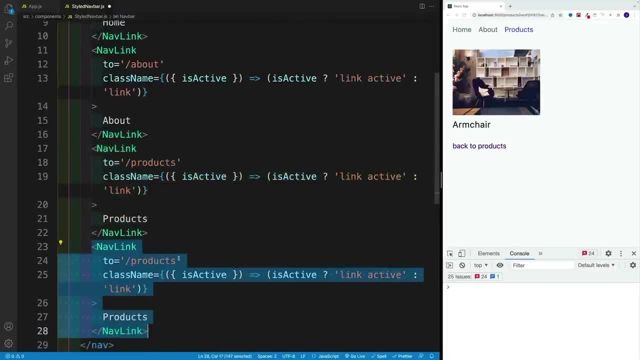 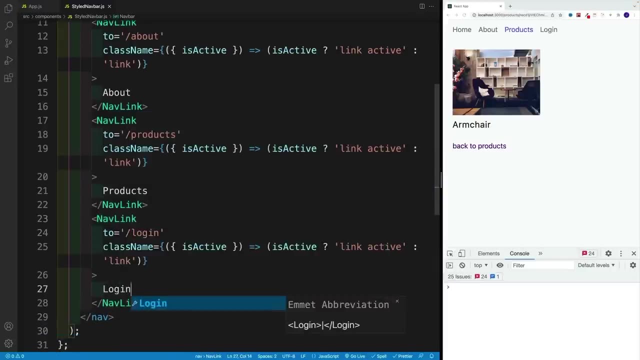 but to the login one, And if you remember, that was in the style navbar. So let's navigate here And let's add one more link: copy and paste. this is not going to go to product, this is going to go, And then also the text will be logged in. Let's save it. we have the login Once we. 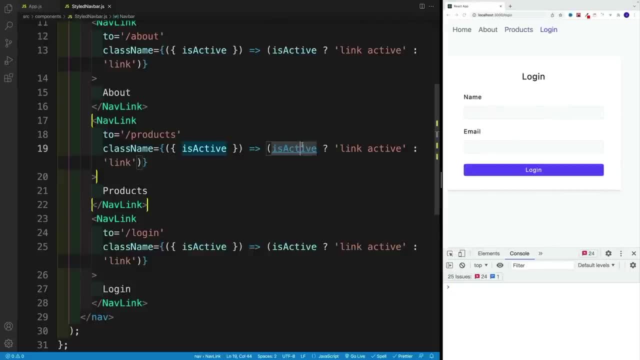 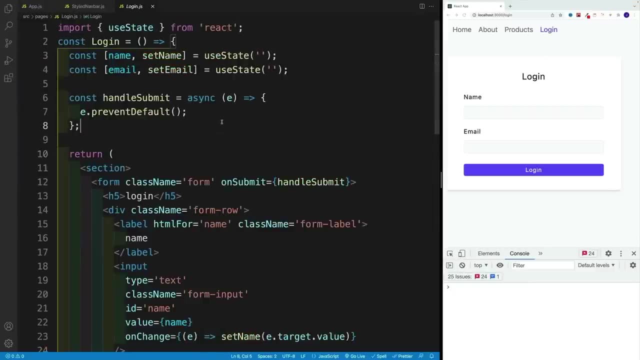 navigate here, we notice that we have the form, which is awesome. So now let's navigate to the page And we'll take a look at what we have and what changes we need to add. So I imported use state. I have two state values, I have name and email, and I right away have 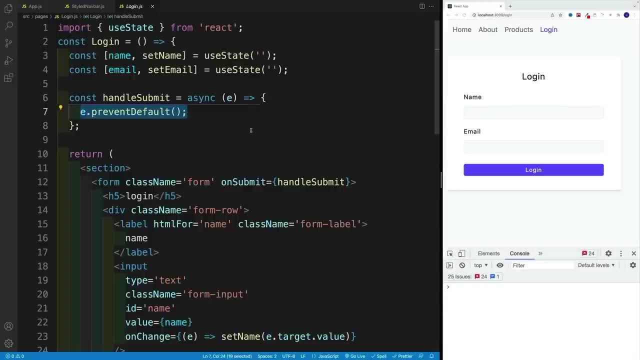 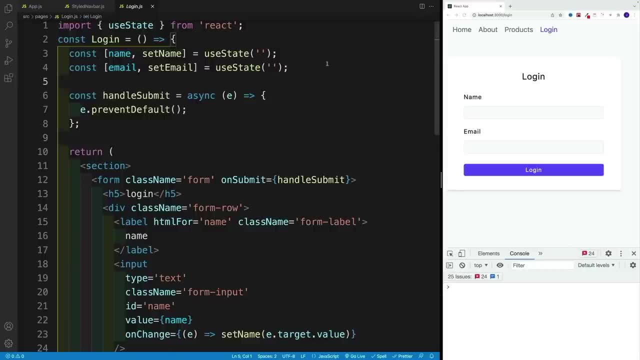 the handle submit where we have prevent default- pretty much basic setup. Also, both of them are set up as controlled input, So they are tied to the state value. So as you start typing you basically will have both of the values over there. Now, if you want to test this out, 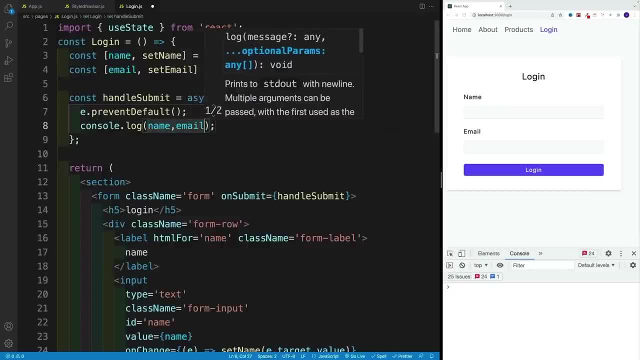 let's go with log and then say name and email. Yeah, I'm pretty typical setup, So I'm going to go here with john John gmailcom And once we log, check this out, we have both of the values. So here's what we want to do In the log: in one, we want to check that we're. 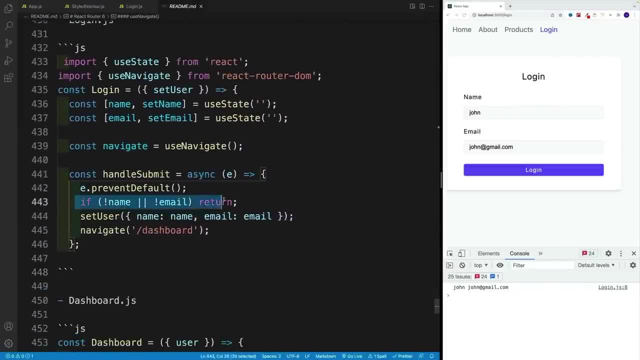 going to have any of theseなんだ here And say they're in the��o of the data set. now an example: like you're causing our datos on Google, which is not the data you're making, check whether both values are there. If they're there, First we want to set the user, So 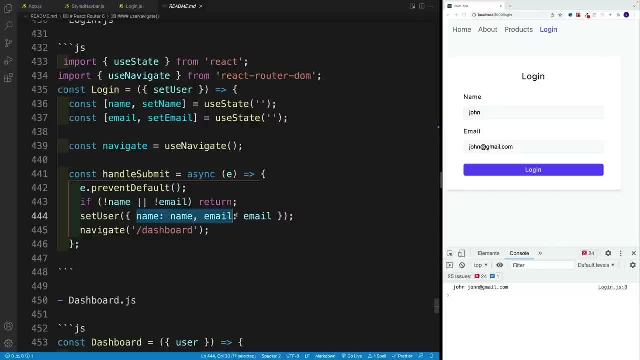 this one is coming from the app js And, yes, I purposely went here the long route. And then we want to get use navigate from reactor down And we want to navigate programmatically to the dashboard. Notice, in this case it's not happening once we're clicking on a link. 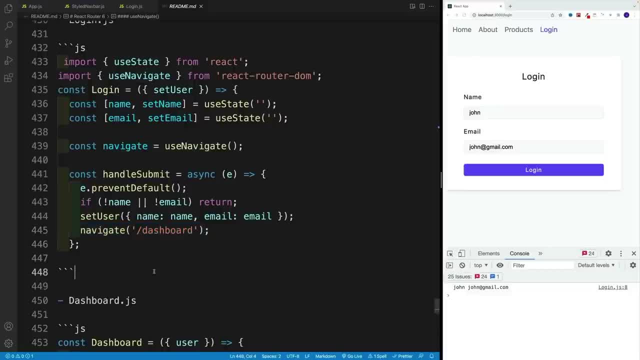 or nav link. In this case, we'll navigate there using navigate And in order to invoke that we get to use navigate, we invoke it. this is going to be equal to navigate, And then in here we just provide where we want to navigate And then in the dashboard- since 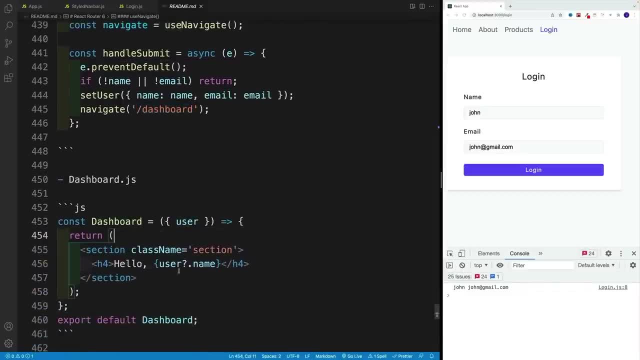 we can access the user. I just want to say hello and then the username. Now we are using optional training because, remember, initially it's going to be now, So let's try to set this one up. We're in the login. 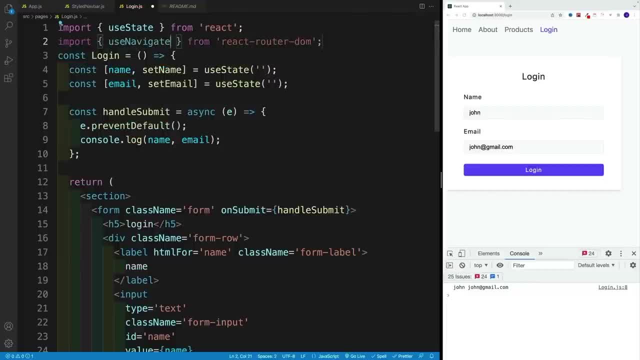 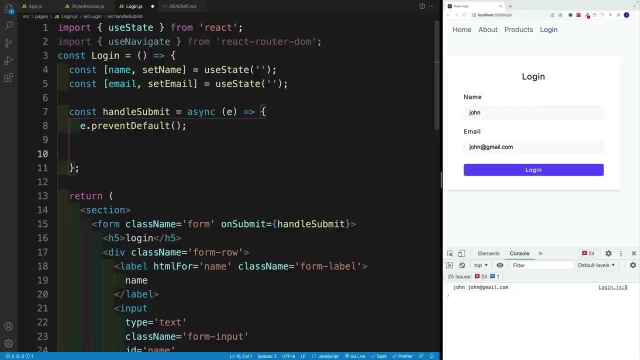 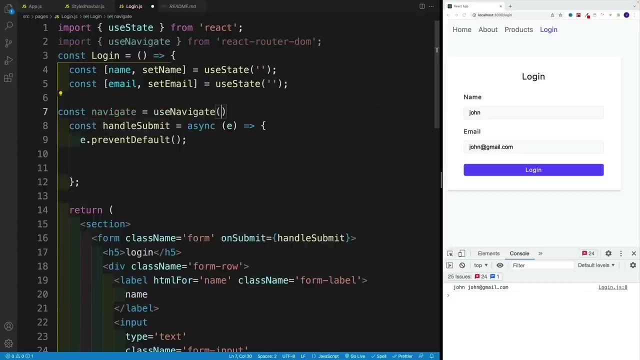 First, let's grab that navigate. use navigate is coming from react router down. then I already have the console log. Okay, beautiful, Let me remove it. And in here above the handle submit: let's set up that navigate. So navigate is equal to use navigate. Let's invoke that. 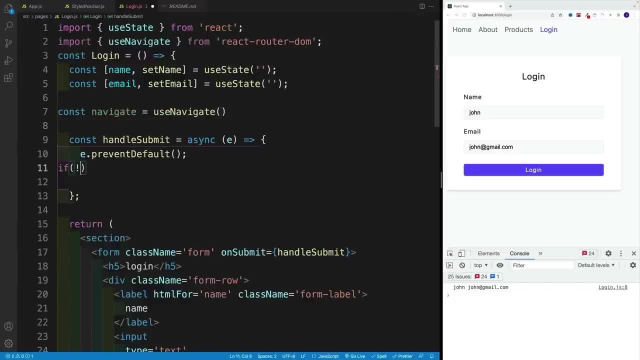 And then we're going to go with if condition. So if there is no name or there is no email, So if one of them is missing, then we want to return And yes, that is the check that I'm going to set up right now. So there's going. 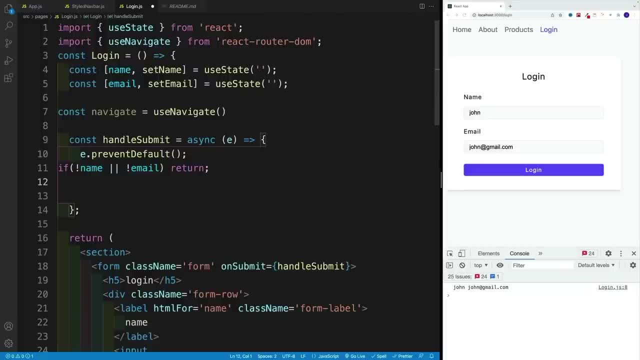 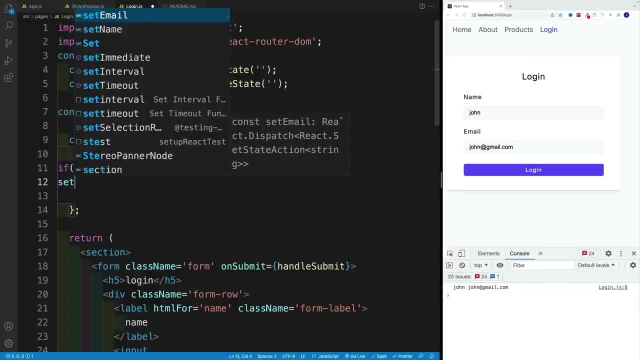 to be no error messages, nothing like that. I just want to check whether one of them is empty. If one of them is empty, we'll simply return Now. if both of them are provided, we'll go set user Now. we just want to grab it from the primes, So let's set up here. 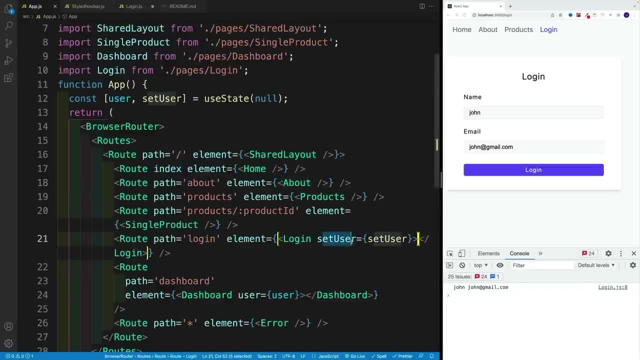 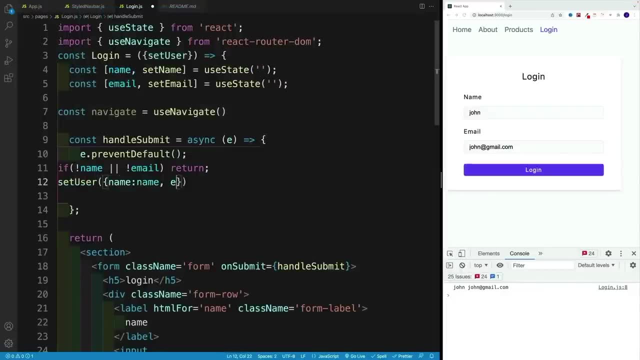 set user. again, this is coming from the app, Just like. so First we want to invoke it, we want to go with set user. Let's pass in: the name equals the name and email equals the email, If you want to shorten. 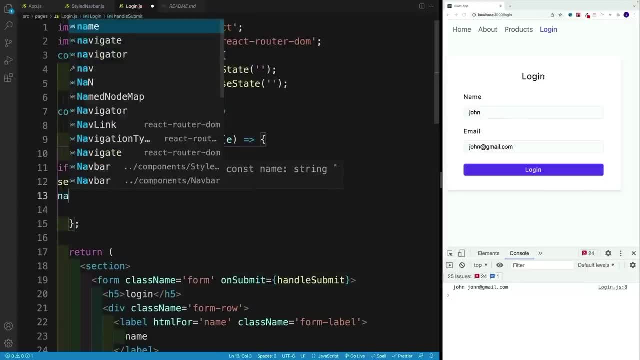 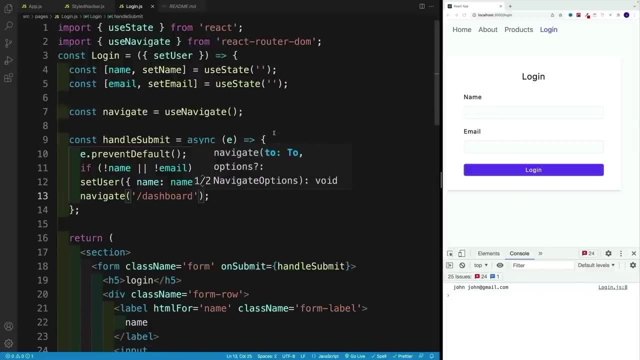 this up. of course, you can definitely do so, And then let's go with navigate And where we want to go. we want to go to forward slash and a dashboard. Let's save this one right now. Let's try to do that with only john. So if I just provide one value notice, can? 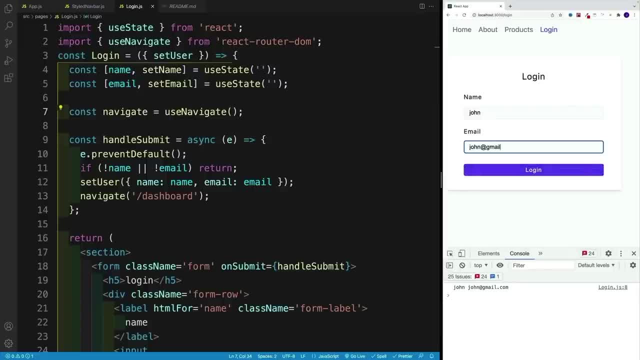 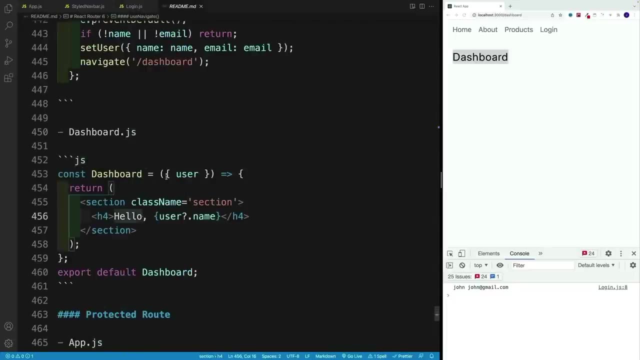 I do anything, Or if I go john and gmailcom, we'll notice that we'll. we'll see that. we'll nicely navigate to the dashboard one And in dashboard, I just want to display the name And the way we set it up. if we take a look at the dashboard, we just want to grab the. 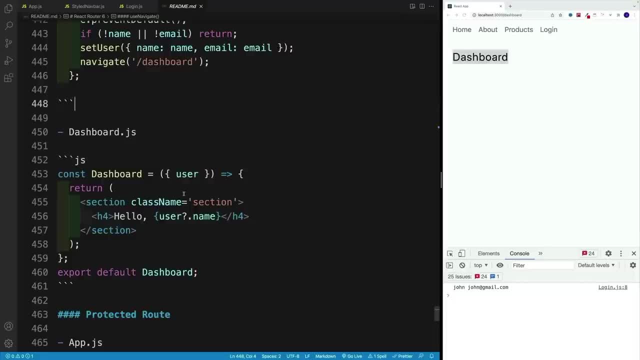 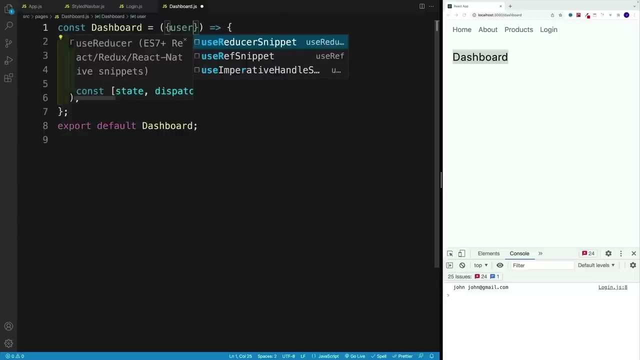 user, Since that is what we're passing in the address again. More specifically, I'll look for name. However, there's going to be optional training, since initially it's going to be no. So let me navigate right now to the dashboard one. Let me grab the user And 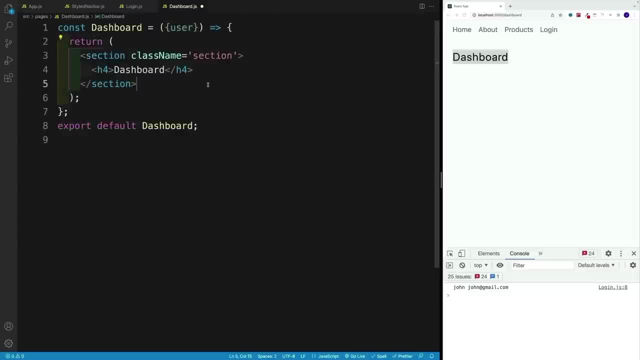 once we destructure it, where we have the heading for, instead I'll say hello And let's just access the username- like I said, optional training- And then let's go for name Once we save we have. Oh, john, if we'll navigate to a login and we'll go with Peter instead. 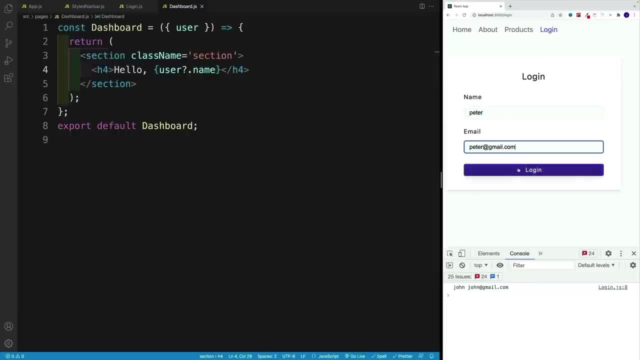 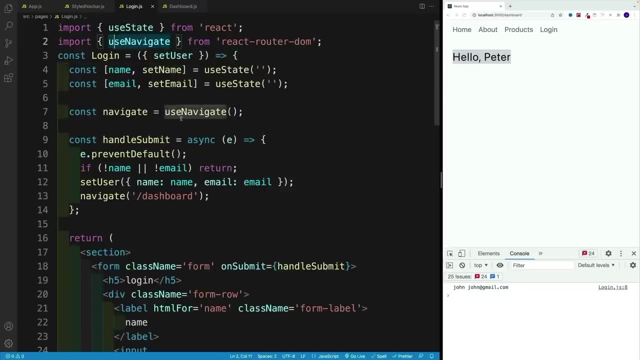 and Peter gmailcom. First, we'll programmatically navigate once we submit the form And then, using the use navigate, which we imported, then invoked it And we just pass in the path, the dashboard one, And in the dashboard page we actually display the name of the. 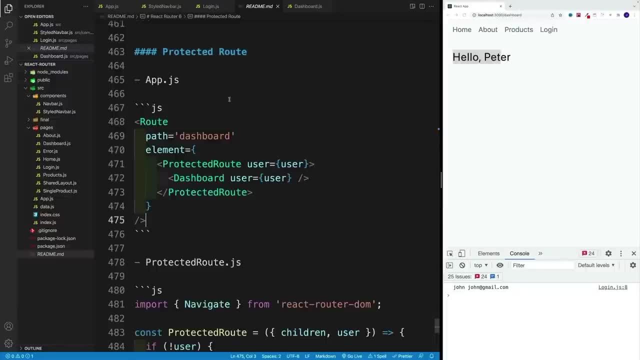 user, which in this case is Peter. All right, and now let's see how we can restrict access to certain routes, And first in the pages, we'll have to create that component. So let's say in this case it's going to be protected route And then in the app: Jess, you want. 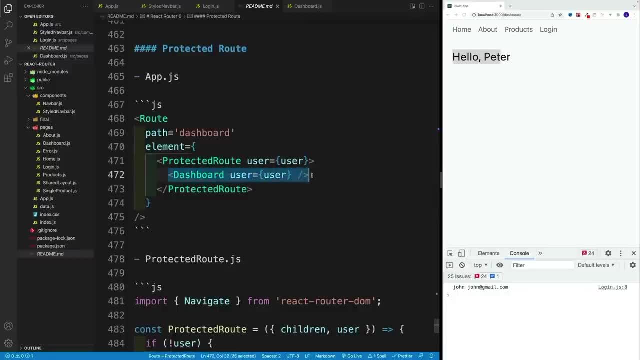 to wrap whatever page you want to restrict access to in that protected route. So yes, in the element you'll have to go with protected route and then whatever page you want to render, So automatically this page will be restricted. So let's start here. in the pages, 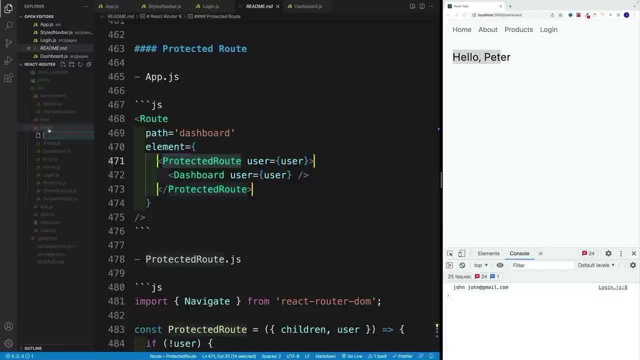 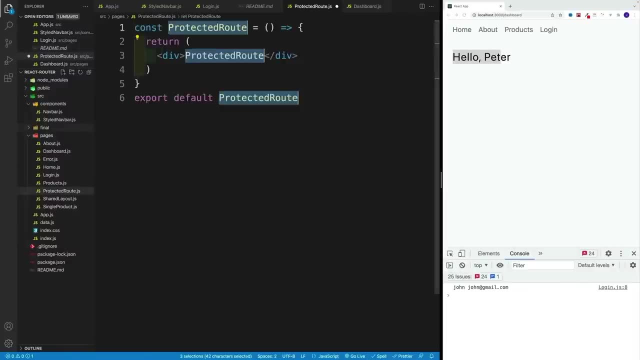 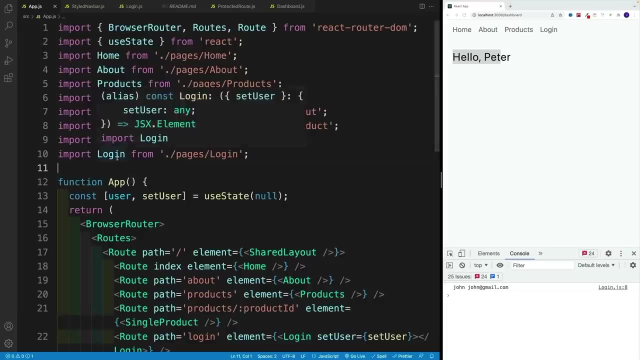 Let's set up New file. I'll call this protected route. For the time being, it doesn't really matter what we display here, since the logic is going to change anyway. And once we have the file ready to go, let's navigate back to app. Yes, we want to go with protected route, And since 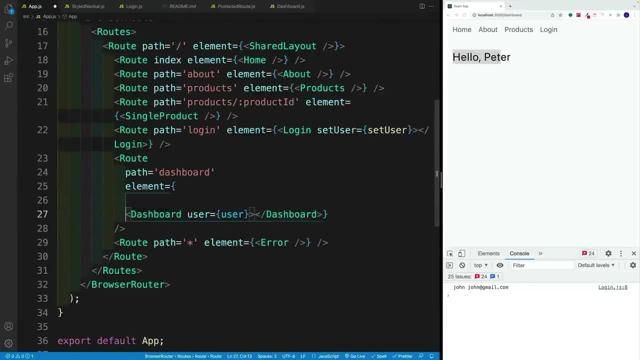 I want to restrict access to the dashboard. now. I want to wrap the dashboard with a protected route. I'll set it up as self closing. Let's go here with protected route And, like I said, normally will pass in the user using use context Or, in this case, since it's right away in. 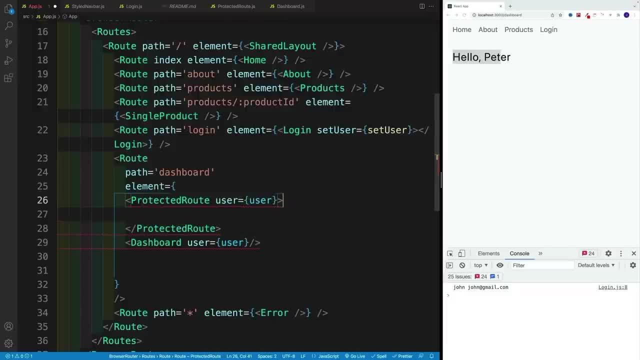 the app. Jess, I just go with user equals the user, since we'll need to check it, And then, if the user exists, only then we'll display the dashboard. So now notice, even though the URL says dashboard, we're displaying this protected route because now we're wrapping. 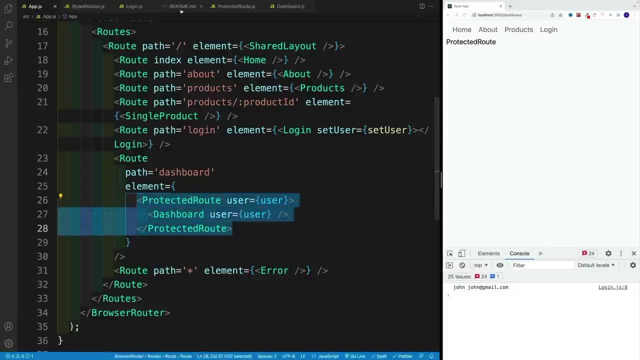 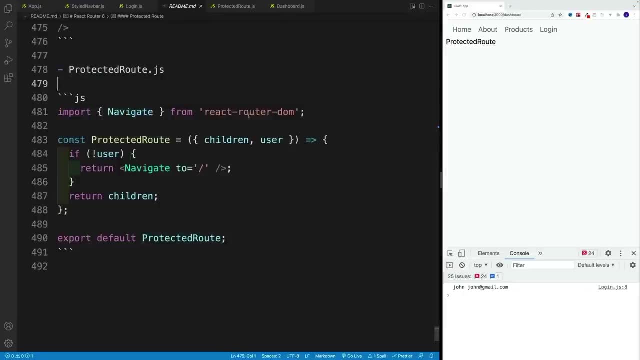 dashboard with protected route. So up next now let's set up the functionality where in the protected route we want to import navigate component from react router DOM And then we want to access two things. we want to access the children, So this is going. 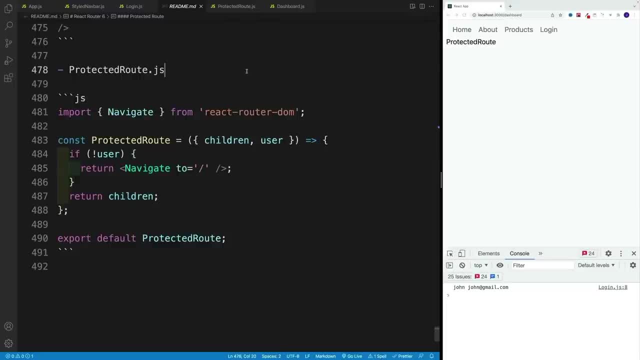 to be that dashboard page or whatever page we place in that protected route And also a user, And then we'll check. if the user doesn't exist, we want to use navigate component. We'll just say where we want to navigate. However, if everything is correct, we'll return. 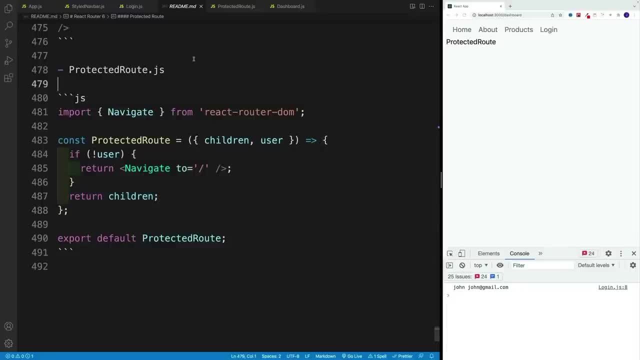 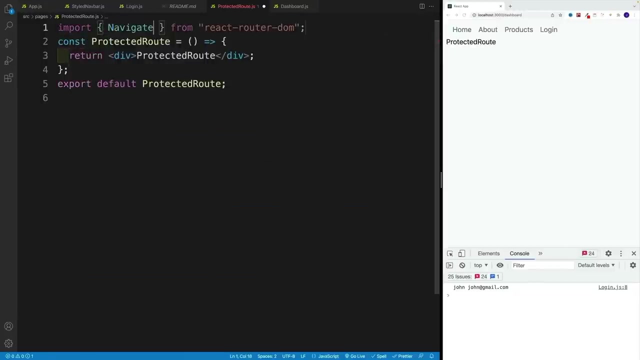 children in our case is going to be our dashboard. So let's go to protected route And first let's grab that navigate. So I'm going to go here with import, then navigate. So navigate component from react router DOM. then let's access both props, So children's prop, so 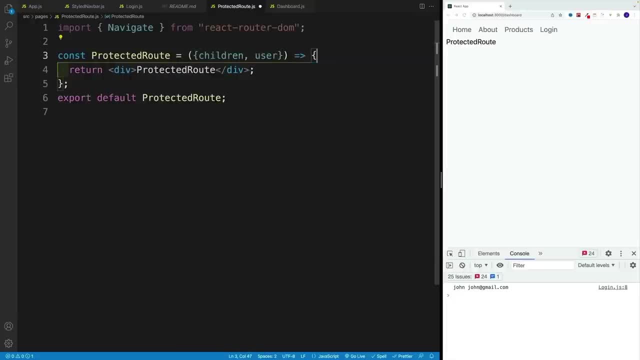 children and then also user. And let's set up that logic where if there is no user, then you want to go with return and navigate to. I'm just going to go to homepage. please keep in mind we can navigate wherever we want And then, if everything is correct, then we'll. 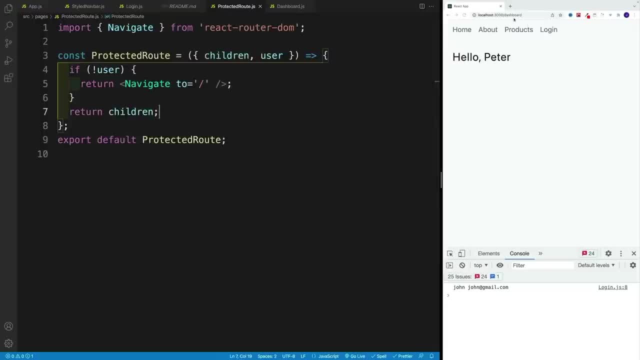 just return children. So, with this in place, what's going to happen? once we refresh, we'll have homepage. If, let's say, we try to somehow manually get to the dashboard, the access will be restricted. Notice how we navigate back, Why? Well, because there is no user. 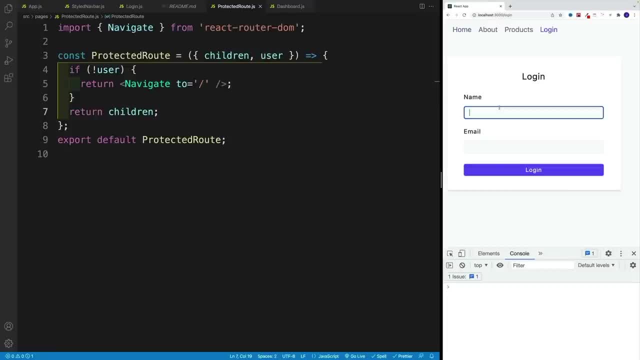 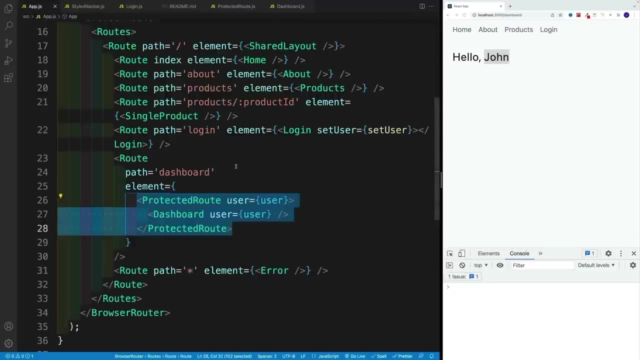 So only if we go to a login one, add that user- my case john john- at gmailcom, then we'll be successful and navigate to the dashboard and display. And again, I guess the biggest gotcha is the fact that in the app js, where you render the pages, you do need to wrap. 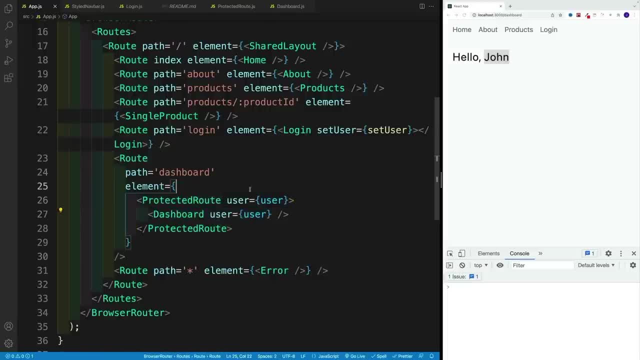 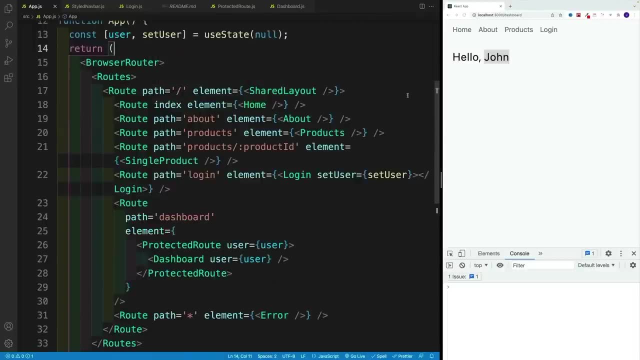 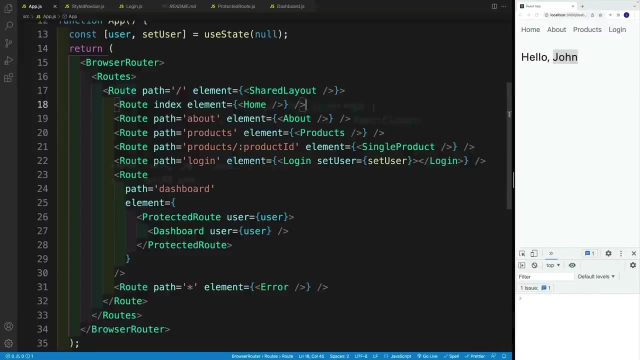 it. you need to wrap whichever page you want to restrict access to in the protected route component Beautiful, At the very end. I just want to set up the product and product ID As a nested route, And this is the case where, if you want to challenge yourself, you can. 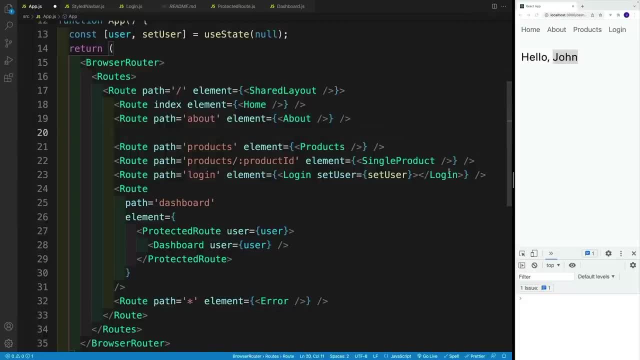 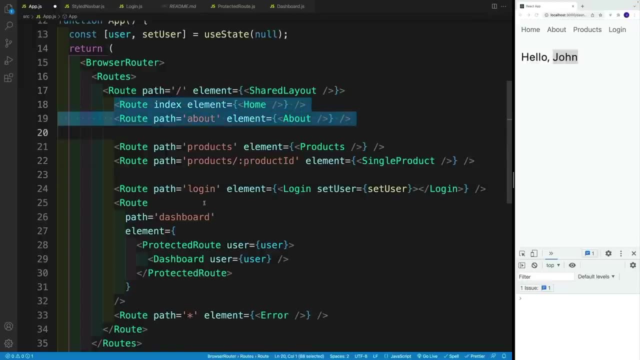 stop the video and try doing it yourself. So, basically, whatever we have right now here with a homepage where we nested rest of the route. I also want to do the same thing with the product where we want to place a product ID inside of the product we do want. 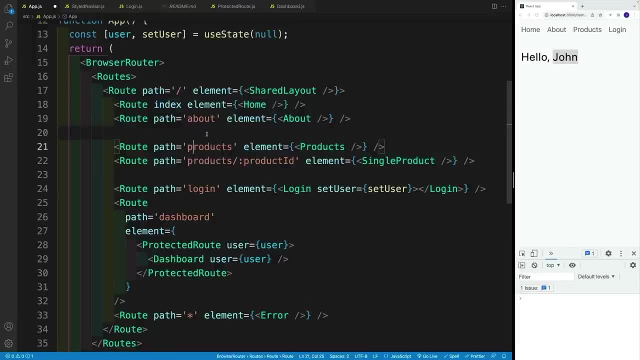 to set up the index one as well as some shared layouts. So again, if you want to try doing that for yourself, stop the video. try to solve this puzzle again. Basically, the setup is exactly the same. you'll probably want to use a different. 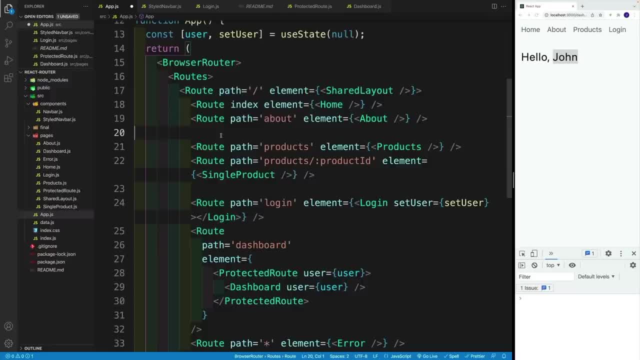 shared component. That's it. So let's start here by setting up that component. So I'm going to go here with shared product and layout. I know it's somewhat long name, but we'll deal with that. Then let's grab quickly the. 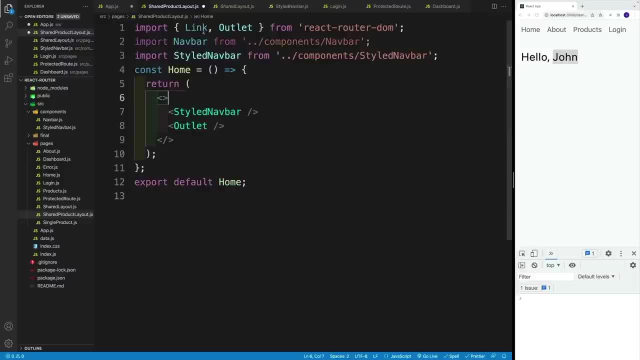 code over here, since I don't want to waste my time on imports and all that. So I have here a link. I don't think I'll need that. What I want is outlet. I won't need the nav bar, And as far as the shared layout, well, there's not really much that I want to add. 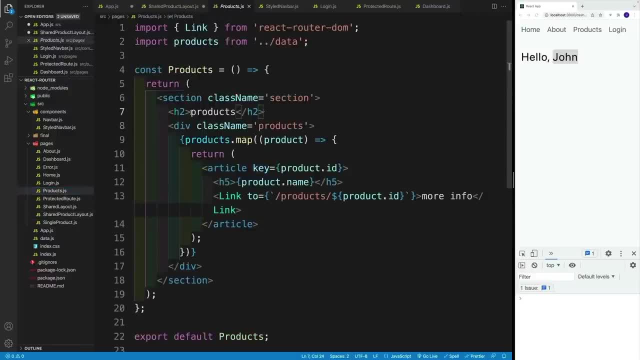 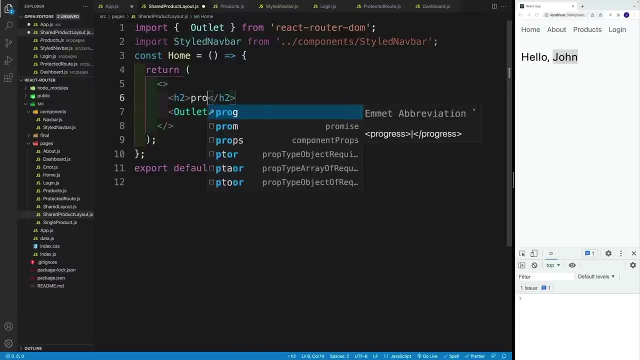 over here. I guess I'm just going to take a look at the product one. So in here I just have heading two. So let's do it this way: where we'll go with heading to go with products, we'll keep that one.